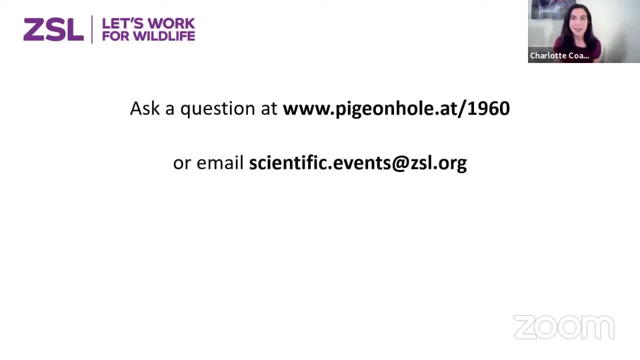 easier for us to see which are the most popular questions and try and ensure that we tackle those during the event. If you're having problems getting onto Pigeonhole, the other way you can ask our speakers questions during the event is by emailing, So please do send your questions to. 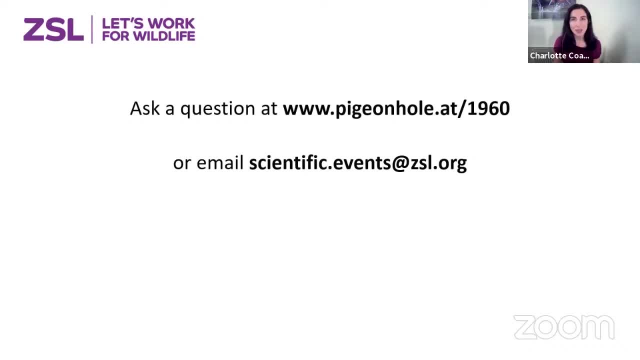 wwwpigeonholeat forward slash 1960.. That's scientificevents at zslorg. That's scientificevents at zslorg. The other thing I'd like to mention before we go any further is that we really welcome your feedback and thoughts at the end of the event, And so we have set up a SurveyMonkey online for this. 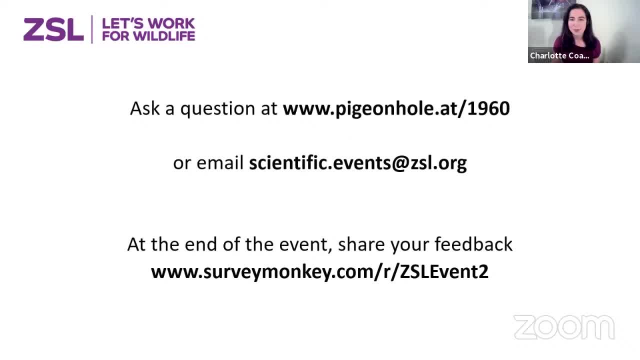 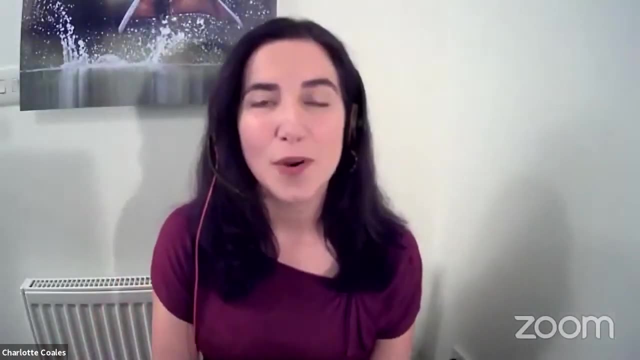 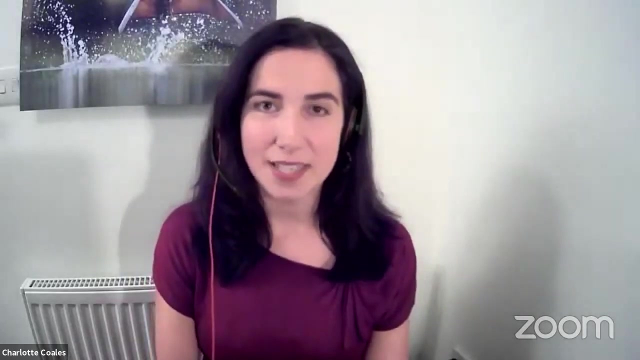 You can go to that survey by typing in wwwsurveymonkeycom. forward slash r, forward slash n, And you can find that link at the end of the event. So, as I mentioned, we're going to be hearing from four different researchers this evening And the first speaker tonight is Dr David Redding, who is 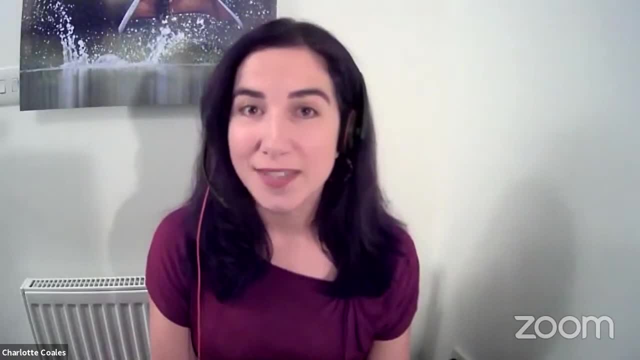 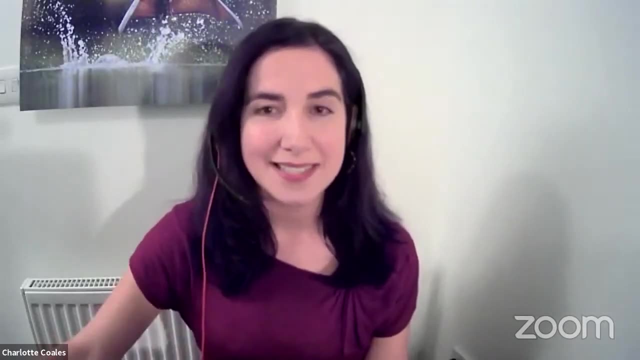 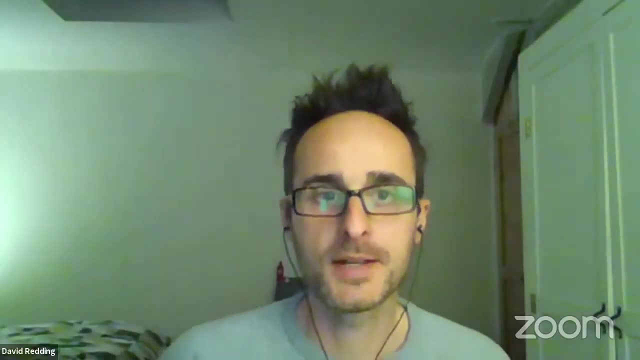 a research fellow at ZSL and also the convener of tonight's event. He's going to be discussing how habitat loss impacts human disease risk. So, Dave, thank you very much for joining us Over to you. Well, thanks very much for that introduction And thanks very much ZSL for hosting us. 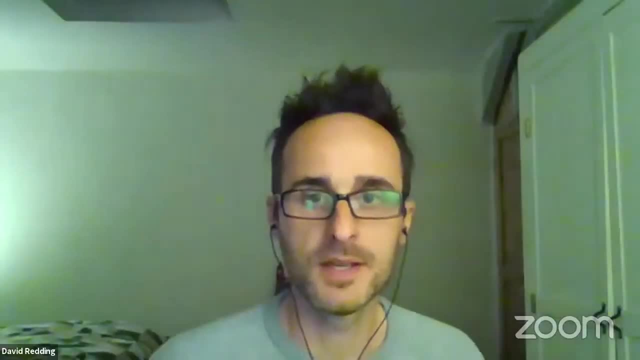 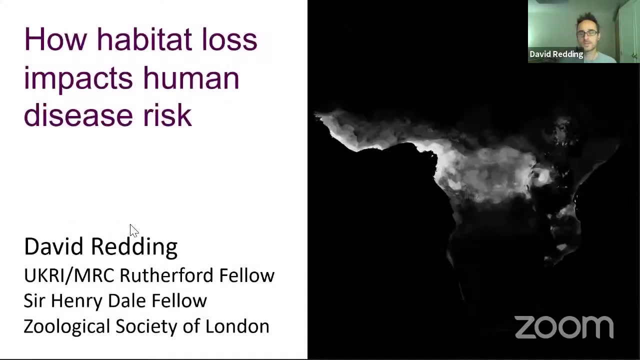 And also thanks to our great set of speakers that agreed to join, And so what I want to do is talk about. I'm just going to bring up my presentation, So what I want to do is give some of the background to some of the things that our speakers are going. 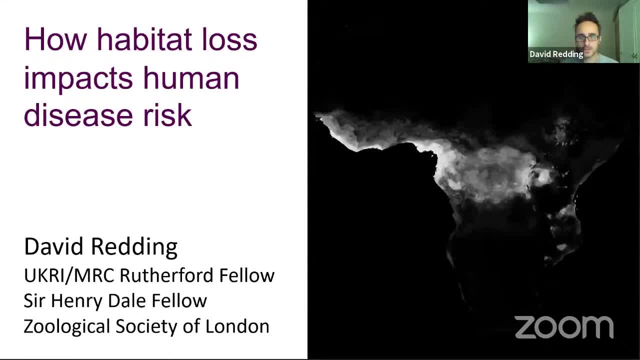 to be talking about next. So to give a sort of background to some of the topics that they're likely to be discussing, And so broadly, this meeting is focusing on the idea of habitat loss and how that might impact us in terms of our health. 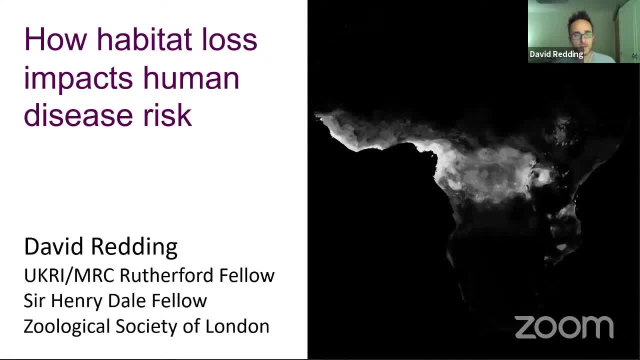 And so this is obviously a topic that is of high current interest, And so it's something, it's an area That I personally have been working on for about sort of 10 years, And so I think it's really, it's really great that that people are so interested and wanting to engage with it. 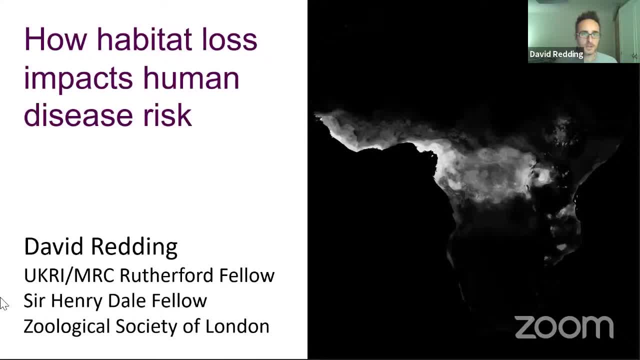 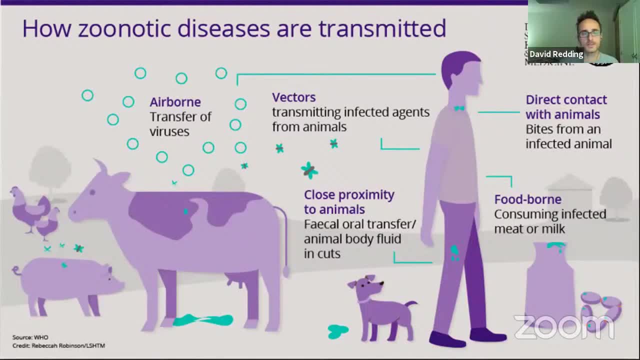 So what so that? so what I'm going to be focusing on mostly are zoonotic diseases. So the recent events have made it much more straightforward to for me to give talks a lot of the time, Because people understand the idea that diseases can be caught from animals. 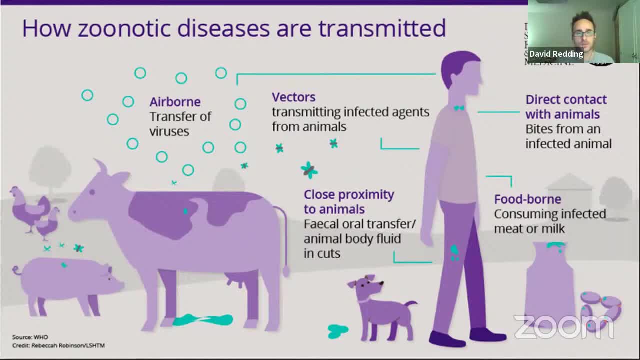 And there's a variety of different ways that that can occur. So it can be through sort of direct contact, where people go and say catch an animal for food, or through animals or livestock, So the husbandry processes, and also through pets and do things like biting insects. 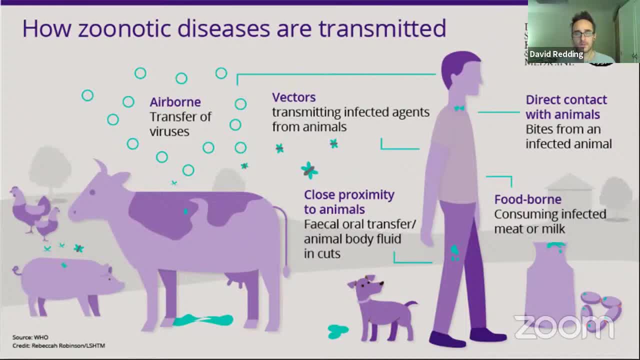 That carry diseases from one animal to two people. So this is a process that isn't sort of rare. It's something that goes on throughout throughout the world. throughout all levels of biodiversity, Organisms are sharing these sort of pathogens. or sometimes they're not pathogens, some of the microorganisms just swapping between species and individuals within a species. 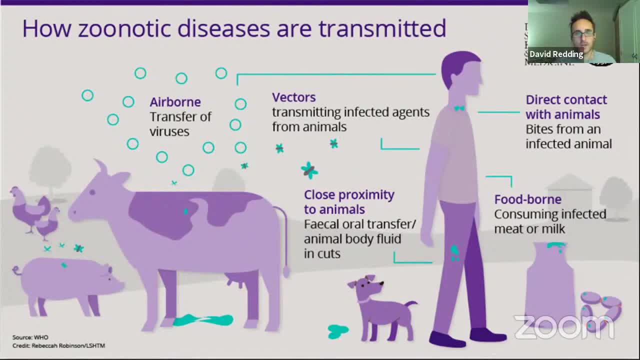 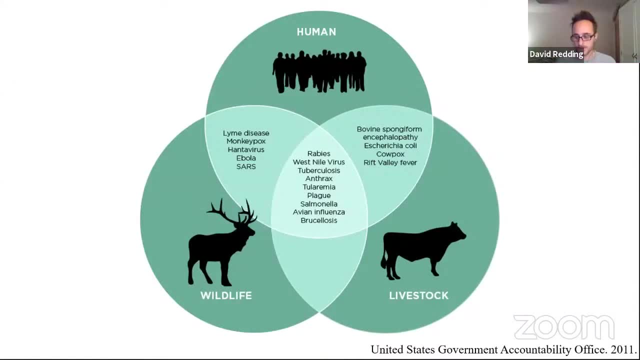 So this is happening all the time, And so This is only a really big problem when those, those microorganisms, the viruses and bacteria and sort of single cell parasites that are transferred between species and from species to people when they cause disease. And so here are some examples of diseases that have either a wildlife source or a livestock source, or both. 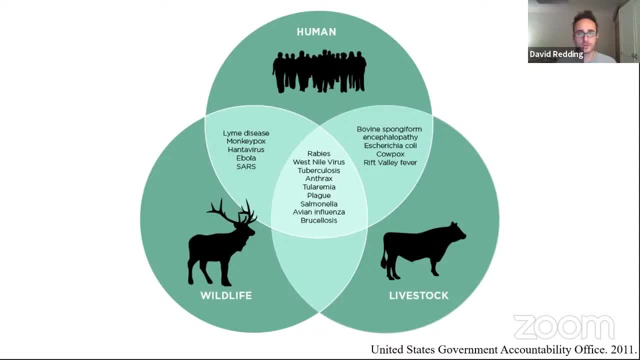 We're both domesticated animals And wild animals are involved, So we've got things like Lyme disease and Ebola, which are principally caught by people from wildlife, And then we've got things like E coli Rift Valley fever in West Africa, East Africa. 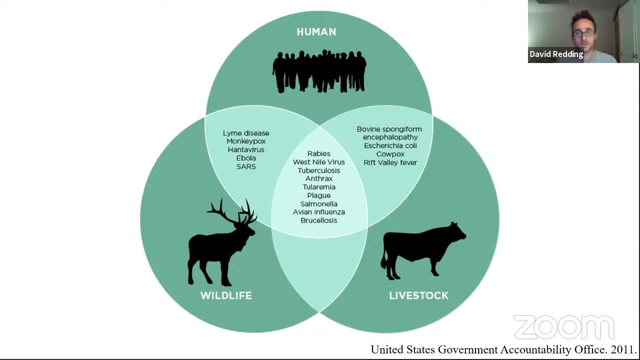 And And then we've got ones where they're either both livestock and wildlife involved, so things like rabies and anthrax and plague. So there's a. there's a huge variety of Zoonotic diseases. in fact, most diseases are most ones that the vast majority of diseases that we know. 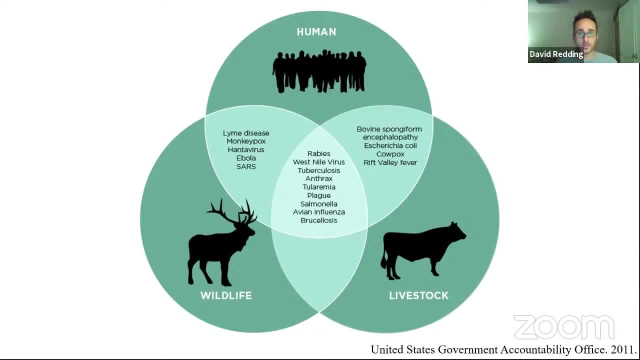 Excuse me- are animal born, so they come from animals, and nearly all human diseases originally had an animal origin. So Why are we talking about habitat change? Well, if most diseases have this wildlife origin- and a lot of diseases Have a wildlife component- 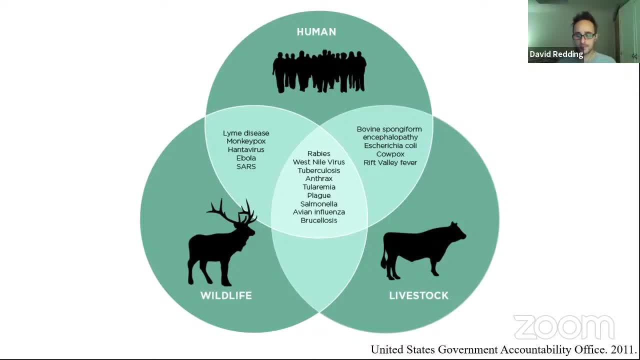 We need to think about what's happening to wildlife and that, and by understanding that, we're going to understand about how, how, what our future health is going to look like. And so probably the most immediate sort of systemic, Sort of global threat to wildlife is- is land use change. 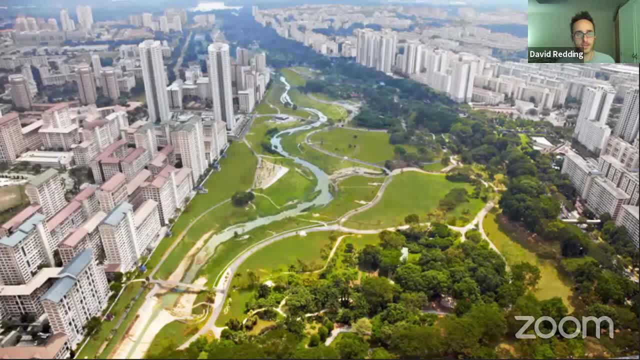 And that is the process by which people are taking the world and taking different sort of natural Habitats and things like rainforests and deserts and grasslands and turning them into habitats that suit our needs, So ones where We get. we get things that we need, such as just food or shelter or or recreation thing. 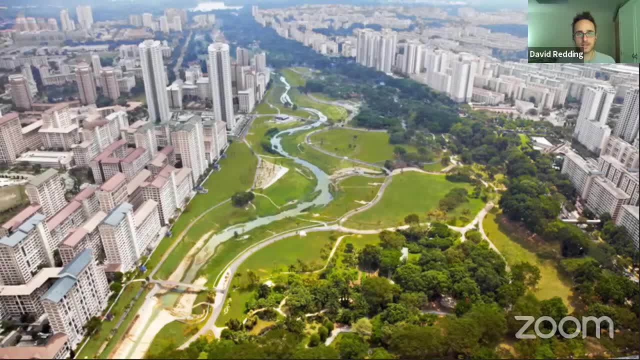 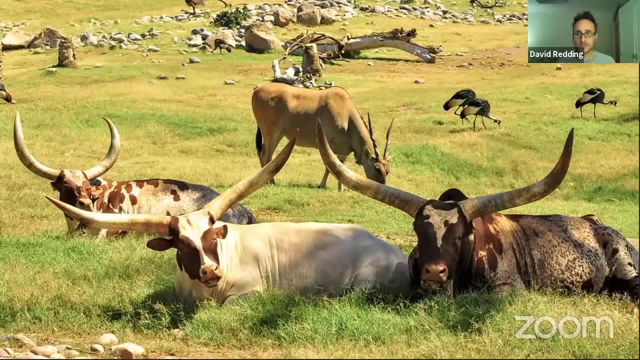 We're converting it into into, into types of landscapes that are useful for us. So so one example is is urbanization, So increasing amounts of habitat where we're living, We're actually We're actively living on, And then there's also habitats that we're converting or using for grazing. 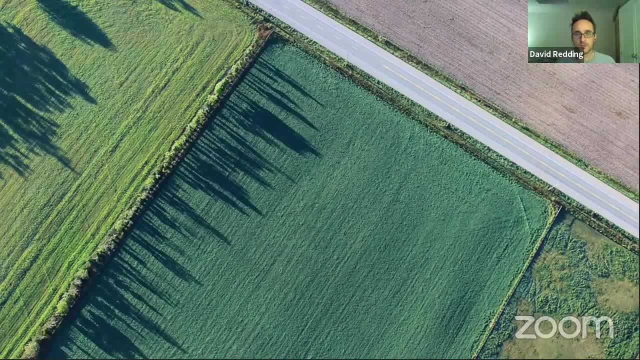 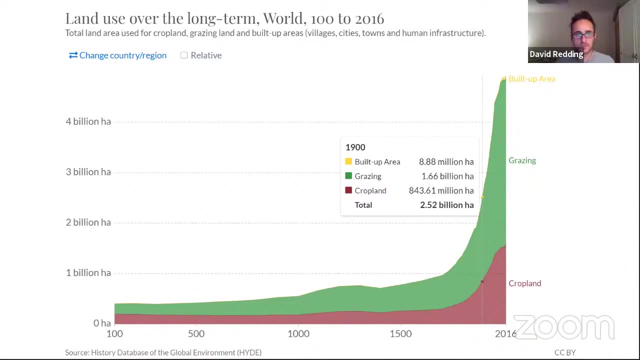 And also just for for vegetable food, a vegetable food production, So that's sort of cropland areas. And Well, This has happened. Obviously, the world, the world's been changing for a long time Recently, And so here we're talking from nineteen hundred. 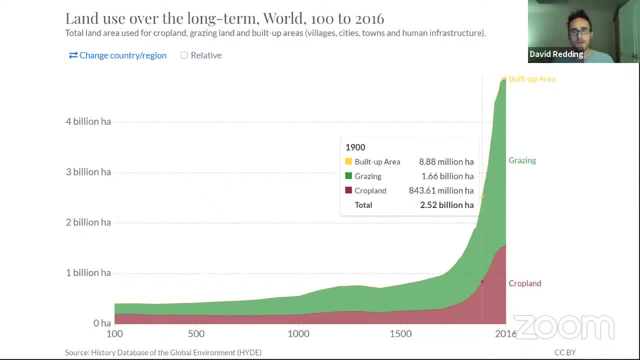 We've got approximately a doubling of of the total area of the world that is covered in in both cropland and grazed areas and in built up areas, And so we're seeing this increasing imprint of, of, of human, of humans, on the earth. 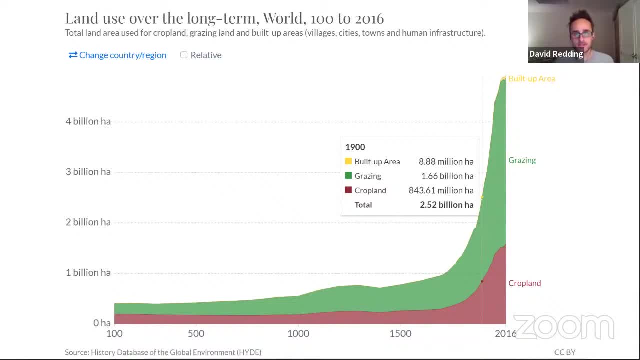 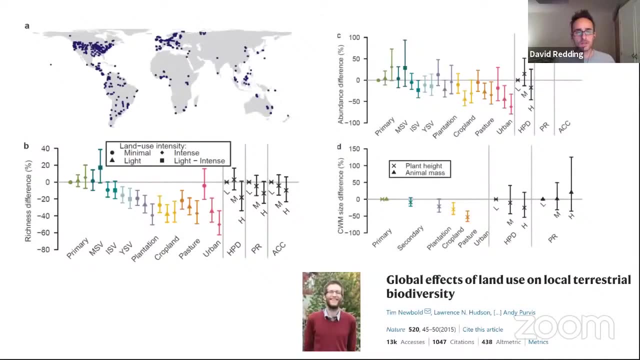 So more and more of the earth is being converted into these, these, these particular types of Landscapes. So why does this matter? Well, here's a paper by Tim Newbold and colleagues from 2015.. And it seems very complicated when you first look at it. 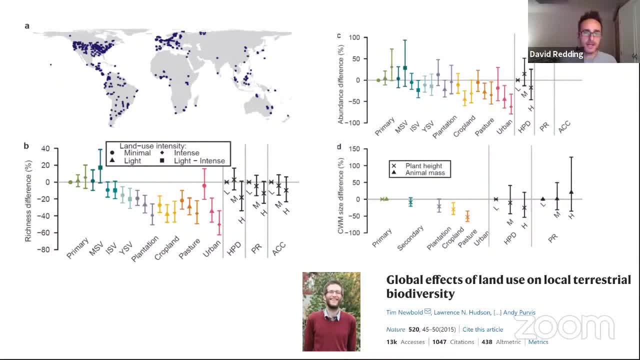 But if we just start in panel A, that's where all of the sites were, And I'll come back to why that's important in a minute. In panel B, we look on the left hand side of your screen. You'll see. 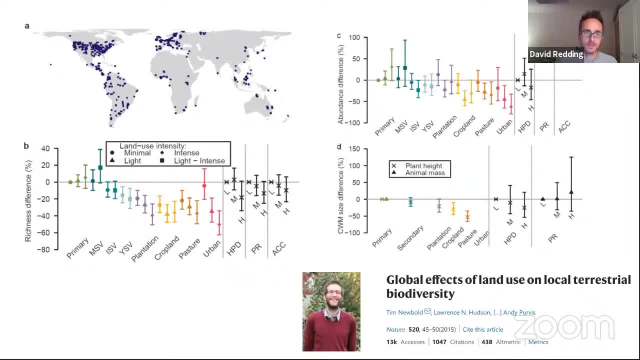 A dot that's underneath, That's above the word primary, And all of these dots with the, with the lines through them, represent different land uses And as you go from left to right, what we're doing is we're moving from more natural through to much more human dominated land uses. 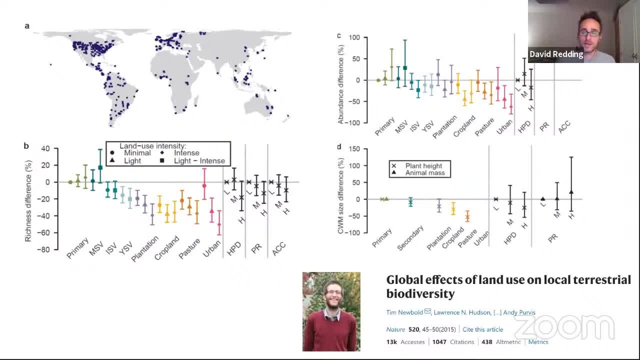 And so this, this graph, is showing how how species richness on average is changing, And so what we're seeing is that across all these different sites That you see in the map above- So this is across the whole world- We're seeing a decrease in the number of species. 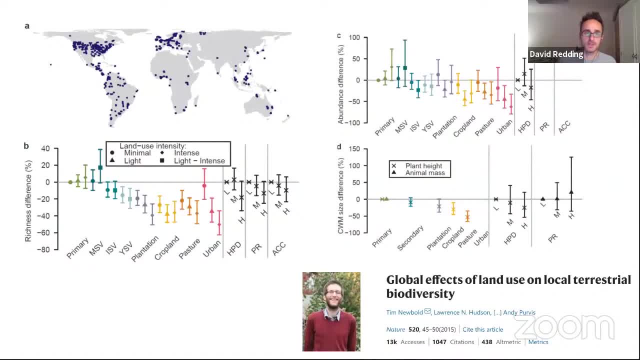 So for any any one of these sites, if you converted it from a more natural to a more human dominated site, what we see is that, in general, there's a decrease in the number of species, And so if we look in panel C and the top right hand side, what we're looking at there is the total number of individuals. 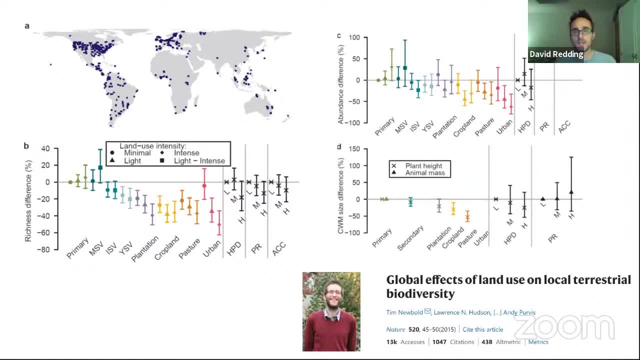 So what we see is a reduction in the total number of species And this is a reduction in the total number of individual animals in these different land uses. So the general response of biodiversity to these large, ongoing changes to the way people are using land is that we're seeing a reduction in the number of species and individuals. 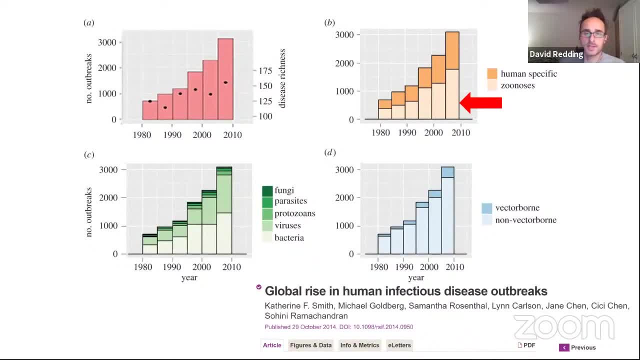 So what? what about zoonotic diseases? So this is a paper from 2014 by Catherine Smith and colleagues, And, and what they've done is tried to look at how the number of human disease outbreaks is changing over time. And if we look at the big red arrow that I put in, what we're looking at there is the total number of known zoonotic diseases. 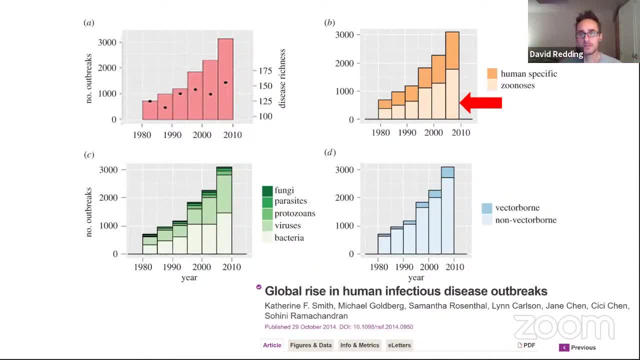 And so what we're seeing actually is an increase. So if wildlife is a key component and we're seeing a decline Generally, why are we then seeing an increase in zoonotic diseases? So this could be to do with we're just better at detecting them. 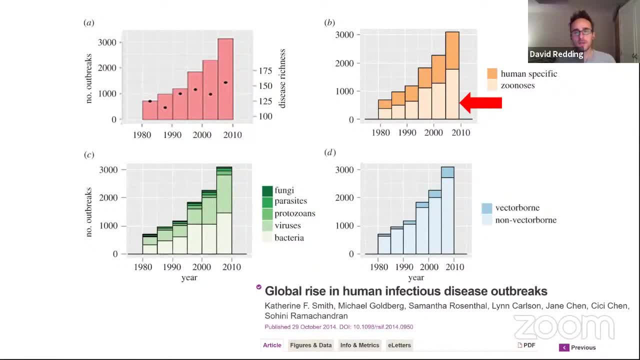 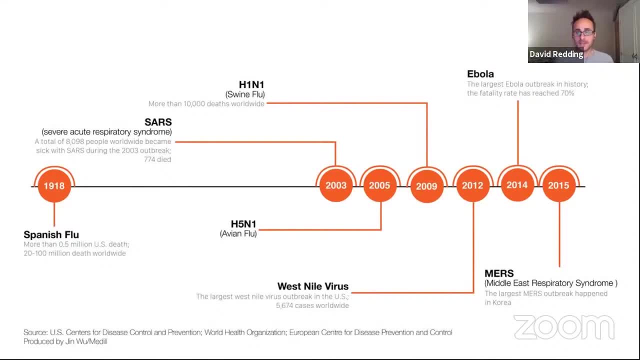 So that might be one reason. But if we think about that, if we look at very large outbreaks which are generally well detected- you know, people very rarely miss Huge global pandemic, as we know Well- these, these large outbreak events seem to be increasing in frequency. 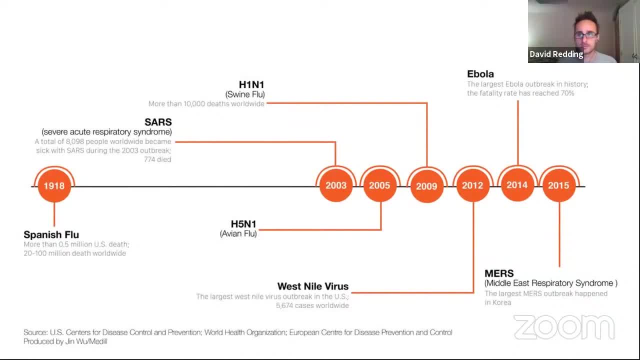 So not only do we have this idea that maybe outbreaks of all sizes are increasing, but there seems to be an apparent increase in the frequency of larger outbreaks, And this obviously doesn't contain the COVID-19.. So to try and work out why that might be happening, 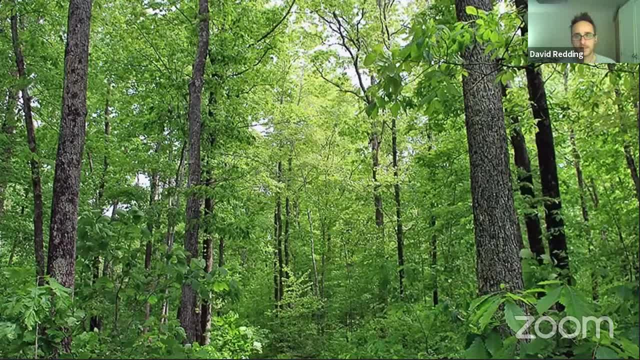 I'm going to use a couple of different case studies, So I want everyone- some people might be there already, but- to transport themselves to northeastern, the United States, and into the deciduous forest there. And what we have in these forests is we have groups, a community of mammals. 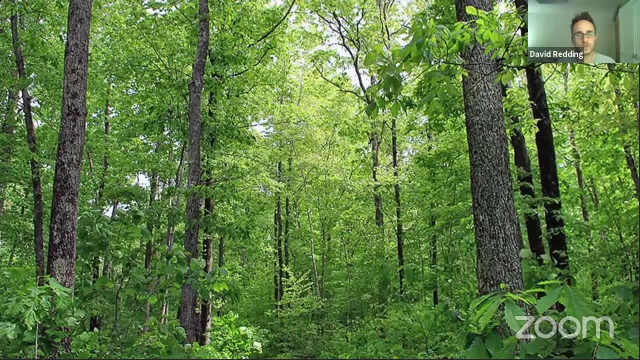 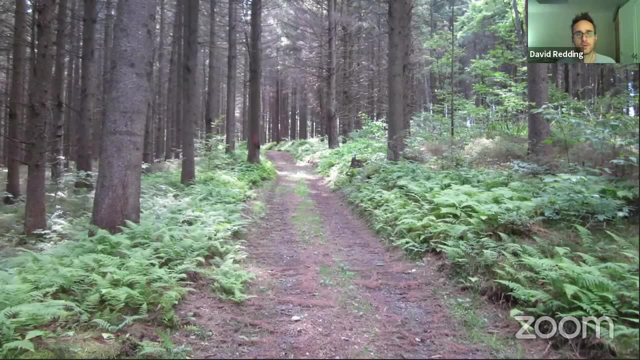 And so the mammals in those in this community exists, as we can see with some of Tim's points, As we can see with some of Tim Newbold's work, in this kind of very intact system is going to look quite different to a more degraded version of that system where it's being used as either a plantation or for sort of human uses. 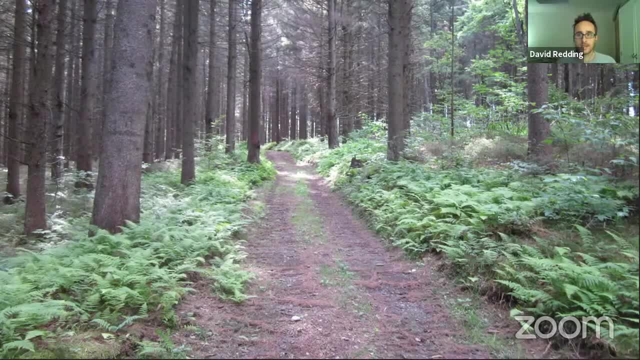 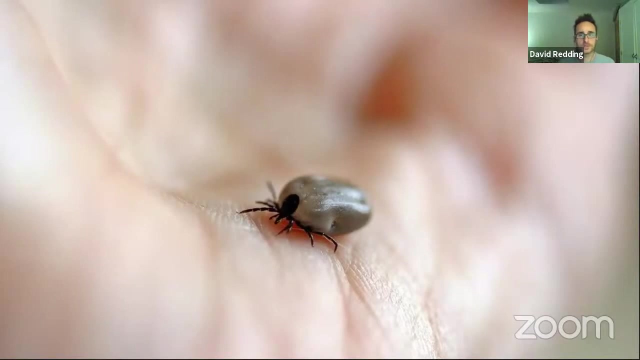 And so what we're seeing here is that, in a degraded landscape, we're going to see, in general, A loss of things like large bodied animals that need a lot of space and and particular animal species that are very intolerant of people, And so one of the critters that you have in this woodland system are ticks. 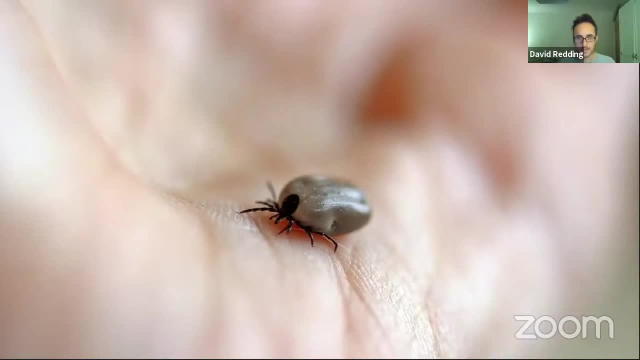 Ticks spend their time, you know, hanging around on vegetation and waiting for A mammal to walk past and will drop on them and then start feeding, And so some animals are much better at getting rid of these ticks, are much better at not having them. 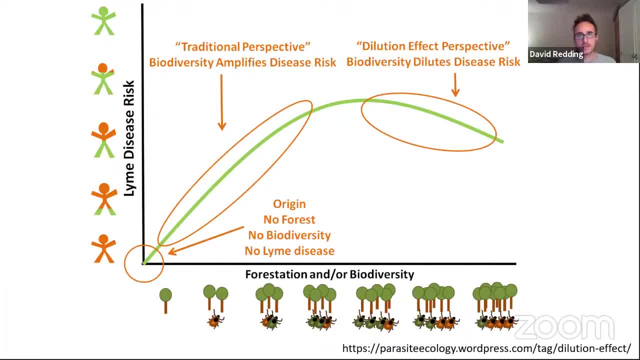 So What this brings us to is this idea called dilution effect. So in the bottom of the graph here we've got, we've got Forest Forest cover. So on the right hand side we've got a completely intact forest. 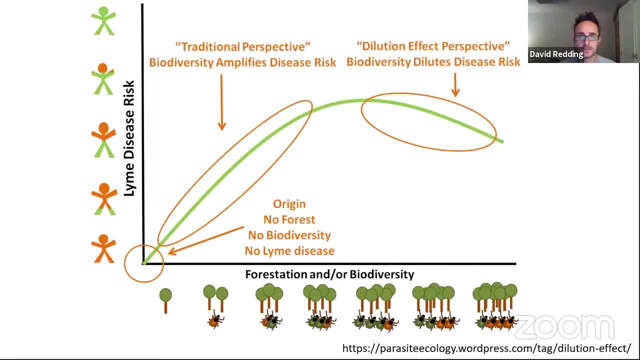 And on the left hand side we've got almost completely depleted forest. And if we just concentrate on the right hand side, what we're seeing is that the dilution effect is is one where it says: in very biodiverse forested areas, What we have are animals of all different competence at carrying. 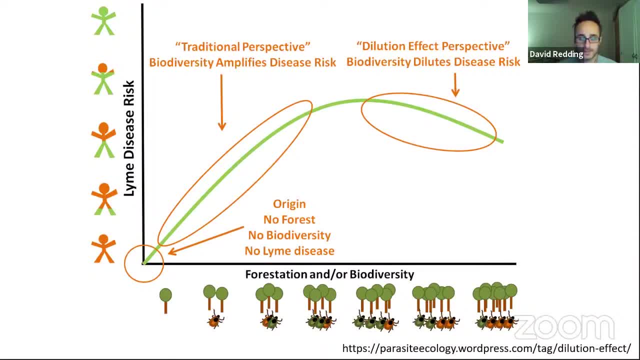 Ticks and therefore giving Lyme disease to people. So the Lyme disease is a bacteria that exists inside the ticks And that when, when the tick bites either a person or an animal, it can then spread into the body and then reproduce, And then next time it gets bitten it then gets transported. 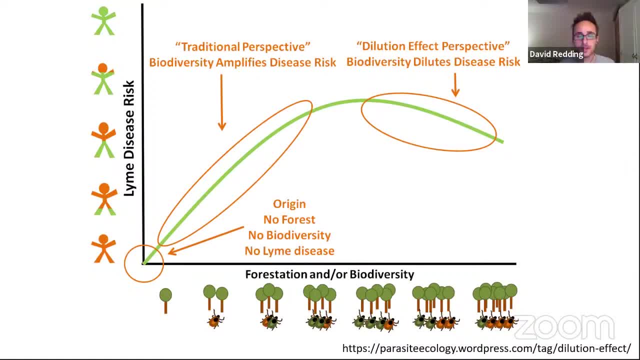 Excuse me. So The idea is: in this very biodiverse areas you've got species that have very mixed tolerances. As you move to this more medium habitat, what we end up with is actually we filter down to species that actually are just very good at having ticks and passing them on. 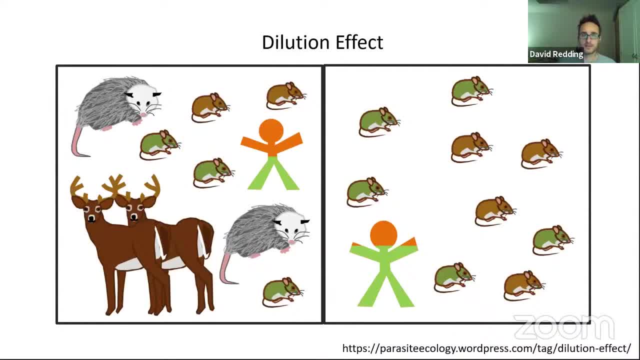 And so what we see here is, in the left hand side, a very biodiverse area. It has possums, it has deer and it has mice. Mice are very good at passing on the ticks and carrying ticks that have disease, And here it's diluted. 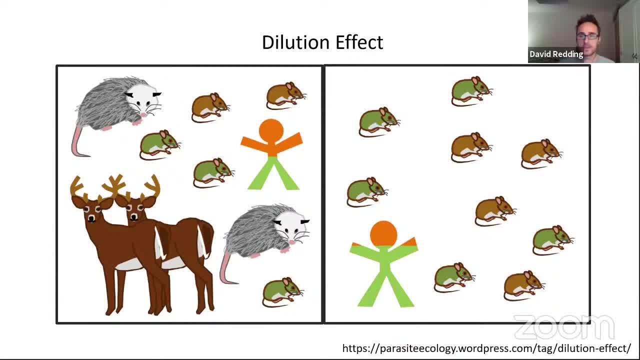 If you go walk around, you're likely to bump into a deer or possum. On the other side, you're mainly going to meet mice. So there's this idea that actually the intact habitats are actually buffering your contact with disease Caring species. 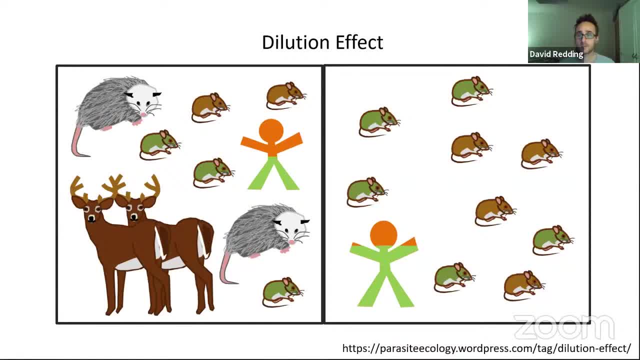 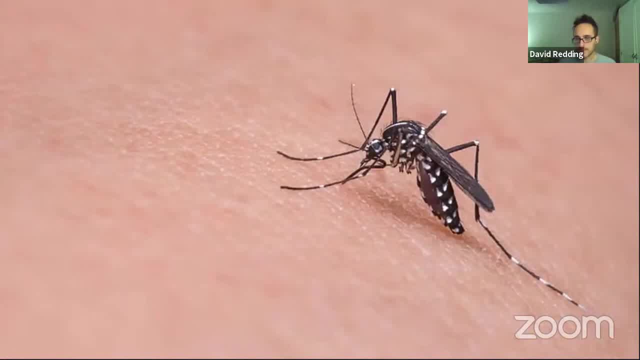 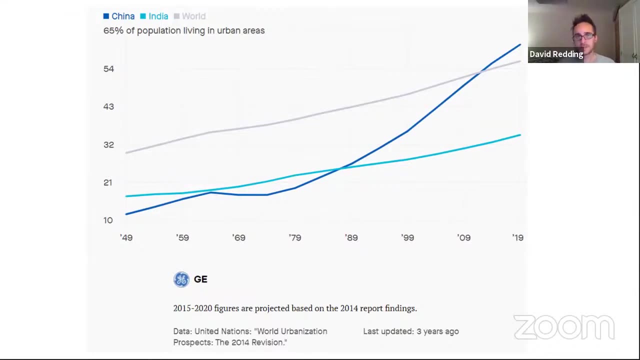 And that's by reducing intact habitats. That's why you're seeing an increase zoonotic outbreaks. So my next example is sort of moving to Southeast Asia and looking at the tiger mosquito And so What? one of the things that we see in Southeast Asia is a huge increase in in urban areas and in urbanization. 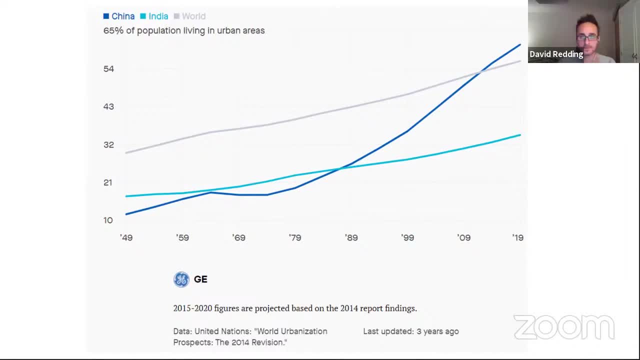 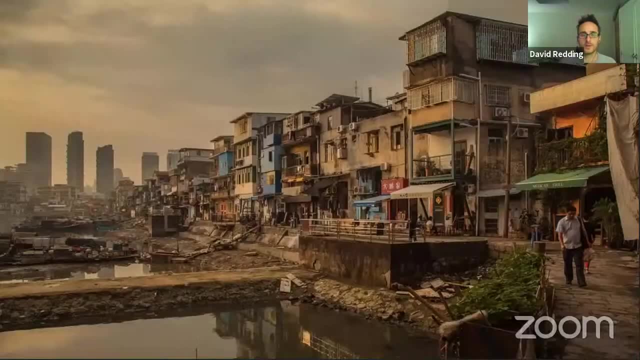 And here we've got China increasing very rapidly, with India keeping pace with the rest of the world, But we're seeing an increase in urbanization, So we end up seeing natural habitats converted into more urban habitats, And one of the things that the tiger mosquito is very good at is existing in just these types of habitats. 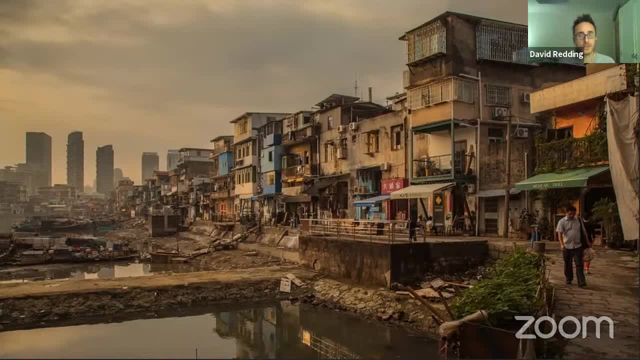 Whereas some mosquito species need forests or they like to live in particular, plants and rivers And rainforests, These mosquitoes, which carry the dengue virus, are very happy to live in these kind of conditions. So the increasing urbanization is what we're doing, is we're increasing the suitable habitat for the tiger mosquito. 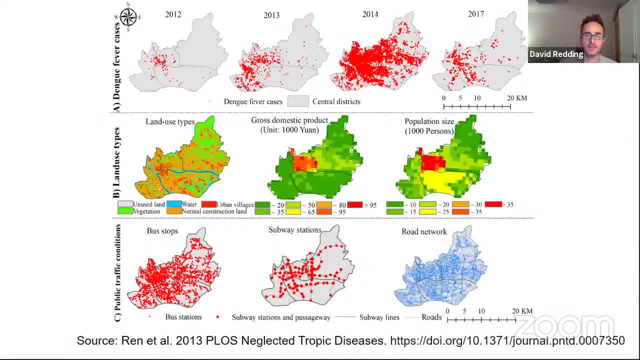 And then that what we're seeing then. for instance, here is a paper looking in a particular province in China And what this is showing. in the central area It's in red. We see urban areas and highly populated areas. What we see is where you have urban and highly populated areas. 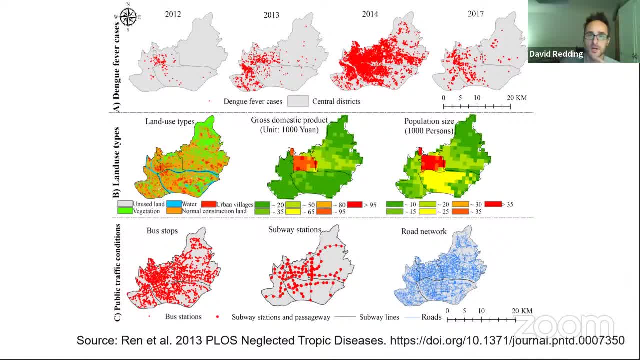 We have, above in the top row, large numbers of dengue fever cases, And this mosquito is so capable of living with people that we see that they can also start using transport systems. Any pocket of water that's anywhere along a road Can be can be used. 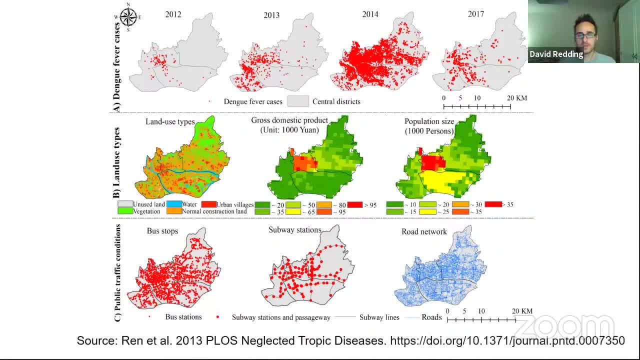 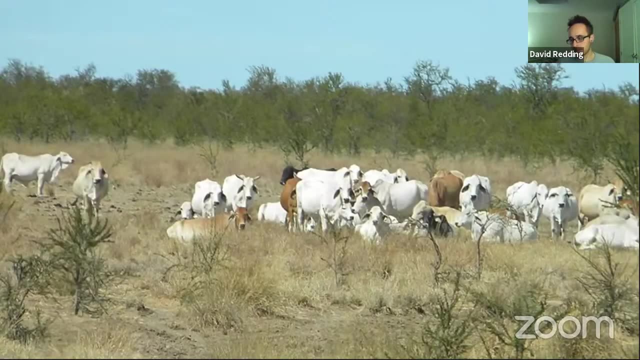 And so this, this kind of urban loving species that carry diseases and this massive increase- urbanization That's- that's another, maybe another reason why we're seeing increases in in zoonotic disease outbreaks And so kind of. one of the last things I want to talk about is is kind of agricultural areas. 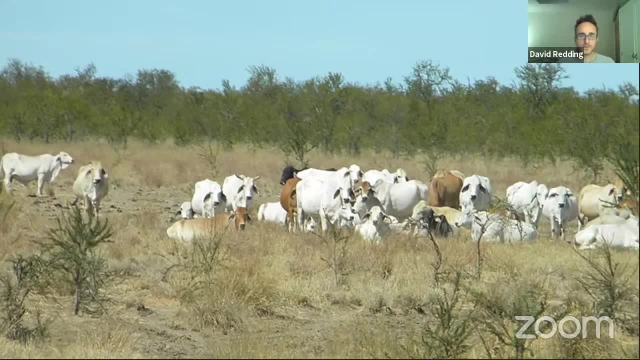 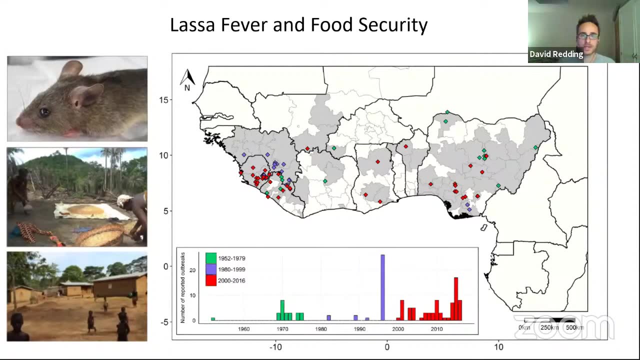 And, for instance, this is an area for the That's being used for grazing and Lassa fever, which is a disease that I've personally worked on, And so that that's the dots that we can see on the map of where we have had lesser outbreaks. 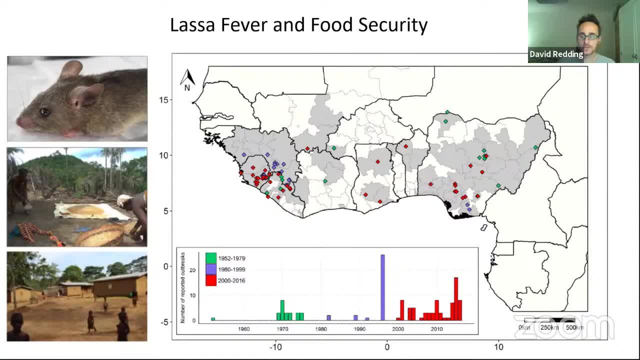 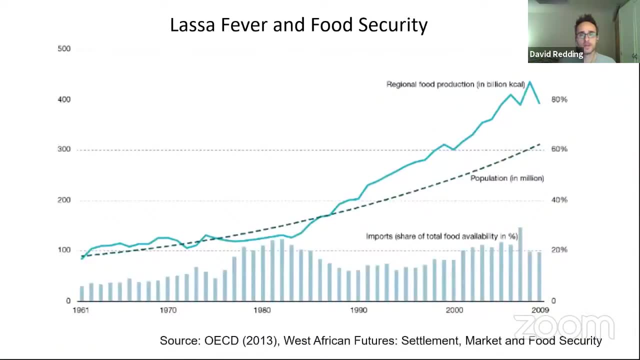 On the left hand side is the rodent that passes this disease on to people, And also on the left hand side we can see the kind of landscapes, these kind of agricultural, rural, village landscapes where master miss does very, very well. And so in West Africa we're seeing a huge increase in population in the dotted line. 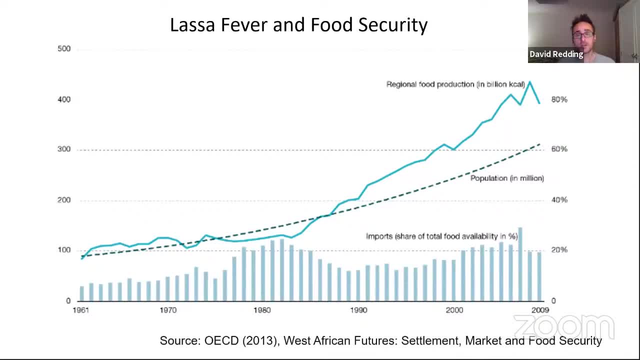 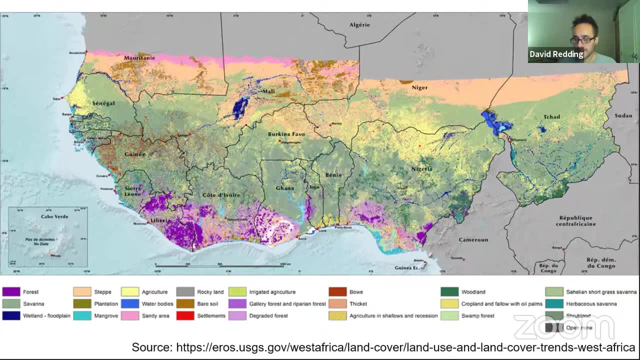 And then in the solid blue line, we're seeing a concomitant kind of increase in food production. And so as we try to meet that need, the food need of that larger population, this map goes increasingly yellow over time. So from 1975, 2000,, 2013,, we see this increase in yellow and yellow. 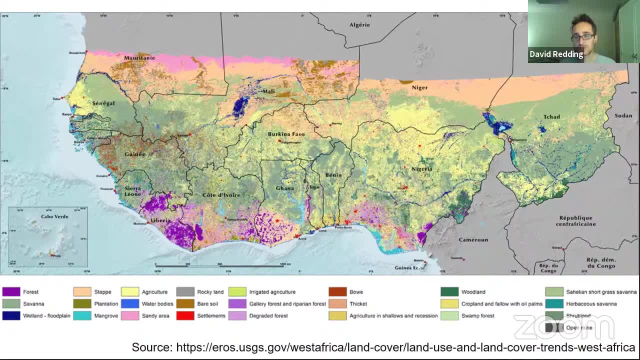 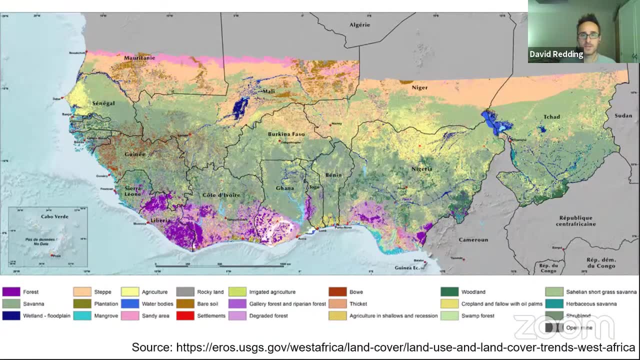 It's cropland And what we're seeing is this huge conversion to cropland area And, as we've said before, must miss that analysis which carries Lassa fever. It does very, very well in cropland areas. As soon as you have some cropland, they will move in. 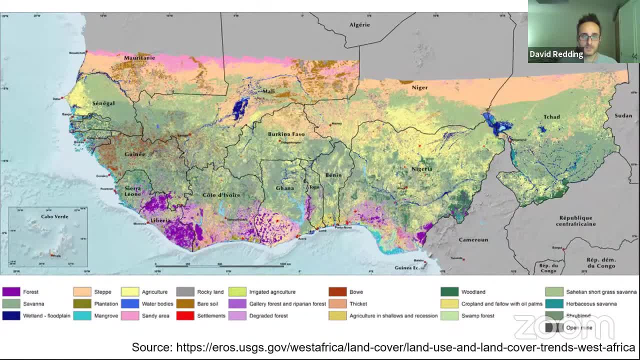 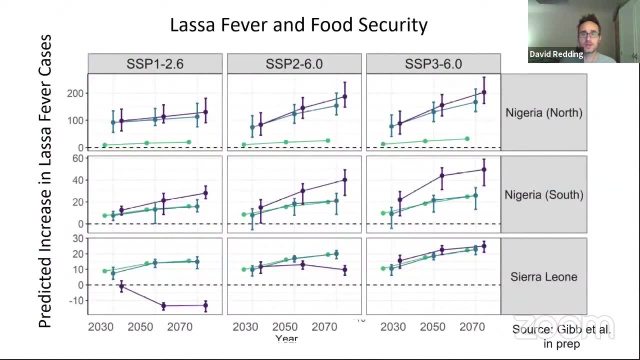 And you're then going to see, We're going to be boosting the amount of food we have, We can increase food security in the region to feed those people, But at the same time, what we see here is- And these columns are different- potential future scenarios of of land use change. 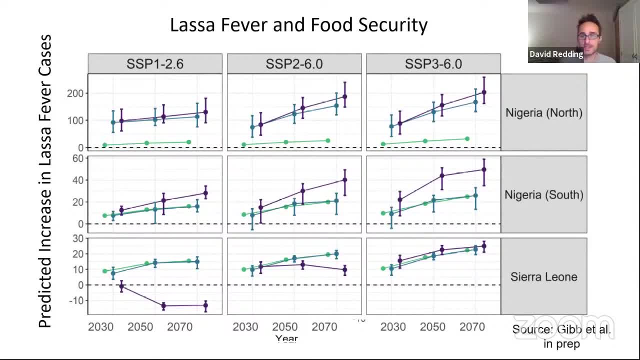 What we're seeing is an increase in Lassa predicted numbers of Lassa fever cases. So this is a paper that Rory, who will be speaking later, is working on, And so that the cost of this increased food security is increasing numbers of disease cases. 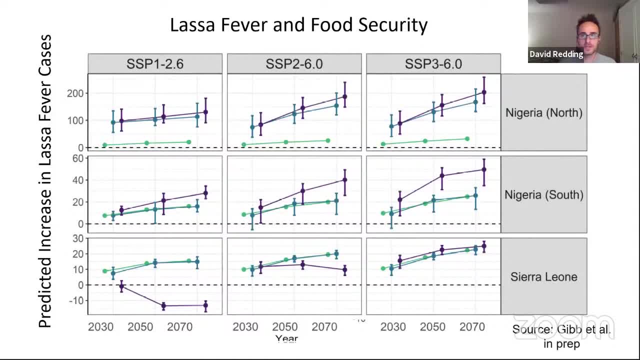 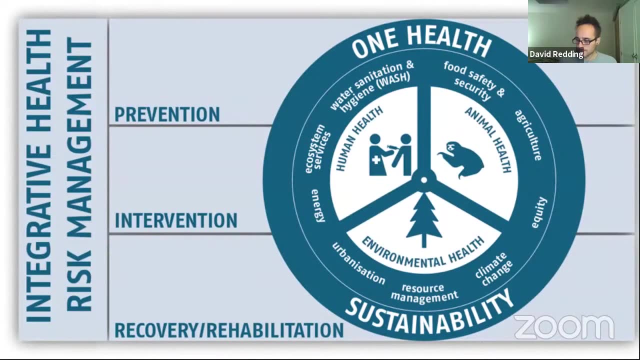 So there's these trade offs, these really important trade offs between Health and sort of other really important ways that the land can meet our needs, But it's a question of trying to think carefully about how these things might interact. And so What's the future? 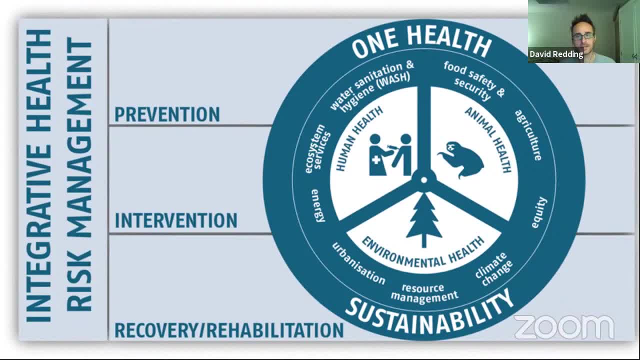 You know, I've used a couple of case studies to think about why we are potentially seeing some of these kind of increasing numbers of of outbreaks. Well, one thing we can do is to start thinking More holistically, So thinking about the kind of food security but also thinking about the sort of biodiversity angle. 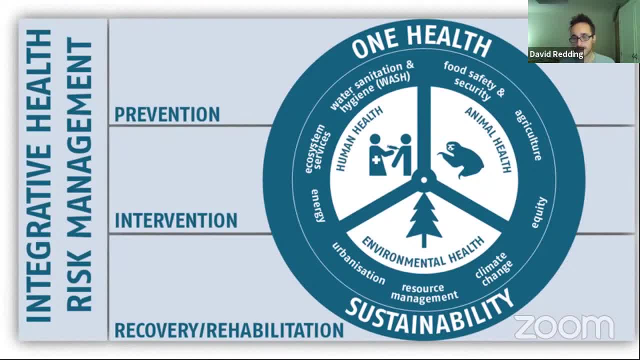 So there's this idea of kind of one health or planetary health. which are these ideas that we can actually Think about all of these things together and actually by promoting them all, We can, actually we can actually find these kind of win win situations. 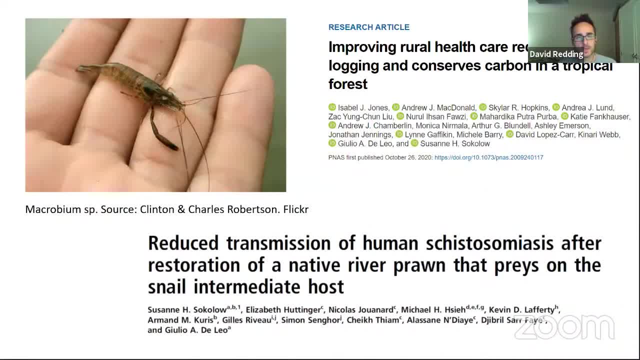 And so this is kind of leading on to some of the work that Susan Sokolow has been has been doing- which I think is a really great body of work, where where she's been looking at her and her colleagues- Obviously there's lots of authors on these papers- but has been looking at how you can actually find these, these kind of win win situations. 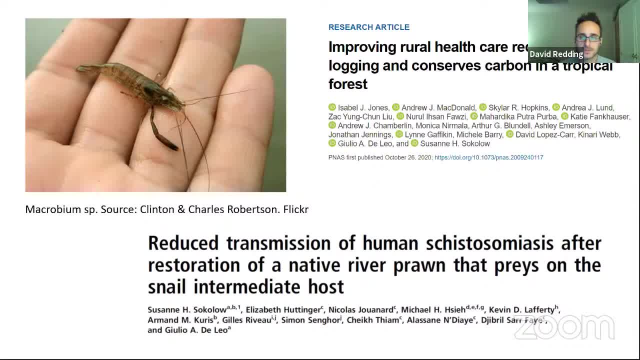 So we've got here a shrimp- It's the wrong species, but it was the best picture I could find- And a very similar species to this in Africa, where we see Adapt. with you down that area. These species can no longer survive. 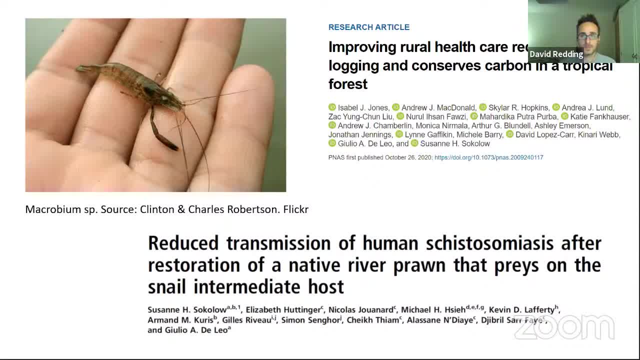 And the snail that then gives people, human schistosomiasis then proliferates and we get these large numbers of disease cases. So by thinking about the health of the biodiversity of the system And and actually restoring the, the rivers, Then we actually see a reduction in in numbers of disease cases. 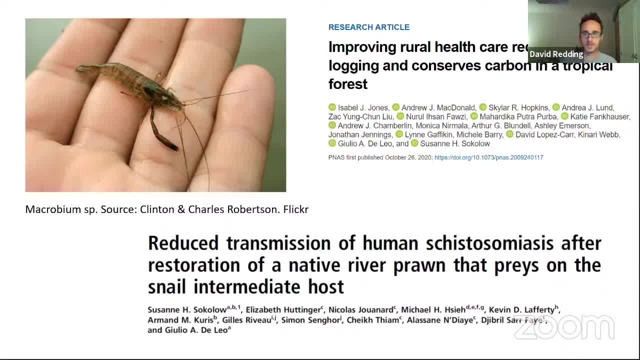 And similarly another paper that's just come out again by a large group of authors, Just come out in October, is looking at how you can actually improve people's lives And actually that reduces the amount of logging and conserves forest areas Such that they are sort of more intact. 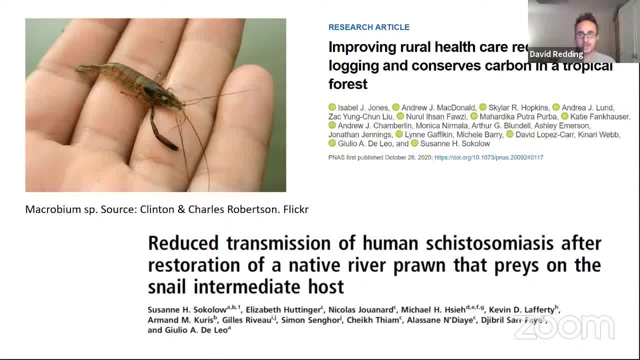 So there's kind of thinking more holistically, thinking about all these different elements And how we can kind of bring them together to to try and benefit both the needs of people, meet these people and benefit the planet. OK, thanks very much. 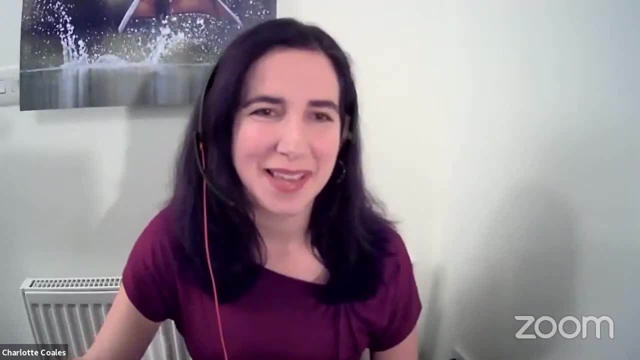 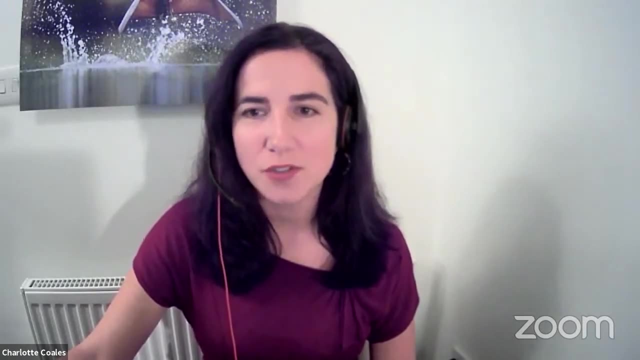 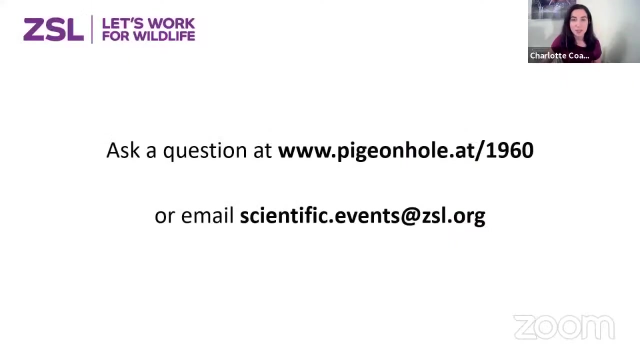 Fantastic. Thank you so much, Dave, for that Talk and also for the examples that you gave too. We have had some questions through already from viewers, But I'm just going to remind everyone, if you haven't already, how you can ask your questions to Dave and the rest of tonight's speakers. 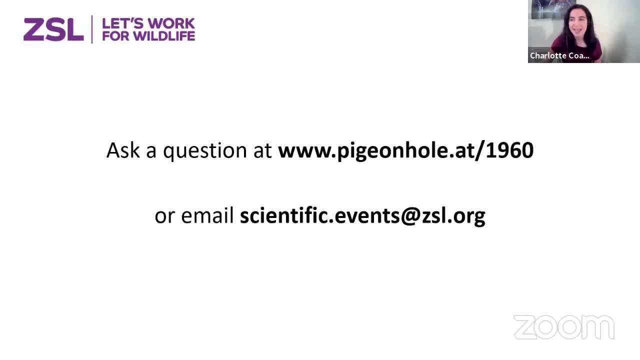 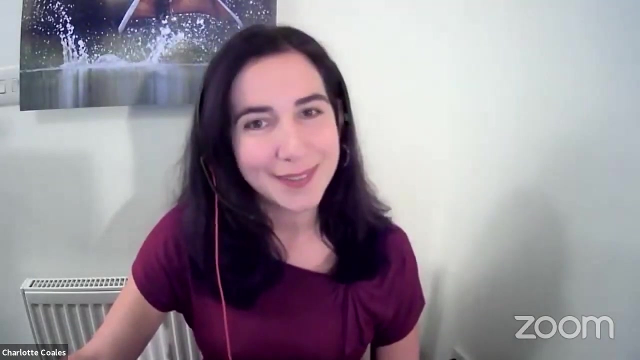 You can do this by either going to pigeonhole dot 80 forward slash 1960 to ask your own question or to upvote other people's questions, Or you can send us an email to scientific dot event At ZSL dot org. As I mentioned, Dave, we have had a few questions through already on pigeonhole and the most popular question. And I'm not sure whether you're in a position to answer this or not, But the most popular question is: is there any analysis of how different places rank in terms of disease risk as a result of habitat loss? Are you aware of any analysis of that kind? 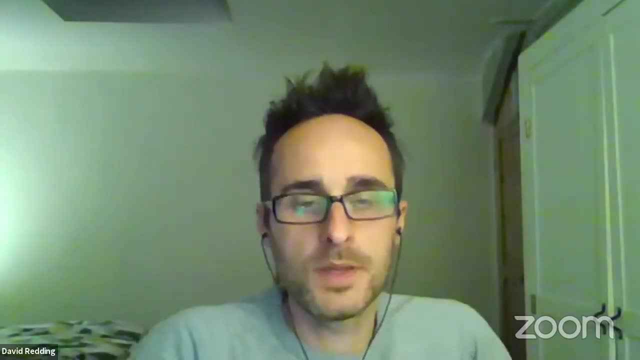 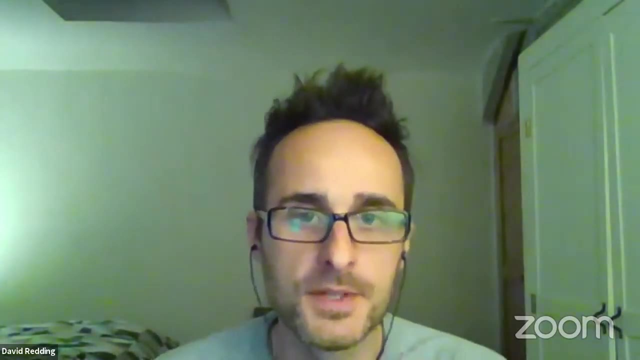 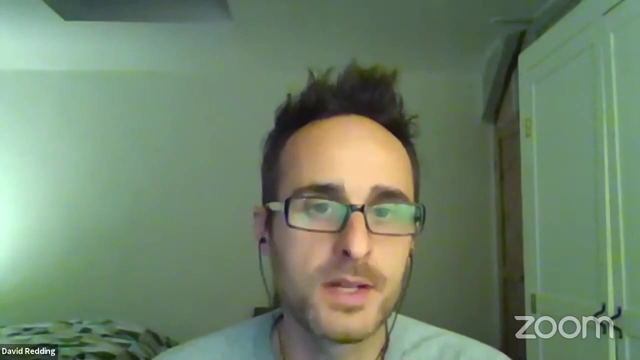 Yes, certainly there are, There's, there's, definitely people have looked at this sort of thing. So Professor Kate Jones at UCL has did a paper in 2008.. That's one of the most highly cited in this area And that's kind of looking at how diseases emerge. 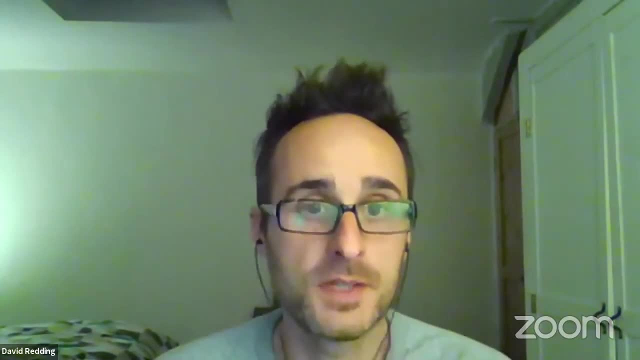 So trying to understand the different drivers at a global level that are causing diseases to start, Diseases to start appearing effectively, And so that kind of looked at things like the total number of species in the area and also the number of the amount of people there. 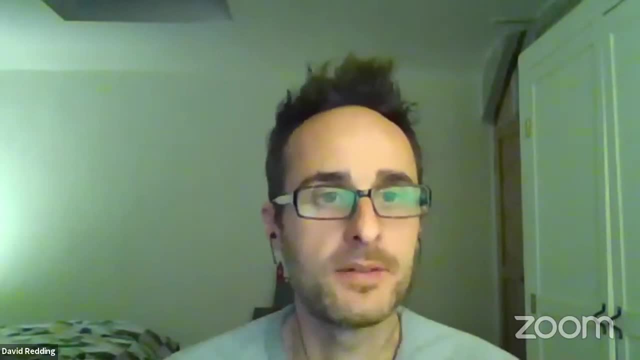 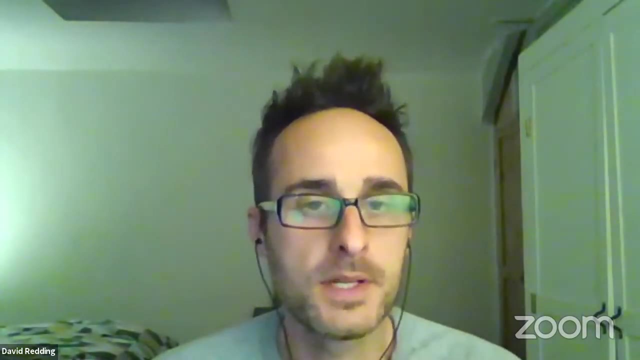 So that's the sort of one index of how disturbed an area might be. is that the number of people? But there's also work by Chris Murray and colleagues, kind of looking at some kind of follow up to some of these These, these questions. So there's definitely, you know, work going on. 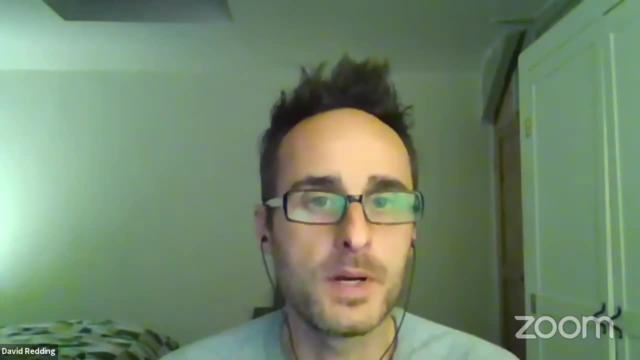 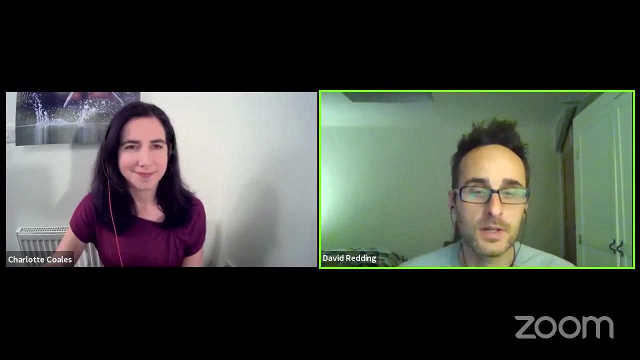 You know, I think, I think also, you know, I think some others, like Barbara Han, has also been kind of looking at some of these sort of global patterns. So, yeah, there is work, Definitely That's that's, that's something that we do need to think about. 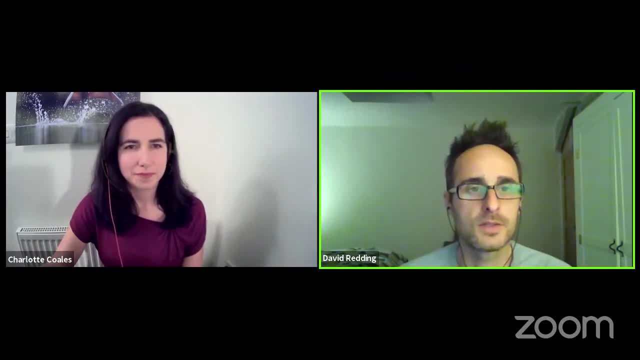 Some of the work that I've done is kind of looked at some case studies such as Lassa fever and Ebola and tried to look at how Sort of current conditions and our kind of future progression of of of climate and land use change is likely to impact. 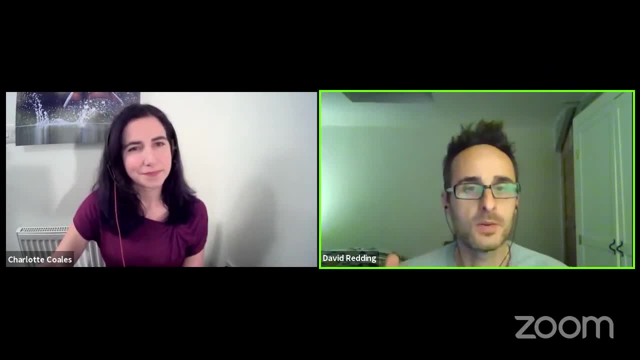 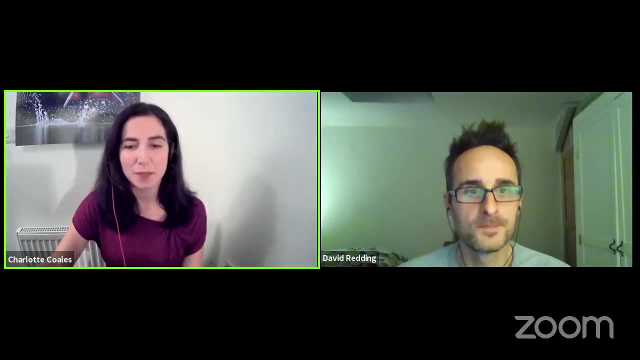 Sort of you know cases, And so it's definitely works on going And I think it's really important to carry on doing that Fantastic. Thank you, Dave. Well, some good, good names there for people to look up if if that's an area they'd like to find out more about. 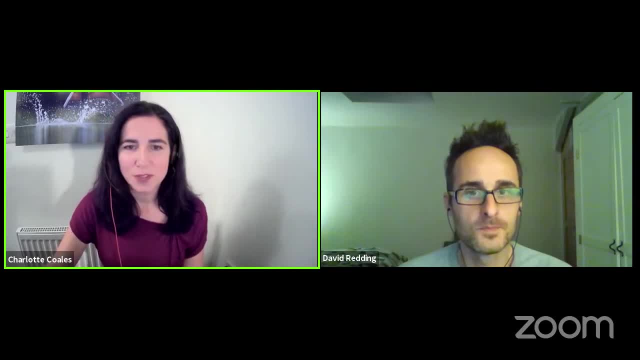 And I'll also ask you one more question before we move on to the other speakers, And that's actually relating to one health that you mentioned in your your talk And the question here from Peter. he mentions that one health is an approach embraced by the scientific community. 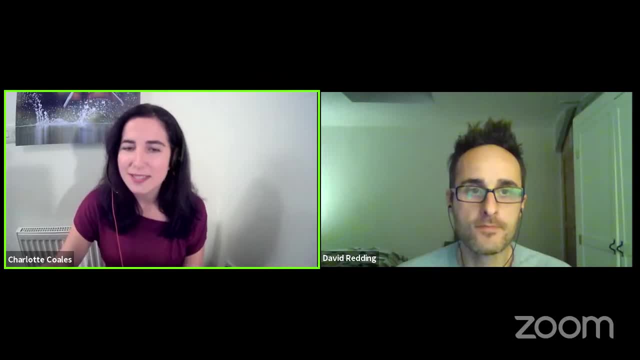 But he feels it's not, doesn't necessarily always seem to be understood by politicians and government departments, And he wonders how you disseminate many of the findings that you're discussing tonight to these, To these politicians and governments. You know how? how do you start to help them to understand the importance of, of this concept of one health? 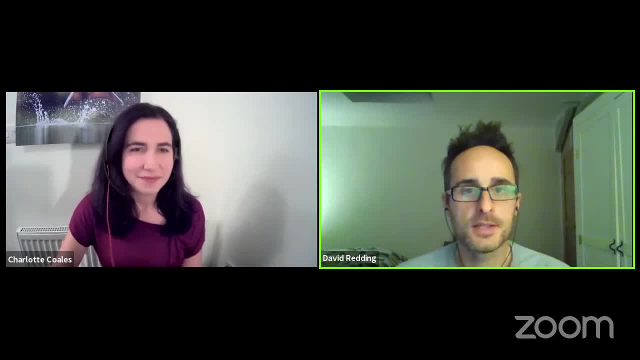 OK, I feel like I have to tread sort of lightly here, because I think there's a lot of interest in a different kind of approaches that are trying to integrate science with with policy. So there's planetary health and one health, which are two big pushes, I think, to try to bridge that gap. 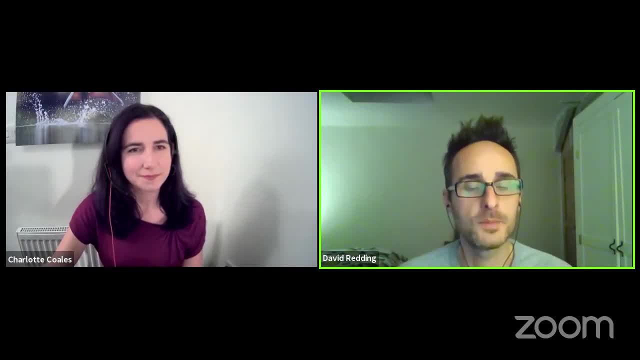 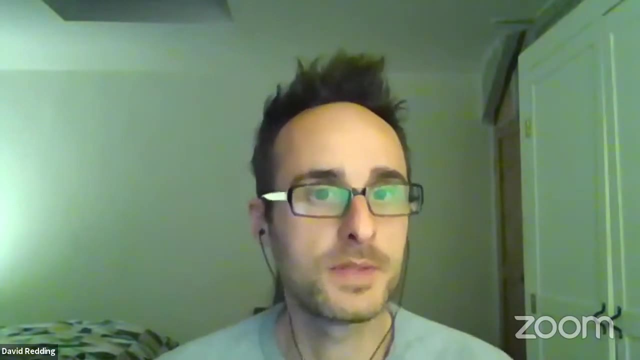 And it's an ongoing challenge. You know, how do we move forward? How do we move from these kind of- you know- scientific studies that are trying to show how things are probably going to change over time under these particular conditions? How do we move to actually saying to politicians: do this, do this. one simple thing. 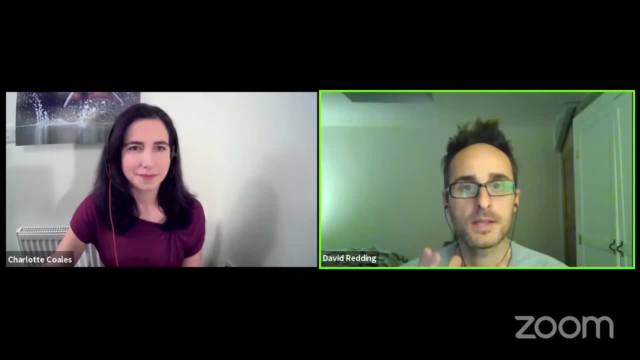 And so that's. that's a continual challenge, And I think that's one of the aims of of of things like one, health, You know, this idea that let's work, let's prioritize all these things. that is going to benefit us, And it's actually a bit like convincing people that that's the case. 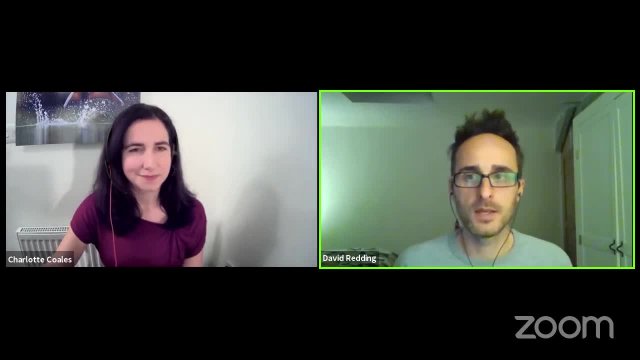 So getting the kind of political kind of leverage. And I think we're in a really different situation now And I think we need to readdress what the political will is now as a result of the covid 19 pandemic, Because I think there's been a huge sort of sudden interest how long term it is. 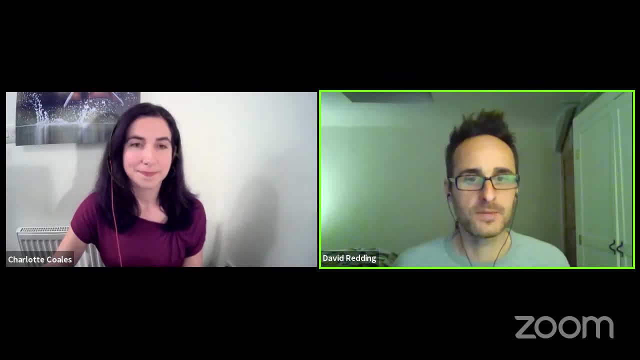 Is. it remains to be seen bit circumspect at this point and and think and actually try really hard to engage um in in effective ways. um, and i think that's about creating, making simple messages and showing these kind of win-win the benefits in terms of of understandable units like: um, how much money you're going to save. 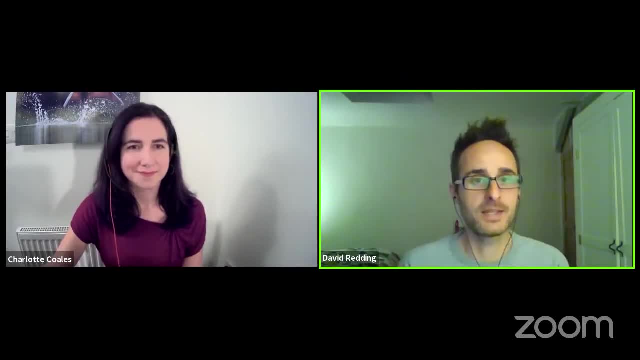 how many lives you're going to save. you know these kind of really basic things that people can understand, rather than some log, odds, ratio or something which scientists tend to talk in fantastic thank you so much. well, um, the questions are coming through thick and fast, so do keep them. 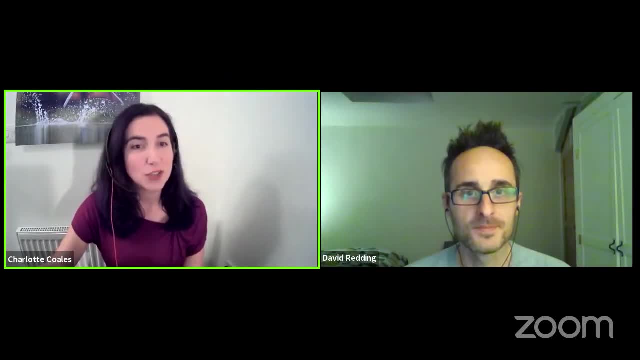 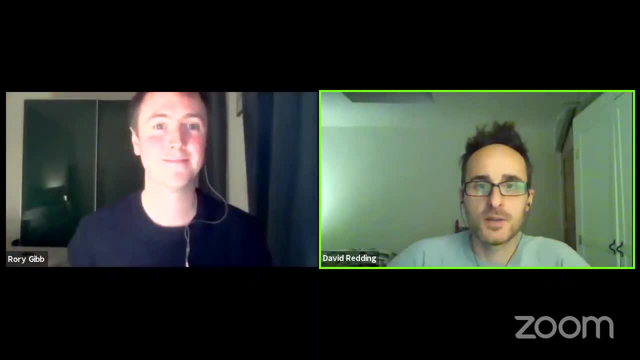 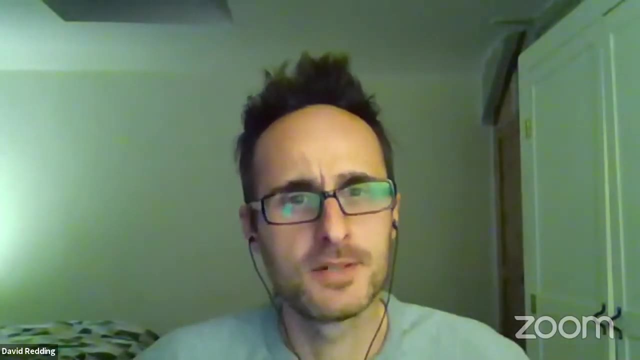 coming everyone i'm now going to hand over to to dave to introduce the rest of this evening's speakers. okay, thanks a lot. so next up is is dr rory gibb, who is a research fellow at the london school of tropical medicine. hygiene, or hygiene and tropical medicine, um and um, he has just uh. 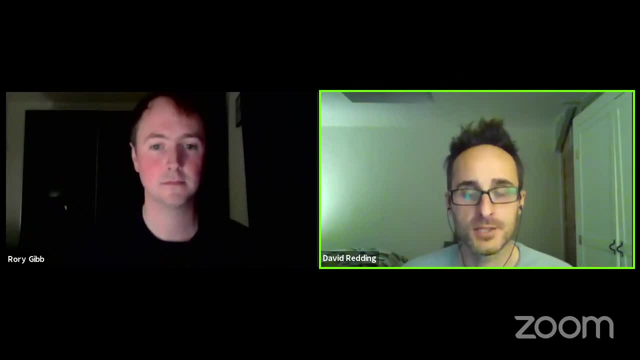 finished his phd um and he's going to talk a little bit more about his research and his research and his work at ucl with um kate jones. i press kate jones i mentioned earlier and his work kind of concentrates on uh, land use change and sort of global change and how it might be impacting. 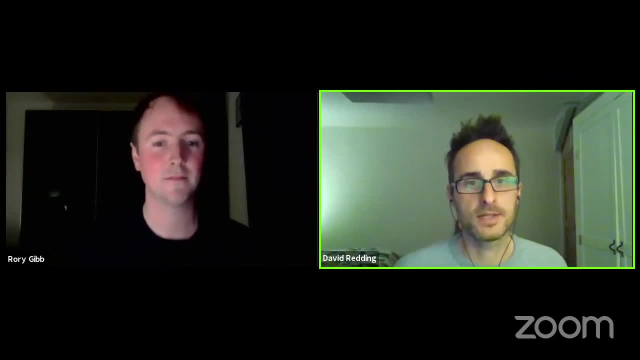 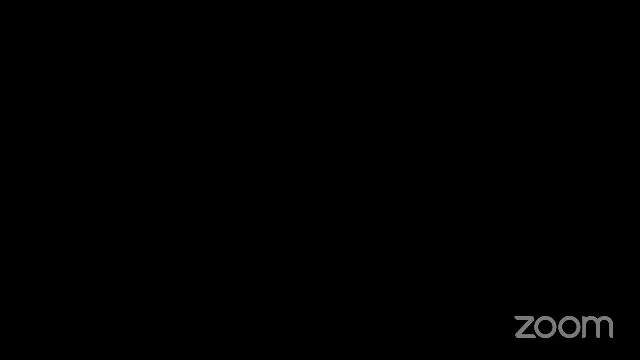 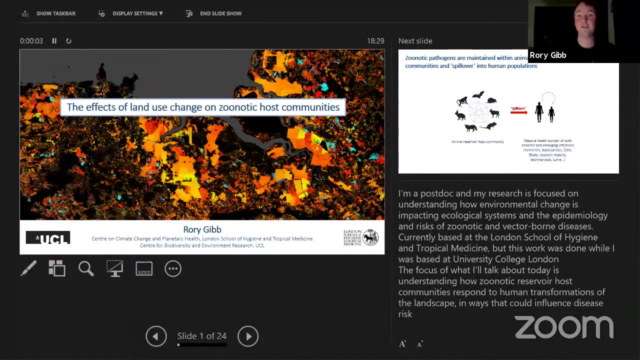 the communities of animals that carry diseases. okay, over to you, rory. thanks. um, i'm just going to share my screen now, okay. okay, hopefully you can all see that. um, thank you so much for the invite to speak. it's a real pleasure to be here, um. so, yeah, my name is rory. i'm a postdoc, um, and my research is focused on understanding, really, how. 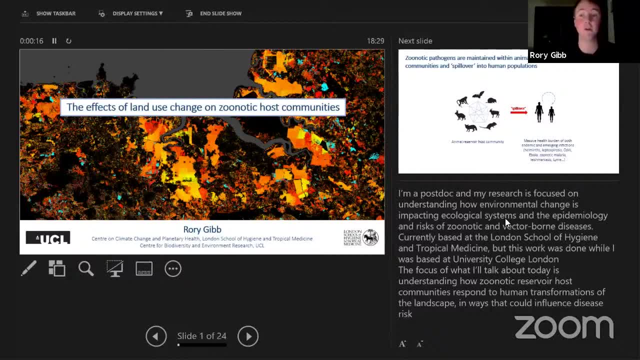 environmental changes are impacting the epidemiology and the risks of zoonotic convective diseases. um, so yeah, i'm currently based at the london school of hygiene and tropical medicine, but the work that i'm going to be talking about now was done when i was at university. 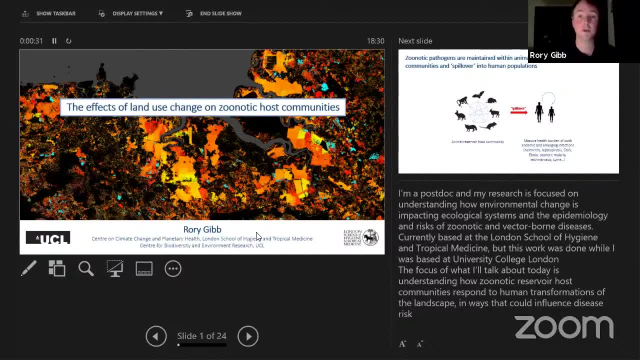 college, london for my phd, and so the focus of what i'm going to be talking about is kind of picking up from where dave left off, really, um, and on understanding how zoonotic host communities or reservoir species respond to human transformation to the landscape in ways that could. 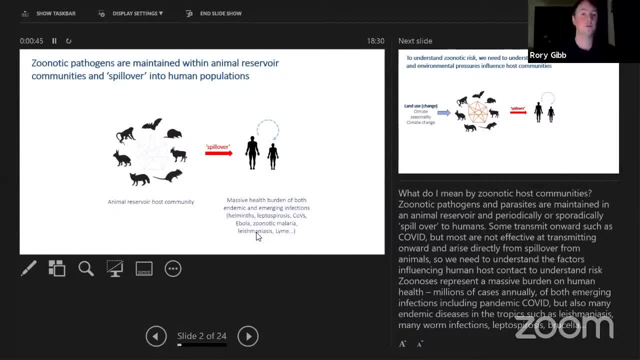 influence disease risk. so what do i mean when i talk about zoonotic host communities? so zoonotic pathogens and parasites are maintained within animal reservoir communities. so you can see here on the slide we've got some idealized community of species in the environment which these pathogens 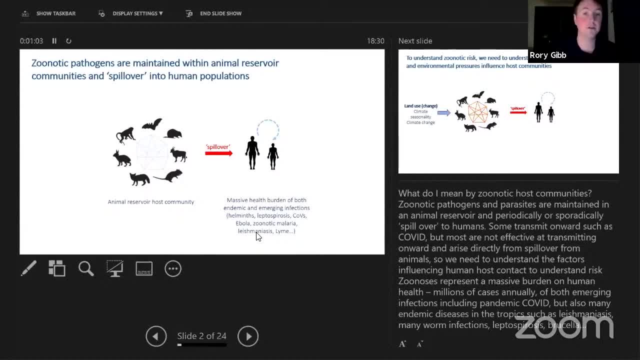 are circulating in, and what happens is that when human species are in the environment, they're transmitting to human populations, and as humans come into contact with these communities, the pathogens can spill over. they can make the jump into human populations and some, in some cases, those pathogens will then be effective at transmitting onward through the human population. so we can. 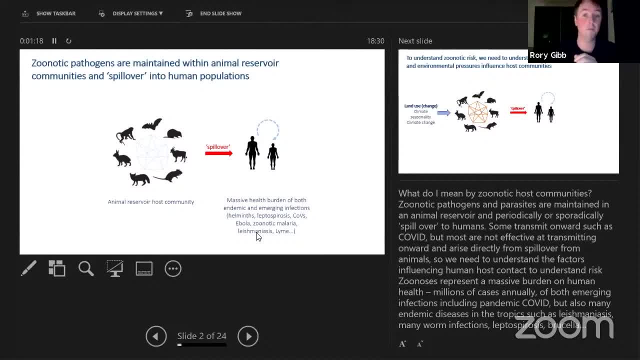 think about covid as a really good example here, right, um? but for the most part, what we find is that zoonoses are generally not very good at transmitting onwards for long- kind of long- periods of time through people. so when we want to understand what's driving the risk of zoonosis, we 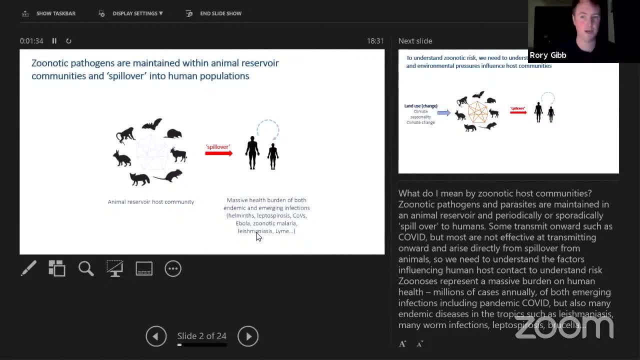 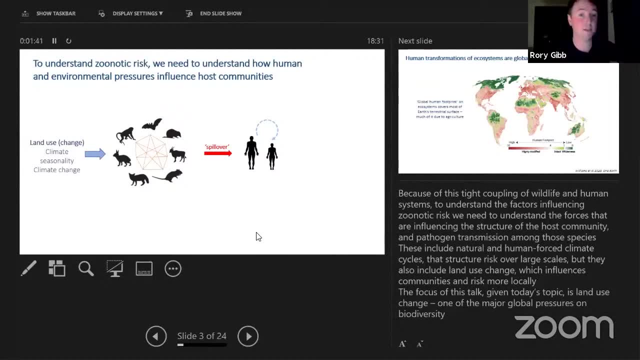 really need to be thinking about what's driving the risk of zoonosis and what's driving the risk of human host contact. what are the processes though creating these contact points and, in turn, because of the way that these human and wildlife systems are coupled? in order to understand what's shaping those risks, we need to understand how human pressures 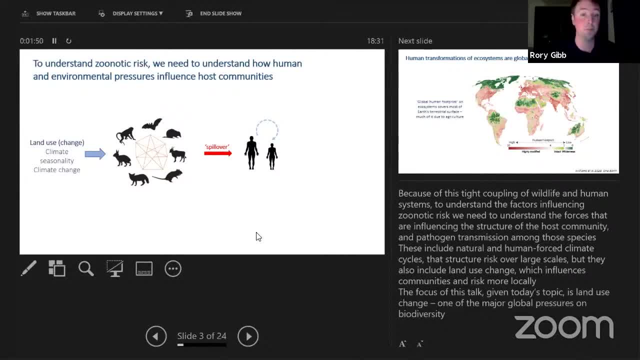 and environmental pressures are influencing those host communities. so this includes things like climate change and climate seasonality. but for today, i'm picking up from where dave left off. i'm going to be talking about land use change. so obviously, the zoonosis is a very important part of the process and it's a very important part of the 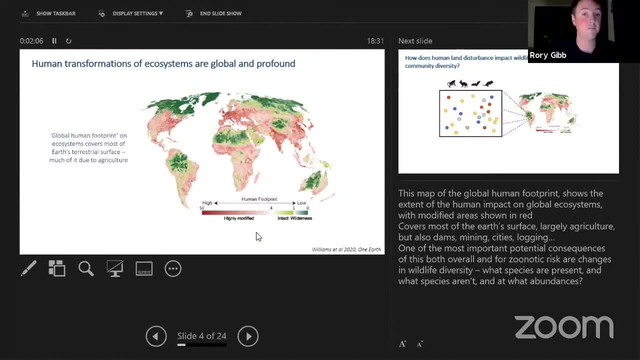 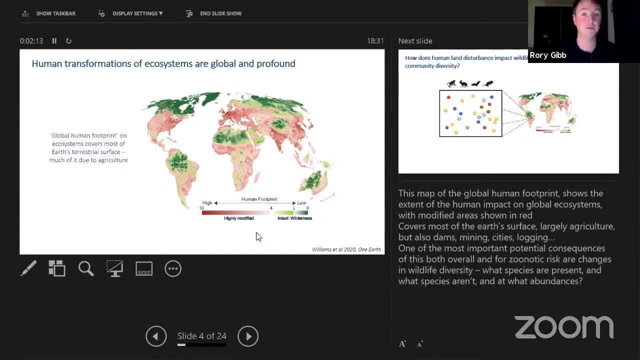 where humans are having a clear and measurable impact on the earth's terrestrial surface. so the clear take home here is that most of the earth's surface is impacted by by humans, much of it due to agriculture and a consequence. one of the questions here is: what's the consequence? kind of 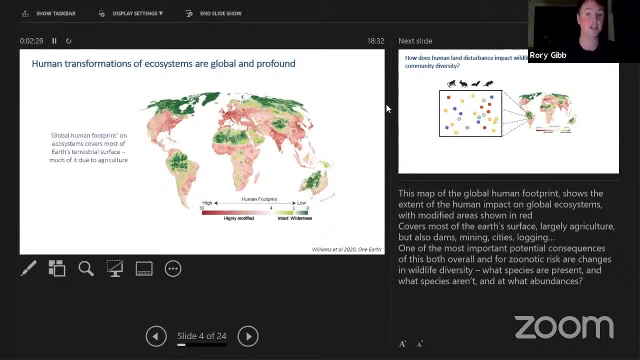 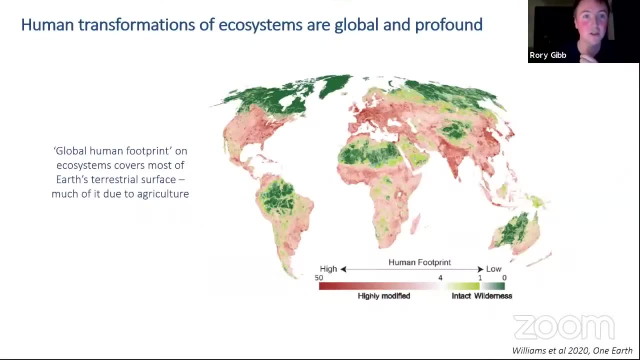 both overall and in terms of, um, changes to the kind of- sorry, can i just interrupt really quickly the notes on your on your slide. if you want to switch to, yeah, sure, okay, brilliant, hopefully that's not been there the whole time, but if it has, i apologize. or um, so yeah, um, what we need to. 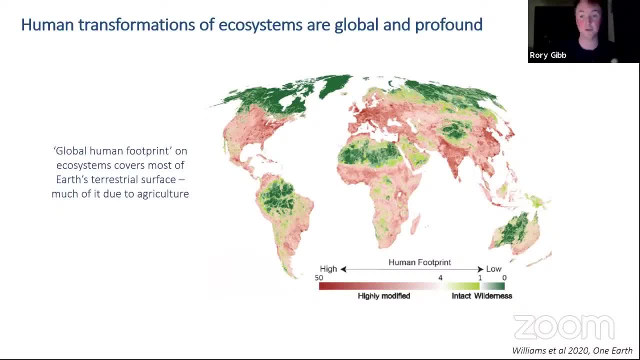 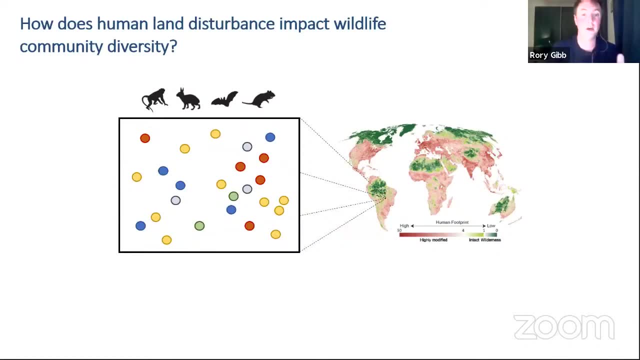 do is really understand how these changes to landscapes are impacting zoonotic host communities. but in order to do that, we need to go out and measure them. so here is a, an idealized ecological community, um, somewhere in brazil, um, and what we can see in the map is that there's a lot of. 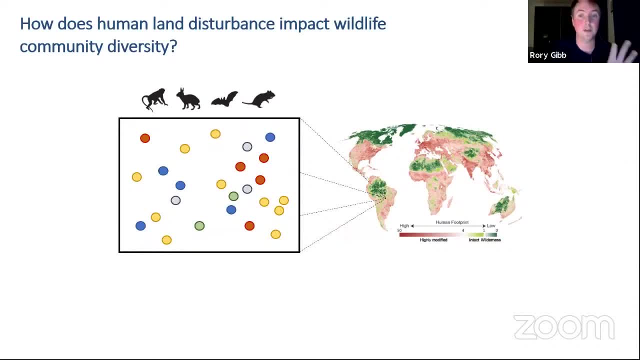 species in this box is these dots. each one of these represents an animals and the colors of these dots represent species, and so if we want to understand what species are out there in the environment, we need to go and survey them, right. so we go out and we catch some stuff. we identify. 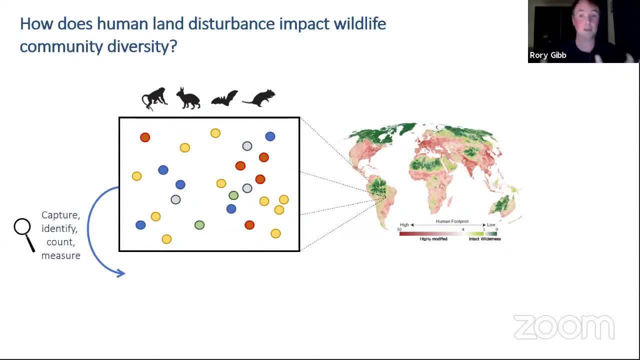 it, we count it, we measure it, and ecosystems are really complex and difficult to summarize, but we can come up with some kind of simple summary metrics which tell us something useful about about what's going on in this ecosystem. right, so we can say that this ecosystem has a species richness of five or five species and a total abundance of 25. 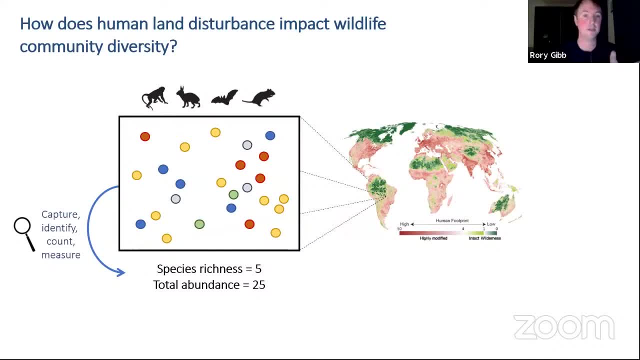 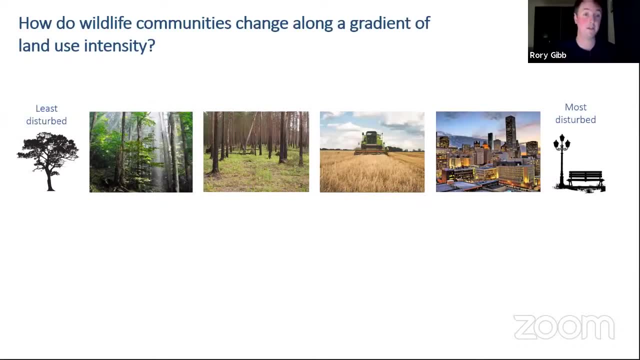 individuals, but what we're really interested in is how are these communities responding to changes to land use? and so, in order to do that, we need to have some kind of baseline to compare to, and so what we can do is use the same methods to go out and survey across a gradient of land use types. 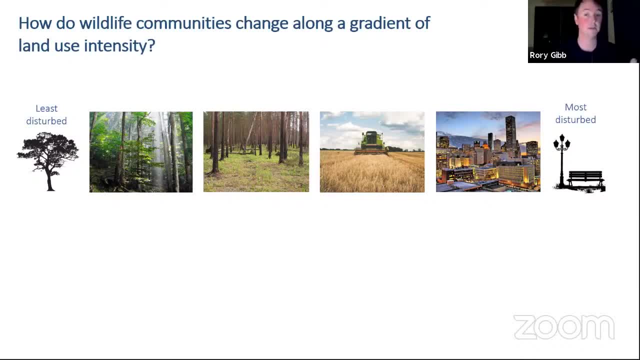 that are experiencing different levels of human disturbance. so we can start on the left here in our least disturbed primary vegetation. so we go out and we survey and we find we've got five species and a total abundance of 25.. and then we can go into secondary vegetation. so here we have. this is vegetation. 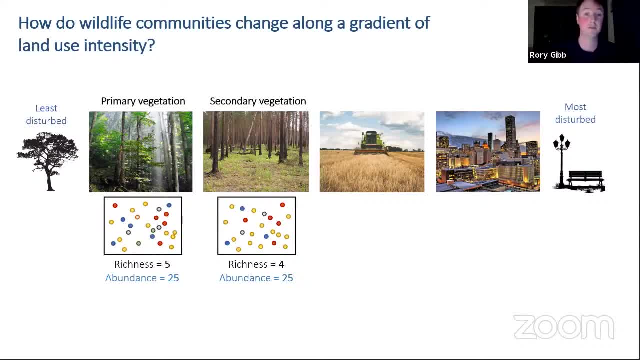 that's natural vegetation but it's recovering from recent human disturbance. and here we've lost a species and we've lost but we've got a similar kind of abundance. and then we can go and survey in some actively managed human landscapes- so agriculture and plantations, and here we've lost. 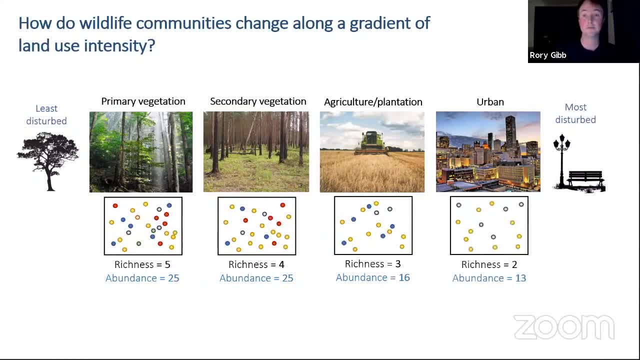 some more species and the abundance has declined. and finally we can go and sample in a city- one of the most kind of disturbed environments you can have- and we find again that we've lost some species and we've lost abundance. so this is a kind of an idealized example of what happens to biodiversity as you're moving along this pressure. 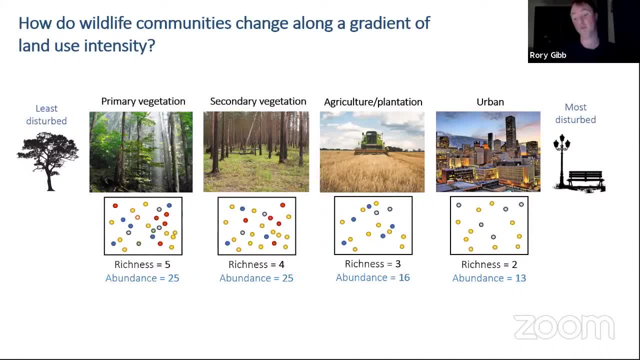 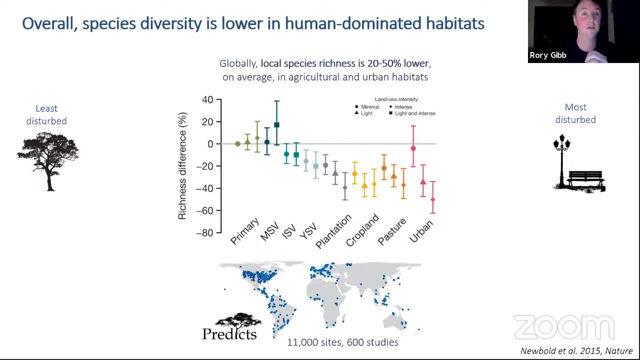 gradient and if we want to understand how this plays out globally, what we can do is basically take loads of examples of people where people have done this kind of study, combine them all together and kind of average them out, and so what we see when we do that- and this is the study actually- that 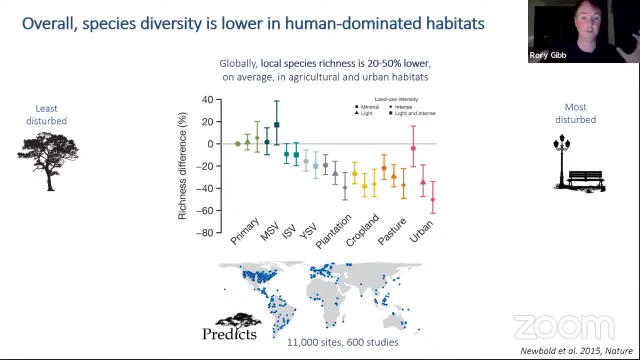 dave mentioned earlier tim newbold study where they've compiled these um these sites from more than 11 000 sites worldwide. is that, effectively, species richness declines pretty consistently as you move into these more agricultural and urban habitats, so as we move away from the primary land. 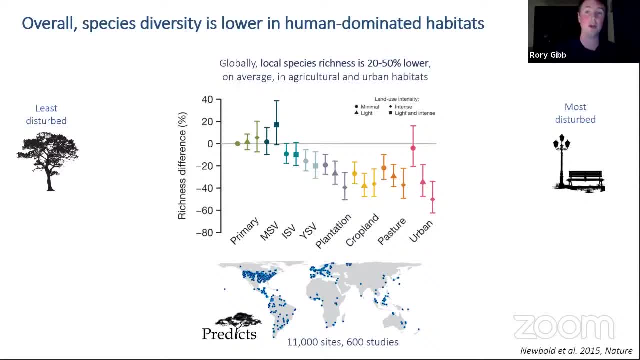 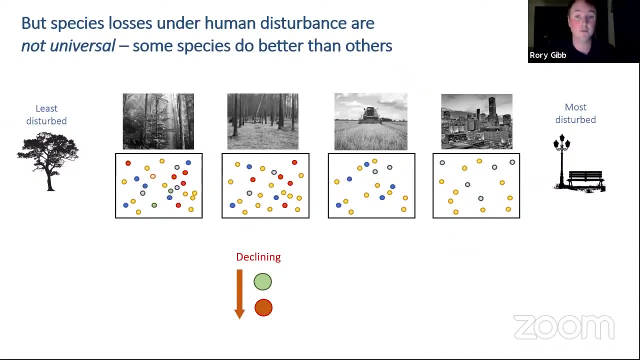 baseline, which we can see on the left of this graph here, into these progressively more disturbed habitats. but this kind of picture of biodiversity overall doesn't give us the full picture, because ecosystems are complicated, they're complex and if we actually look at this example that i've provided here of different 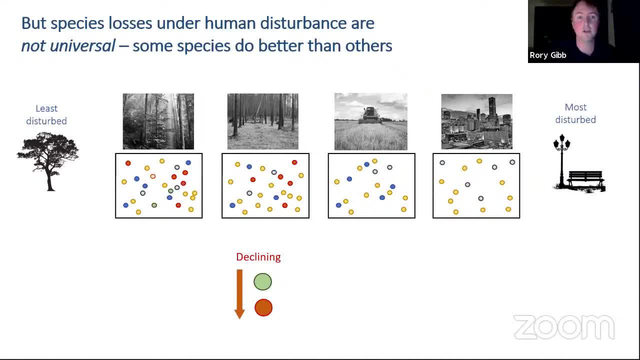 different ecosystems under disturbance. we can see that actually the species losses aren't universal, so not all species are disappearing and some are doing better than others. so on the one hand we can see that the red and the green species are gradually dropping out as we move into the most. 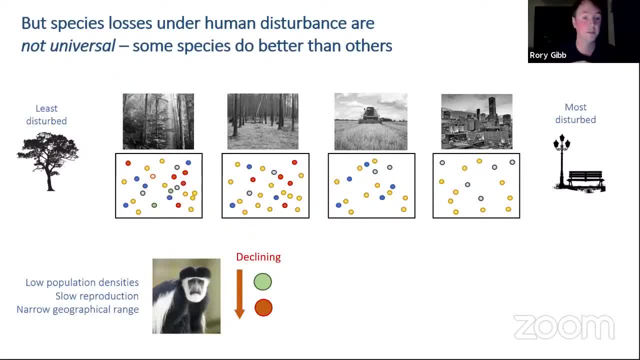 disturbed land uses. so an example of a species like this might be something like the colobus monkey, which tends to be quite sensitive to human impacts and found in less disturbed forest, and there are certain traits that predict where the species are likely to to respond like this. so 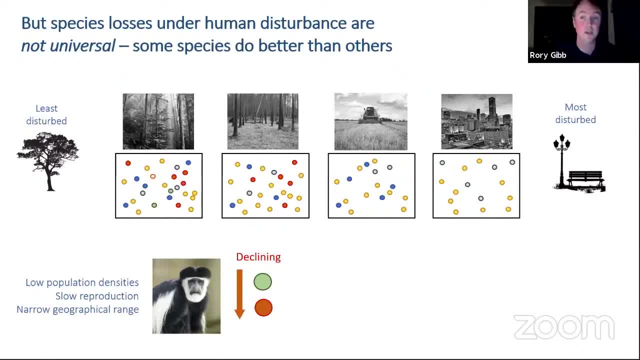 they often live at low population densities, they're slow to reproduce, they're relatively narrow geographical ranges and on the other hand if we look in our kind of urban and agricultural ecosystem we can see that actually the pale, blue and the yellow species are in fact doing really. 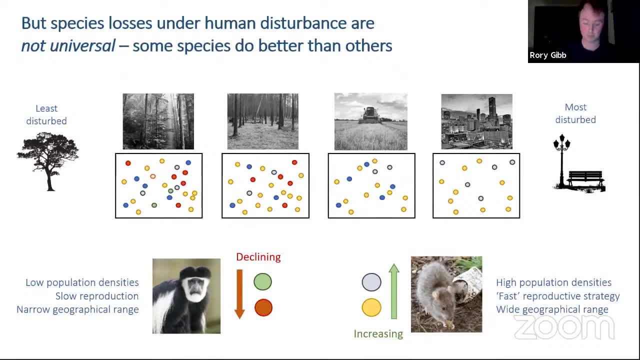 well, they're persisting or flourishing, and so an example of a species like this might be the brown rat. so these are species that live at naturally high population densities, often in the middle of the urban. they reproduce quickly. they have wide geographical ranges, and so the question here. 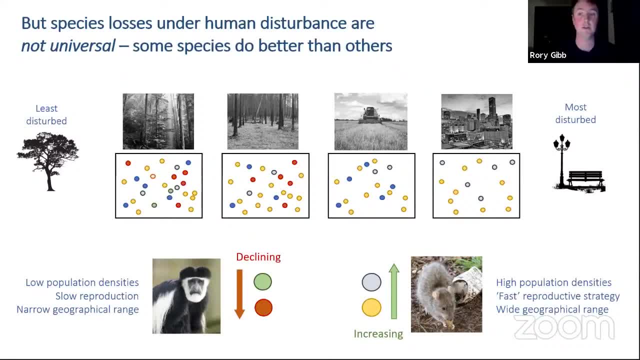 really is. what do these kinds of uneven and kind of non-random filtering effects on biodiversity? what do they mean? and do they mean anything for zoonotic disease spillover risk? and there's a reason to think they might do, because a lot of these traits that predict 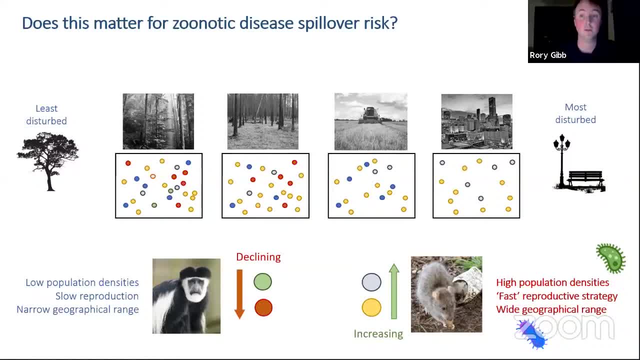 whether species are more likely to persist are often things that are associated with being more likely to carry zoonotic pathogens, and so what we were interested in doing was finding out, you know, what are the effects of zoonotic pathogens and how do they play out? so effectively do hosts? 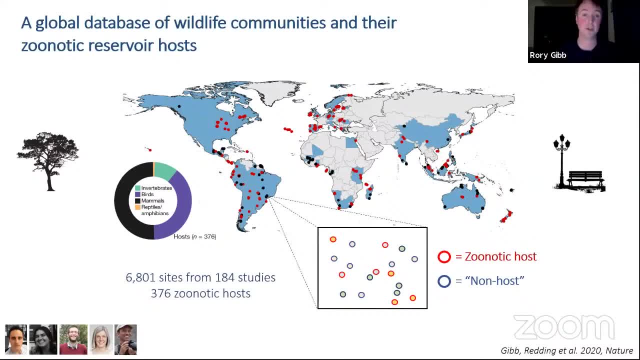 respond differently in some way than biodiversity overall, and so what we did was to take the same database that was used for tim's study earlier, so this huge database where people have gone out worldwide and sampled across all these gradients of disturbance and rather than just looking at 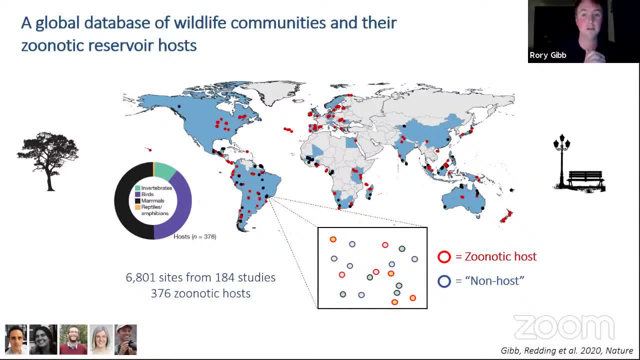 biodiversity overall. what we do is we identify those species in the community- which you can see in this box ringed in red, that we know are reservoirs of zoonotic pathogens, so pathogens that can infect people, and then what we can do is effectively compare the responses of those species to the responses. 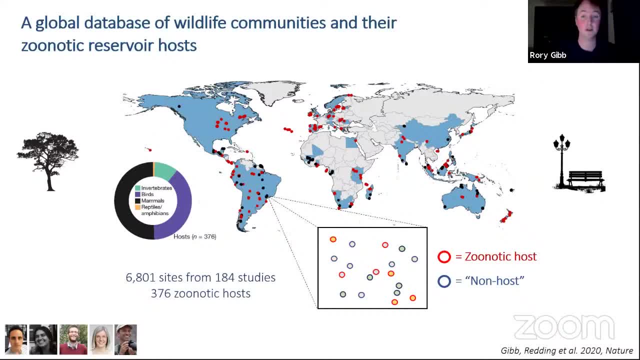 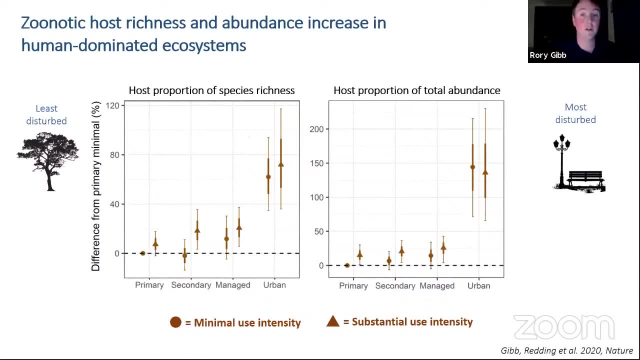 of biodiversity overall, which we consider to be non-hosts, and ask: are hosts doing something different? and when we do that, what we find is is a really interesting result, right? so what these graphs show, firstly, on the left is the proportion of the total species richness in the community that's taken up by host species and on the right the proportion. 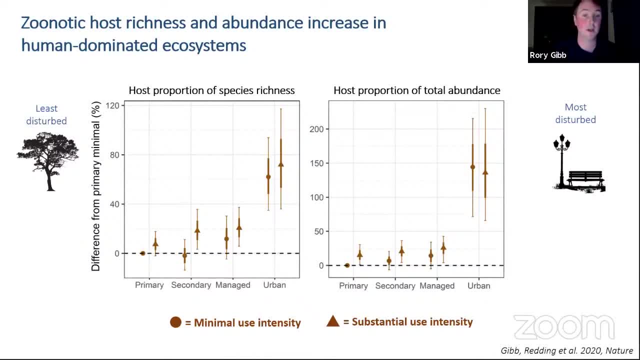 of the total abundance, of the total number of individuals in the community that's taken up by host species, as we move from primary minimal use landscapes on the far left through progressively more disturbed landscapes, as we move rightward on the graph, and if we're above the line, we're 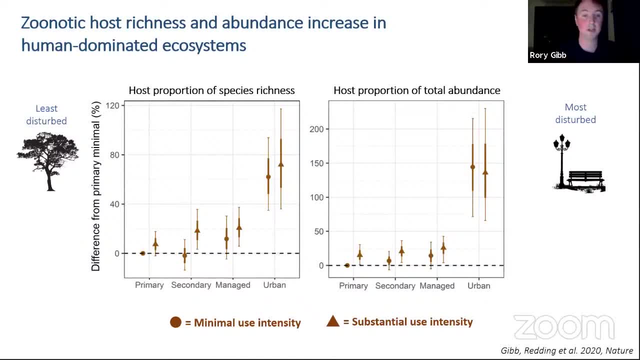 increasing, and if we're below the line we're decreasing, and so what we see, the kind of key take-home here, is that as we move into more intensely used landscapes, both within and between kind of categories of land use, we see this kind of increasing shift towards communities that are 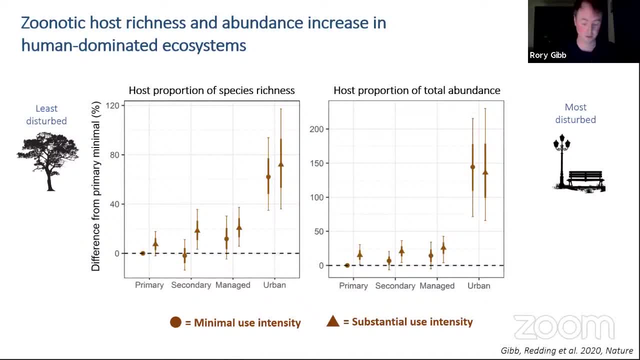 dominated by zoonotic species, host species to species that can transmit pathogens to people. So there's some kind of systematic filtering effect going on here in these ecosystems, where we're losing the non-host species and those species that are more likely to transmit pathogens to people. 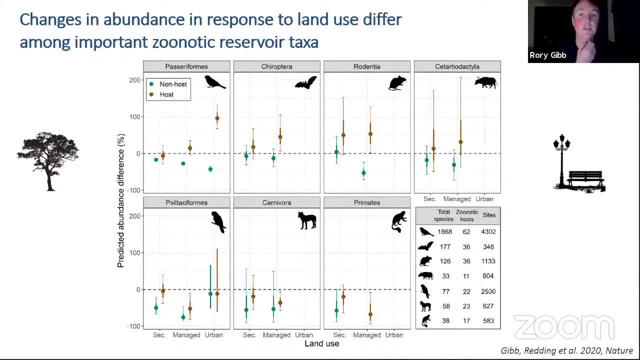 tend to persist. But if we dig into this in more detail, what we can see is that actually these effects aren't universal among different types of species that are more likely to transmit pathogens to people. So what these graphs are showing is something similar to in the. 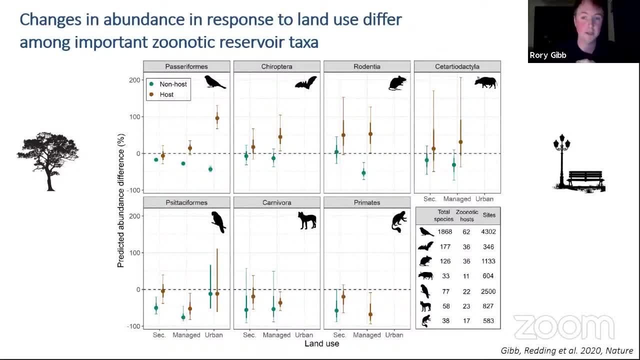 previous slide where, along the x-axis, what we can see is different land use types are secondary, managed and urban, And what our points and error bars are showing is effectively the average response of species, the average change in abundance of those species as we 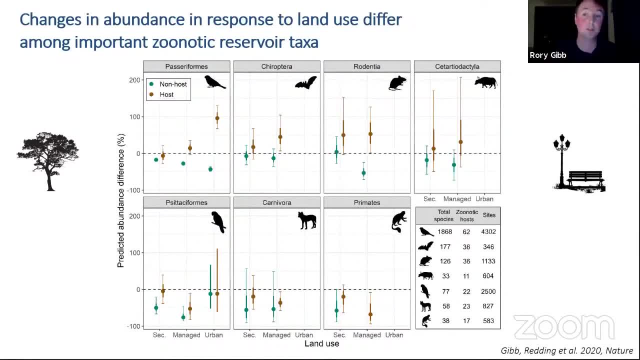 move away from primary undisturbed habitat into these progressively more disturbed land uses, And what we do is we partition this out among host species and non-host species, So hosts in brown, non-hosts in green, And so the kind of key take home here really is: 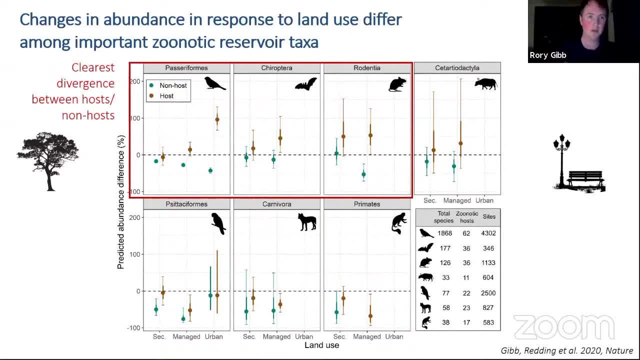 that actually what kind of species group you're in matters. So we see this kind of very clear divergent response in terms of abundance between host and non-host species within these orders for passerine birds and for bats and for rodents. So as you're moving into more human-dominated 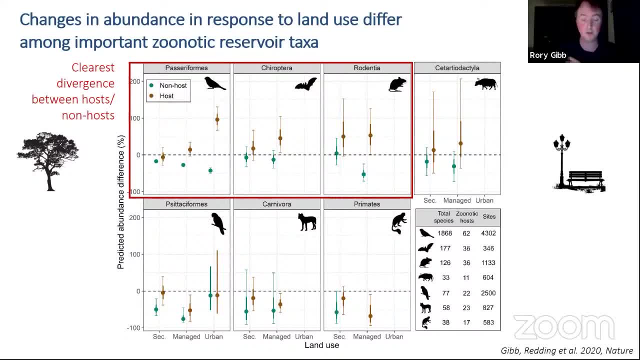 landscapes, this filtering effect is really strong and we're left with communities dominated by hosts, Whereas, in contrast, we're left with communities dominated by hosts. In contrast, if we look at primates and carnivores, we see pretty similar responses to land. 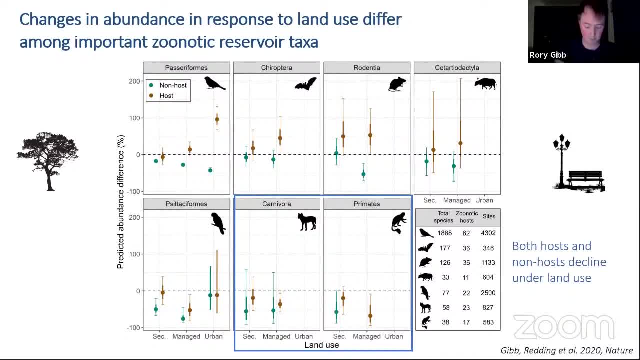 use, regardless of whether you're a host or not, And so what this means is that we're likely to see different kind of types of landscapes being potentially riskier for contact with different kinds of host communities and different kinds of diseases. So, for example, we might 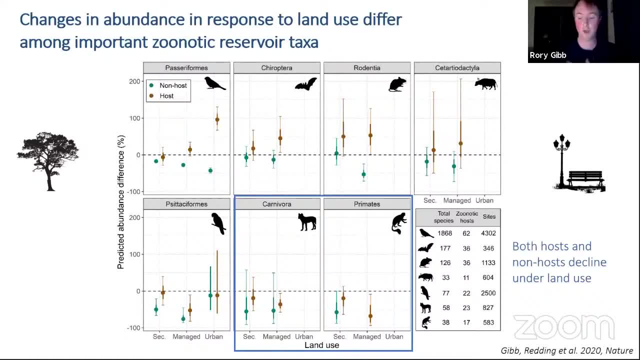 be more likely to come into contact with primates and carnivores in these kind of more mosaic, partly disturbed, partly edge habitats, Whereas maybe we're more likely to encounter rodents in these more intense environments, And so we're likely to see different types of landscapes. 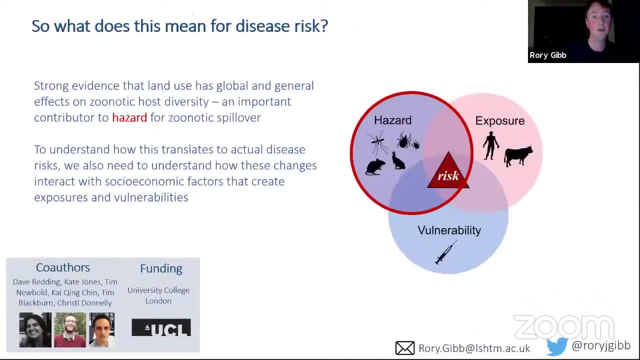 and different kinds of habitats, And so we're likely to encounter rodents in these kinds of environments. So we can think about this as being an important contributor to the kind of hazard for zoonotic spillover. But if we want to understand how risks play out, we also need to understand 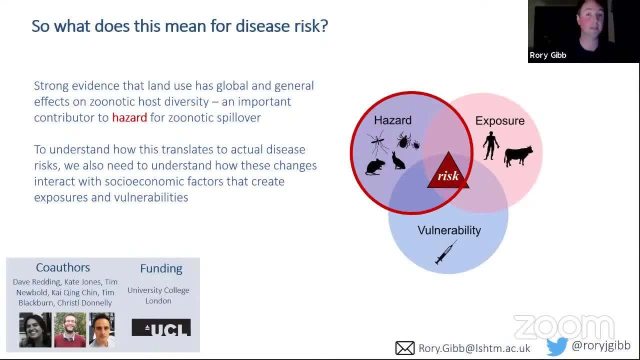 what are the factors that are influencing people's exposure and their vulnerability to these hazards? I think, kind of moving beyond this ecological only perspective, what we need to think about is what are the kind of socio-economic factors that are creating exposures and vulnerabilities to these kind of hazards that are changing systematically worldwide. so, um yeah, thanks. 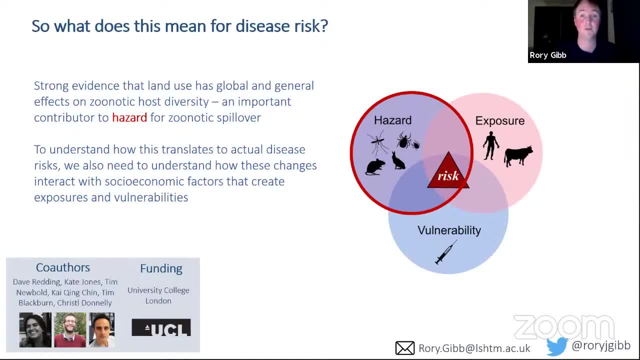 very much and, yeah, thanks to my co-authors and to UCL for funding this. thanks very much, Rory. that was a really great talk, um very clear, which was really brilliant. so, um just having a quick look at some of the questions coming up, uh, let me just have a. 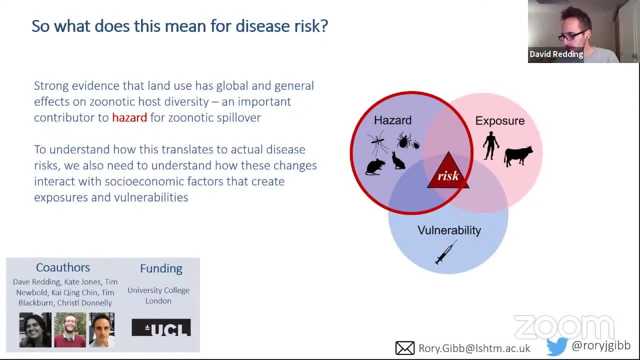 quick look. so just in the meantime, just a question I was thinking of, you know, is there what? what can we do? is there, is there any sort of take-homes in terms of how, of how we should sort of move forward in the future in terms of landscapes, you know? is there something things? 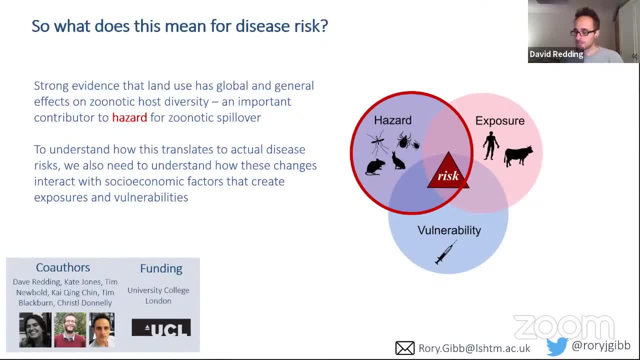 that we can do, uh to try and to try and prevent um or try and help human health in the future. so I guess one thing that I feel like this kind of result speaks slightly to is this question about how intensely we use landscapes, um. so what we see quite clearly is quite a strong effect of 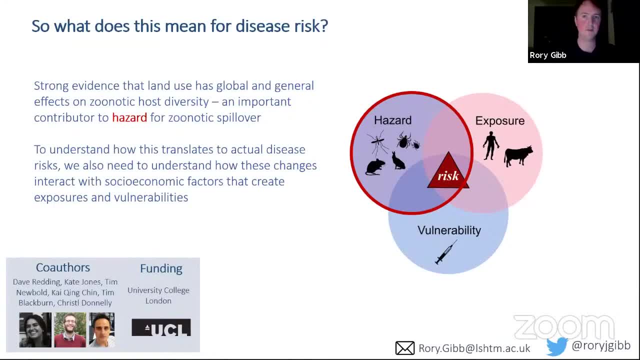 of land use intensity on this filtering effect. so even if you're in an agricultural landscape, the landscape is being used kind of less intensely, the filtering effect is less strong. so I think this raises some interesting questions about how it is that we can kind of design landscapes in ways that um kind of help to preserve the kind of 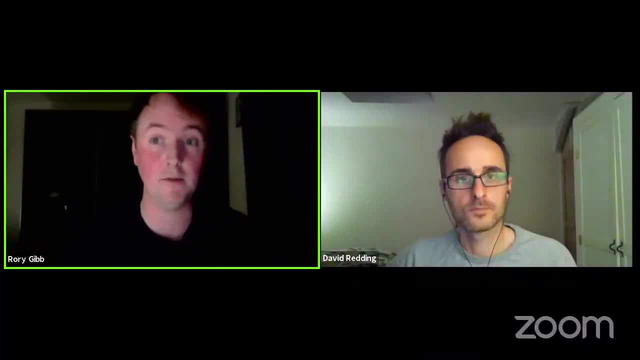 natural regulatory functions of ecosystems and biodiversity and kind of help keep those populations, um kind of hosts, in check, um. so you know, like I suppose, speaking to your point about um food security, you know it's like kind of how can we ensure food security while also kind of helping to regulate these populations naturally? I think is a really important question. 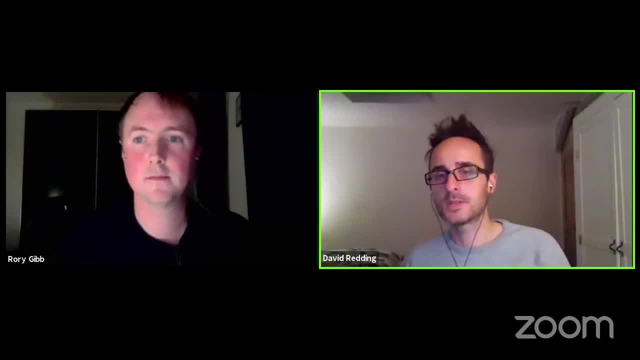 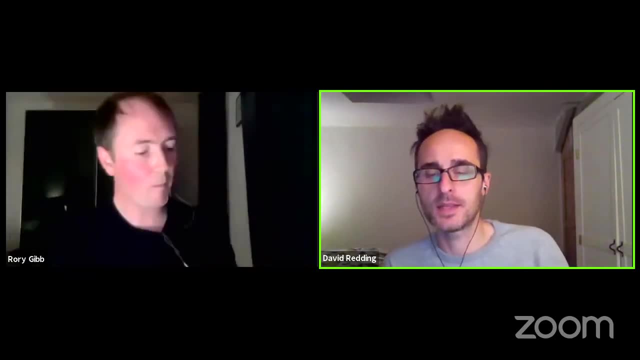 for the future, um, okay, so. so, leading on from that, we've got a question about um food security says: is there an you know of where holistic thinking has been achieved to ensure food security and biodiversity security at the same time? obviously, if you don't, don't know, don't you know? 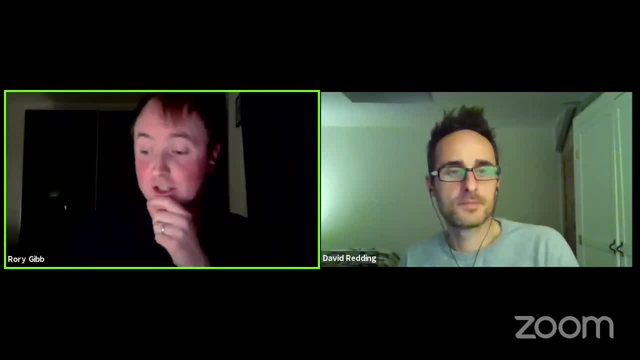 that's a good question. there are a lot of examples of it and none kind of specifically springs to mind. i think there's one example from a disease risk perspective, which is actually the work that you referred to of suzanne soccolo and some of that group. 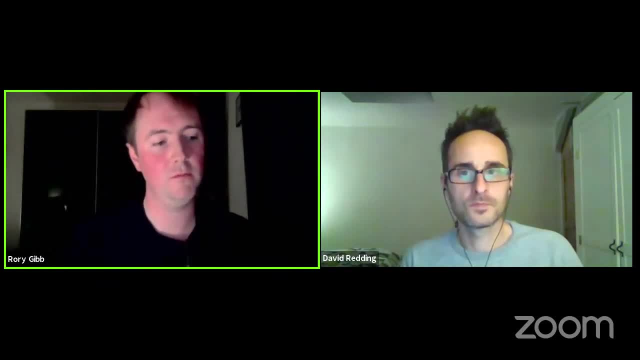 that have been trying to think holistically about how you maintain kind of riverine ecosystems in ways that regulate disease risk while also providing food security, because you can. you can raise these prawns in aquaculture and use them as a food source and also use them as a. 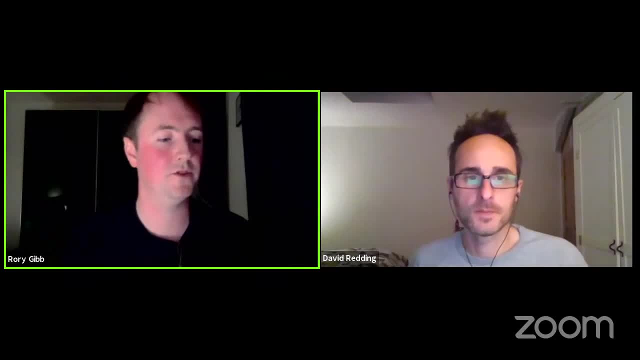 kind of an economic product. so these are the kinds of, i suppose, sort of planetary health and one health focused solutions that are thinking about how you achieve kind of net benefits to all sorts of different kind of ecological outputs. um, but yeah, i mean it's a huge area and i think there. 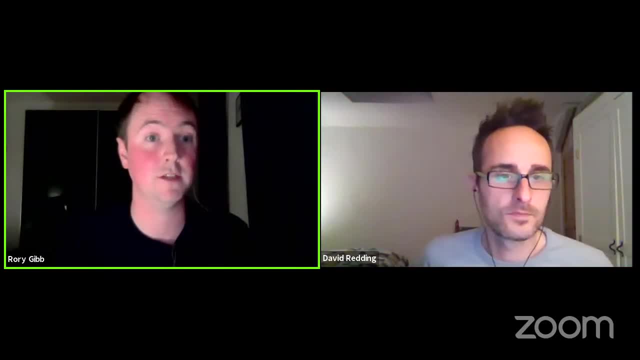 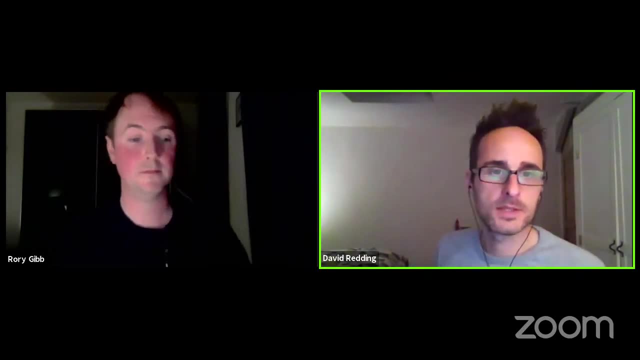 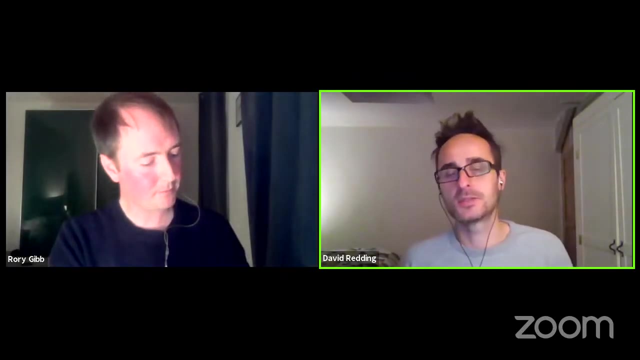 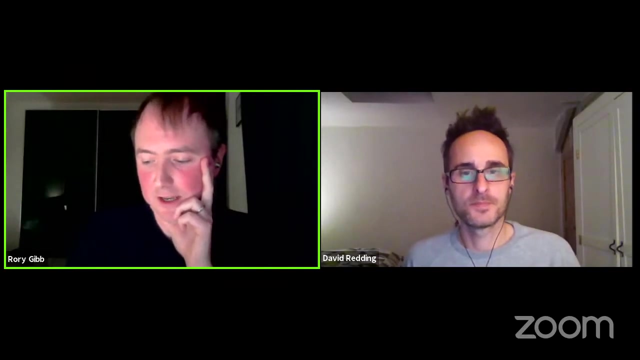 are many examples of where people are trying to reconcile food security with biodiversity conservation more as well. okay, great and a lot. one final question is: um, is there- sorry, is there- a correlation between more resistant or tolerant animal species and the occurrence of pathogens? so that's a good question and i think it's a really um, it's still quite an open question. i. 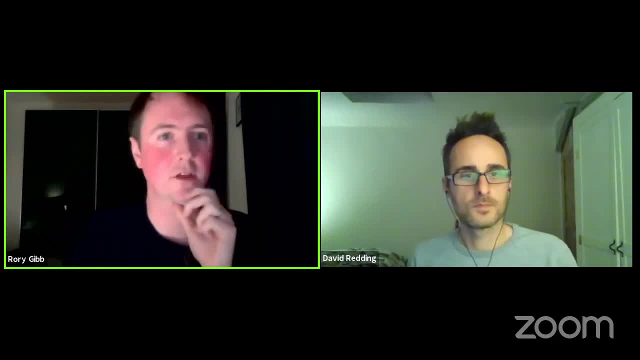 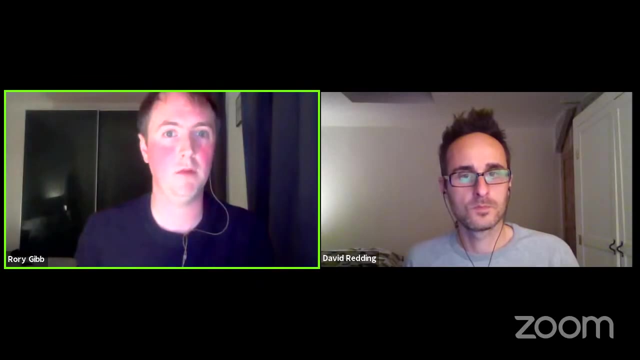 think in this field, um, and it speaks a bit to the dilution effect stuff that you were talking about earlier, um, so there's kind of a lot of discussion around kind of the role of different species, um, abilities to host pathogens, um, and kind of what we call competence, um, and what kind of aspects of 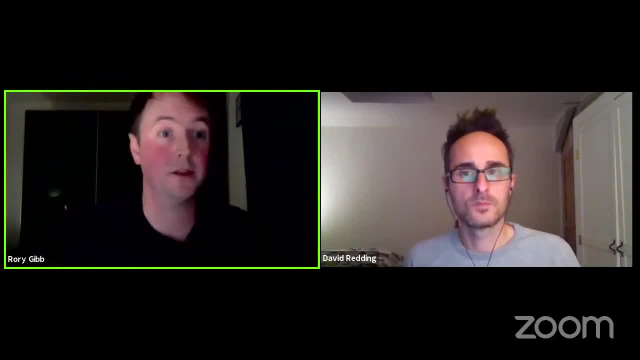 of species, make them more likely to hope, to make them better hosts of pathogens. i think there's kind of on the one side there's people that think that fast living species are very good at kind of hosting pathogens because you're constantly replenishing your population and living at high. 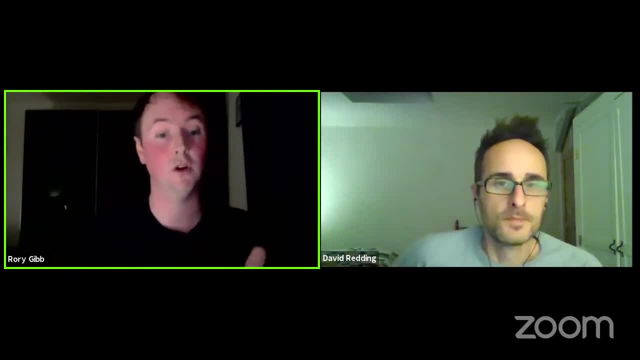 density, so pathogens can spread really quickly, and so i think there's a lot of discussion around that in the contest itself. but that's something questions, yeah, yeah, so i just want to point out that we and in a very limited time and very limited ability for species to, because of their unique 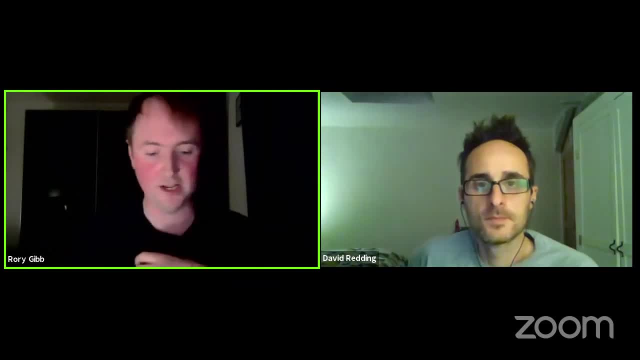 significance in ab Romania are veryり well. on the other hand, you've got longer-lived species that can kind of persist with these pathogens and transmit them among themselves very slowly. so the pathogens are more likely to persist and i think it's still an open question about what kinds of 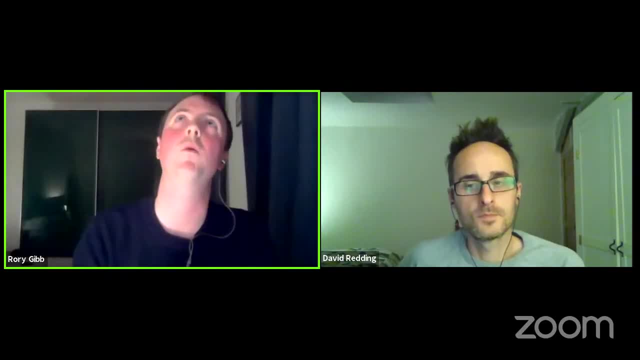 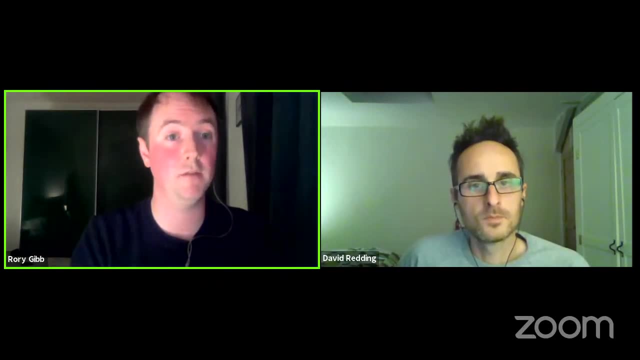 species we um need to be thinking about in terms of what kinds of risks, and i think the short answer is that it's probably likely to be quite context-dependent a lot of the time. i think these kinds of general analyses can get us so far, and then you get to the point where you, you know you. 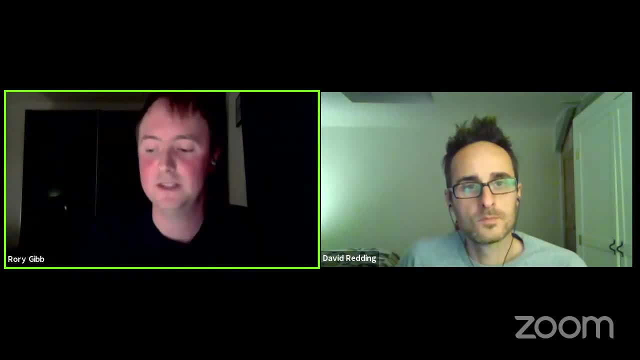 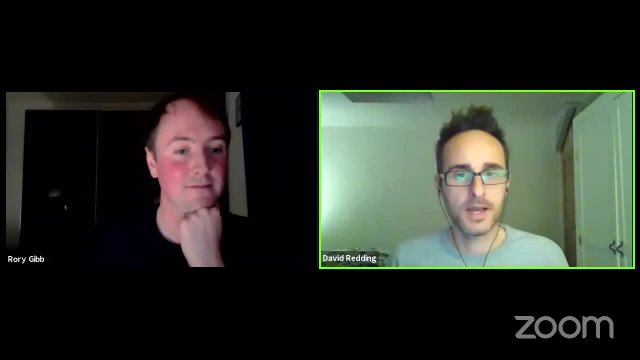 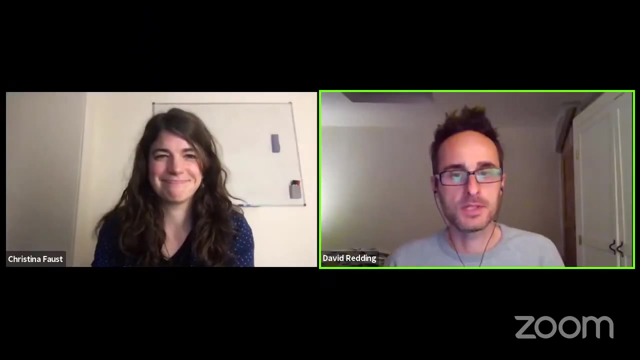 start really needing to think about what are the kind of context specificities to your particular disease you're interested in in terms of managing that risk. Great, well, thank you very much for that. that was great, Okay. so our next speaker is Dr Christina Faust. Christina is a research scholar. 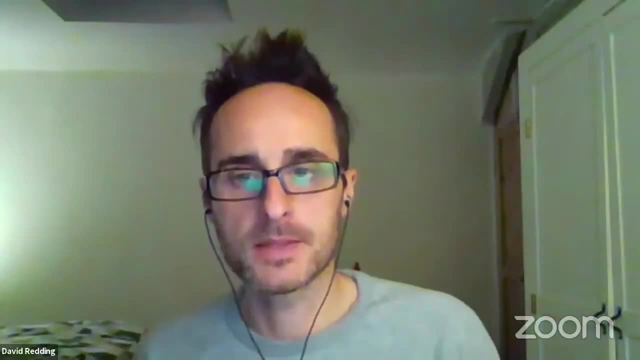 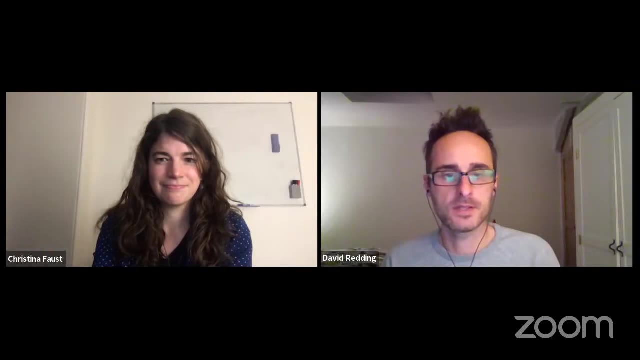 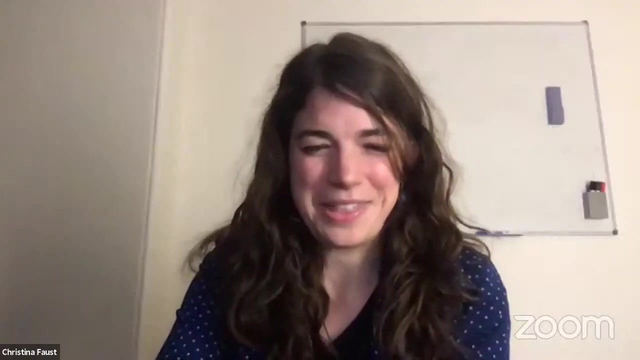 at the Center for Infectious Disease Dynamics at Penn State University. Her research focuses on environmental change and infectious disease dynamics, particularly looking at human and domestic animal diseases. So thanks very much for coming and I'll hand over to you now. Thanks so much, Dave. Thanks for having me. Hi everyone. I, like Dave said, I'm going to be. 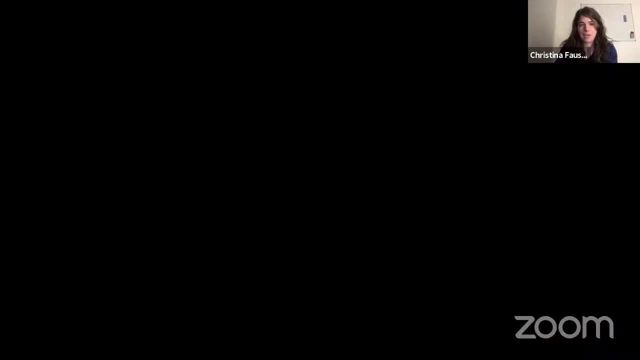 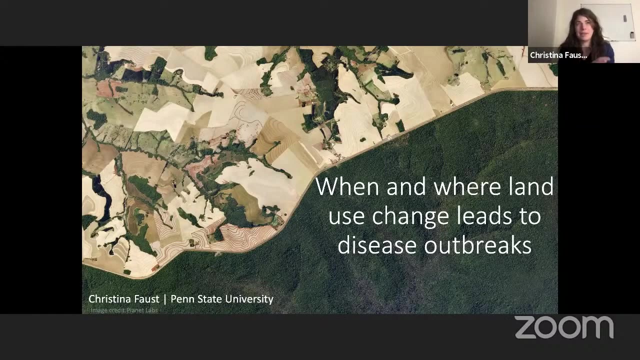 talking to you about the disease dynamics at Penn State University. So I'm going to be talking to you today about some of my research and kind of generally what we think about when we think about land use change. So this image has been on all the promotional material. 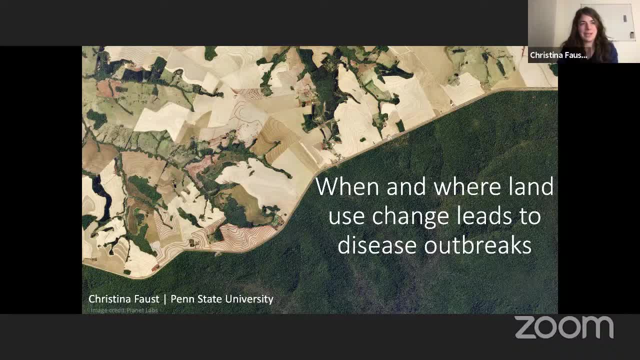 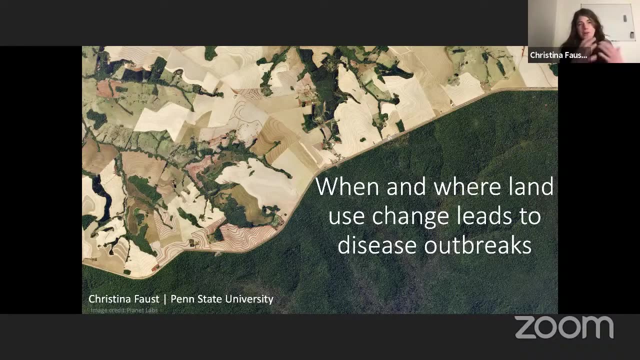 so hopefully you've seen it before, but it's one of my favorite images. It's taken from a satellite run by Planet Labs, but it's in the Amazon rainforest and it clearly shows how protected areas can help preserve this natural habitat. And on the other side you have a very human, intense landscape that's intensely managed for. 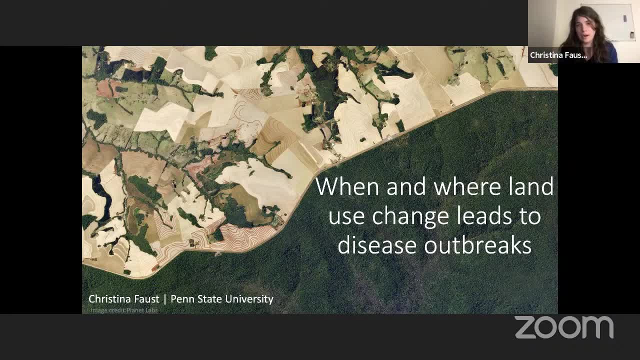 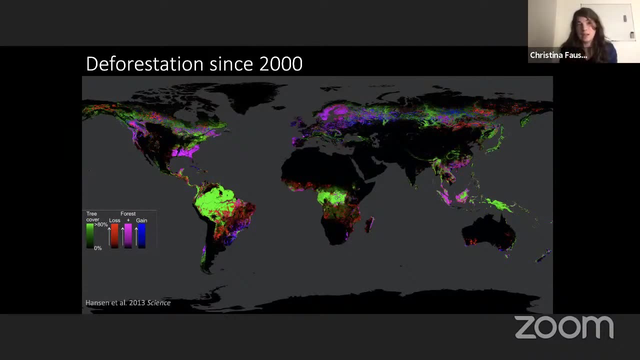 agriculture, but the human density is relatively low there. So this is the case in the Amazon, but we also have this occurring around the globe. So this is an analysis, using satellite imagery at a 30 meter resolution of forest cover around the globe. So in green areas we have areas that are 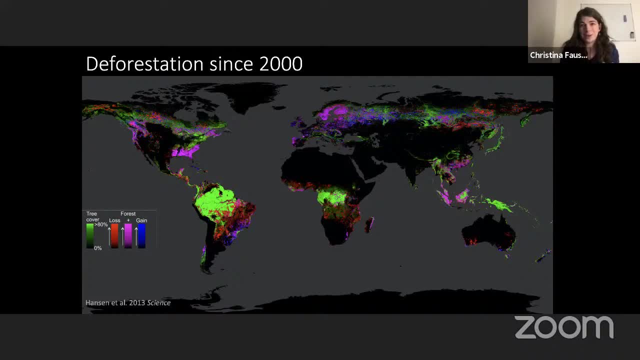 still heavily intact forest ecosystems, and in pink we have areas that have lost forest in the last few decades but also gained, and in red we have a net loss. So you can see that forest loss is occurring around the globe and it's pretty ubiquitously occurring in all ecosystems. I would 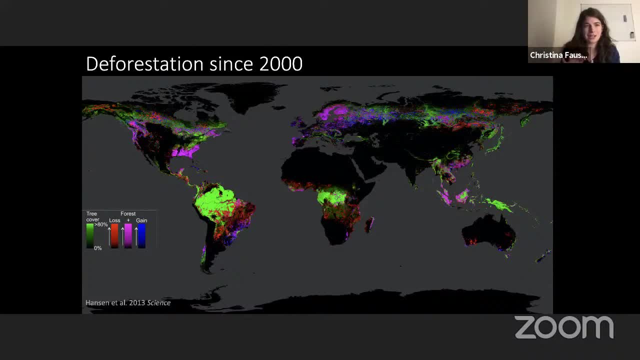 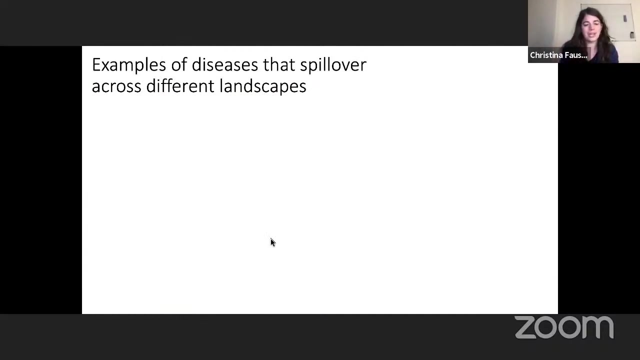 like to say that a lot of these purple areas, especially in Southeast Asia, are actually regenerating into plantations which have lower biodiversity value, and Kim will be talking about that next. So why do we care about forest cover change or land use change? We've heard many really nice examples from Dave and Rory, but I'm going to 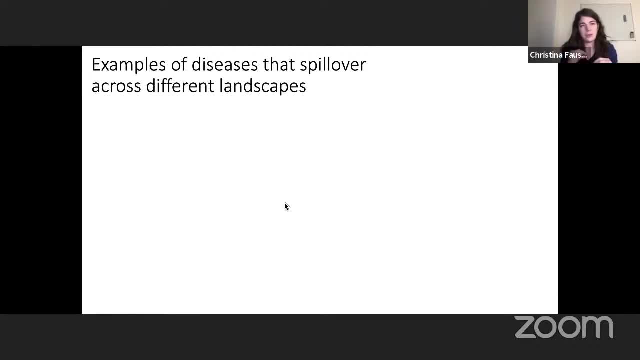 be focusing on this interface and how this land use change changes contacts between two different species. So there's been lots of examples over time about how conversion of one habitat to another can lead to spillover of new pathogens. So Ebola has already been mentioned and this often occurs. 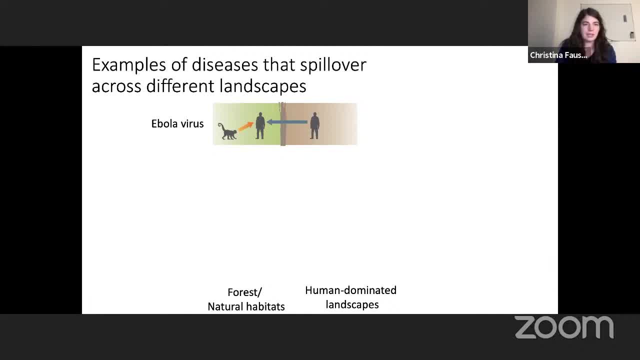 when humans move into forested ecosystems and either contact infected carcasses or harvest meat or some other contact mechanism. But we can also spread diseases to animals in natural habitats as well, and a prime example of this is humans giving measles to mountain gorillas in Central Africa, which has been recorded many times. 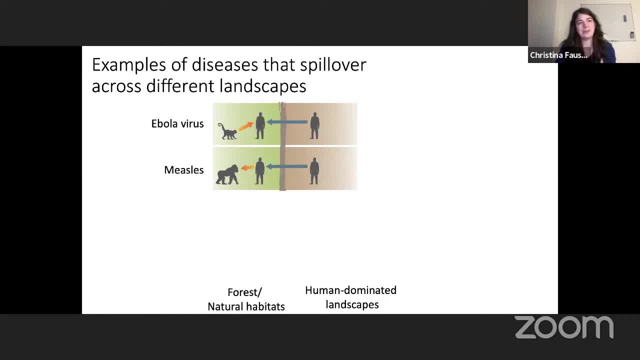 And when we think about humans converting landscapes, we not only fill those landscapes with ourselves, but domestic animals, which has been mentioned, and this has been implicated in the spillover of canine distemper virus into carnivores and Serengeti, so they get it from contact with domestic dogs in those human dominated landscapes. 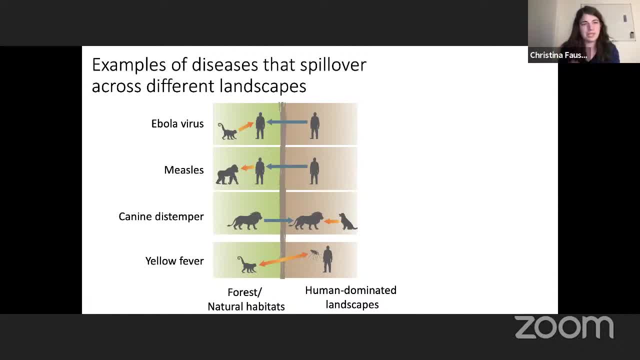 And, as Kim will talk about in a bit and was mentioned earlier with dengue, we can have mosquitoes moving pathogens across these different landscapes as well. And, as Kim will talk about in a bit and was mentioned earlier with dengue, we can have mosquitoes moving pathogens across these different landscapes as well. 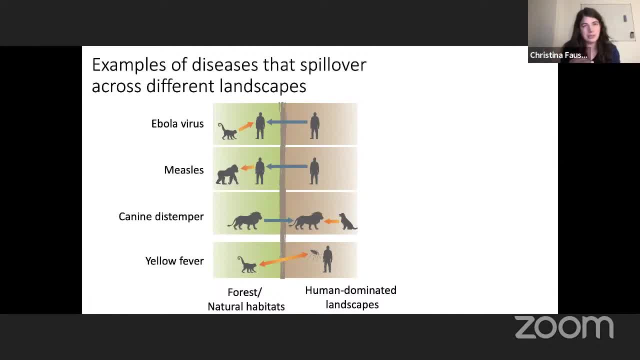 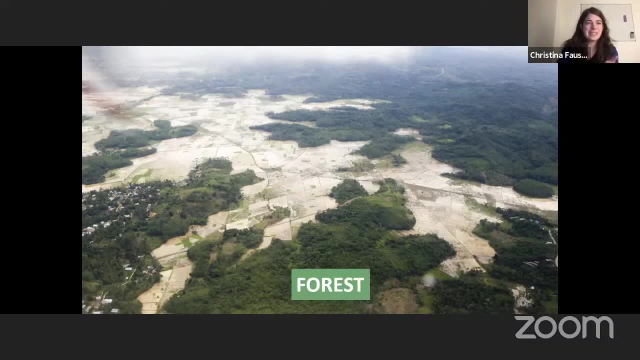 So there's lots of contact that's facilitated between these two landscapes and and disease transmission that can occur. So I'm going to go back to another aerial photo. This time we're in Ecuador, actually, And you can see that there's a forested landscape and, as Rory mentioned, these normally have really nice high levels of biodiversity and also high levels of abundance of certain species. 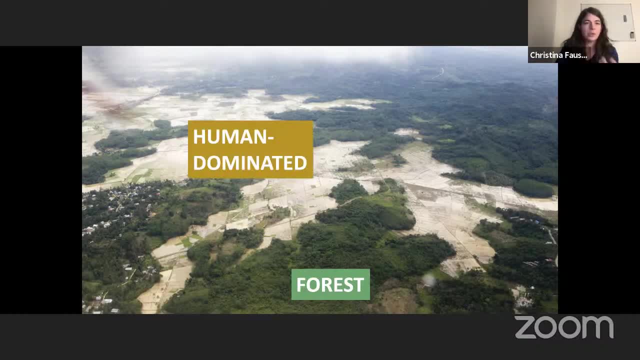 Then we also have these human dominated landscapes. Then we also have these human dominated landscapes, which are the ones that we're talking about here, which are the ones that we're talking about here. So we have a lot of these landscapes that support both human populations but also domestic animals. 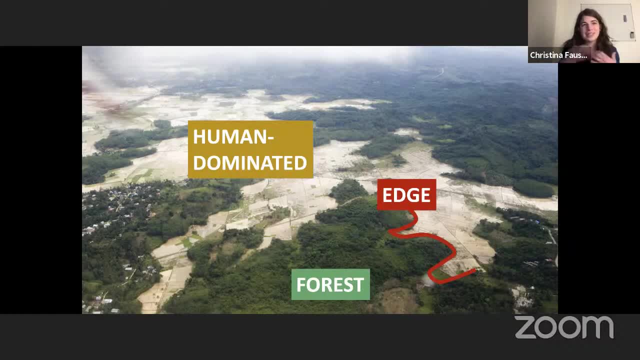 And what we've been trying to look at is this edge, So this, this interface between the human dominated landscapes and forest and what this can tell us about transmission and maybe be used as a nice proxy. And what we've been trying to look at is this edge, So this, this interface between the human dominated landscapes and forest and what this can tell us about transmission and maybe be used as a nice proxy. 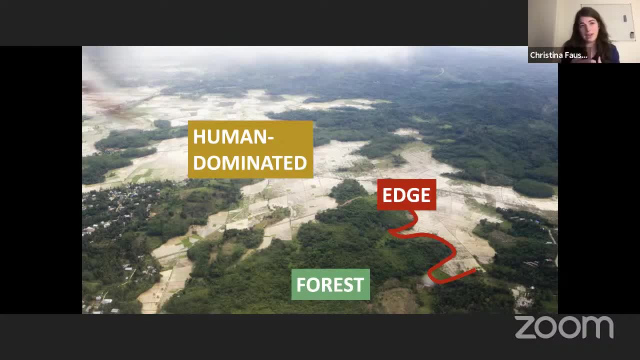 Because we can measure these edge habitats- and they're quite predictable- and how we start changing landscapes in many areas of the globe. So I'm going to show some modeling, some theoretical work, but I'll also back it up with some case studies as well. 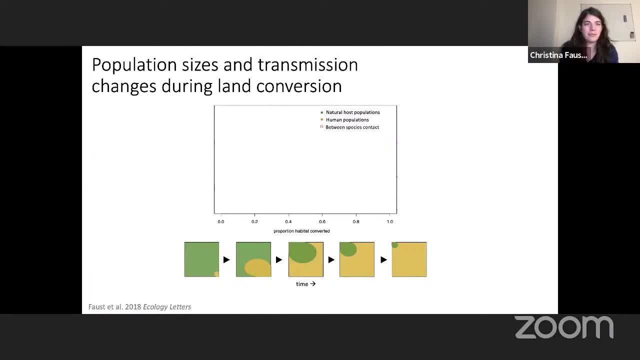 So this is just a very So, this is just a very kind of toy model that we have, but if we can think about on the bottom habitat being converted. so in all my slides, green is natural habitat and we're moving towards this tan or human dominated landscape and we think about these as not as urban habitats, but more is like a mosaic. agriculture is still supports biodiversity, but has more humans. 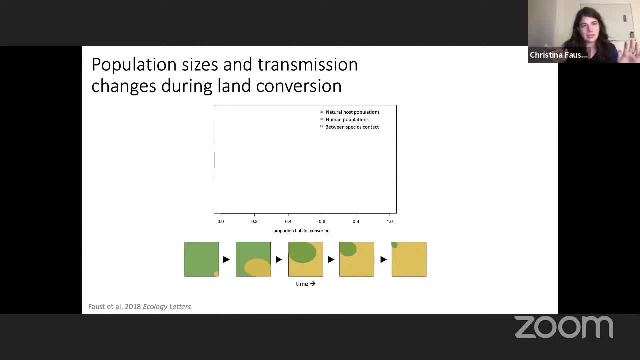 And so all of these plots along the horizontal axis will have proportion habitat converted. so on the left hand side So we have a lot more natural habitat, and the right hand side we have mostly human habitat And Currently we think about these, the amount of host or animal wildlife hosts declining as we go across this gradient. but worry, talked about examples where this is not the case. 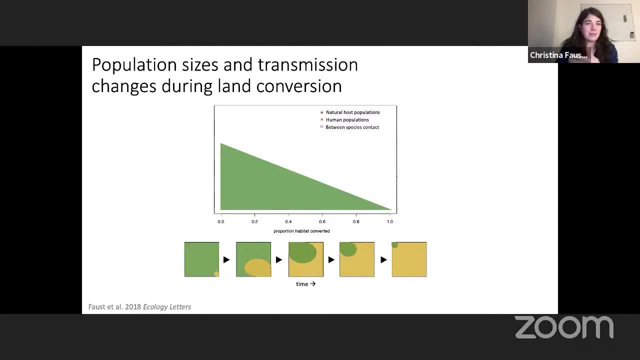 And and then, but also along this gradient, we have human population density increasing or domestic animal density increase, increasing, and this is important to think about as well as we can predict about the realities of the climate, of tenant description, of moment in time. you can see this really interesting. 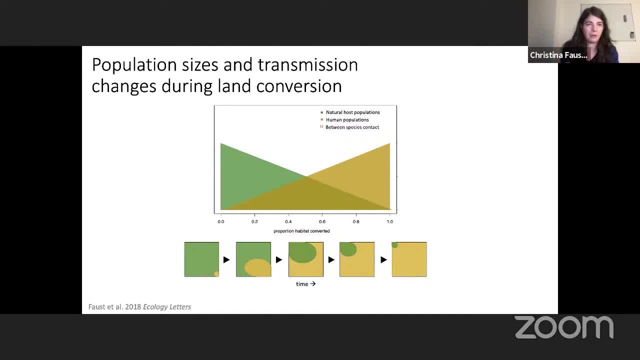 Which is which? which which convert more habitat. we have more and more people in that habitat to become infected, and both of these things are occurring on a monotonic platform, so they're only increasing or only decreasing, but interestingly, the edge or that interface between the two habitats is non-monotonic, which? 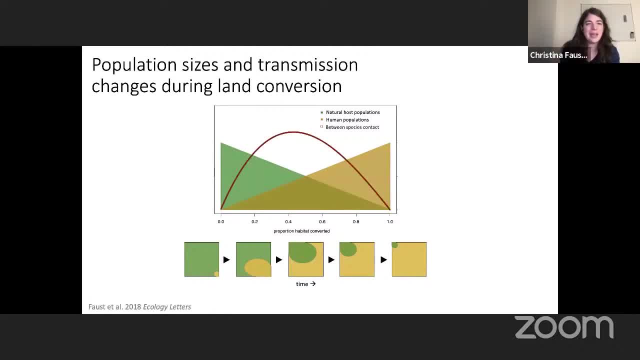 it's just a fancy word for saying it increases and then it decreases, and we think this has interesting implications for transmission. so if we think about contact between these two hosts being maximal at this intermediate level, and we can kind of simulate an epidemic in this, in this, 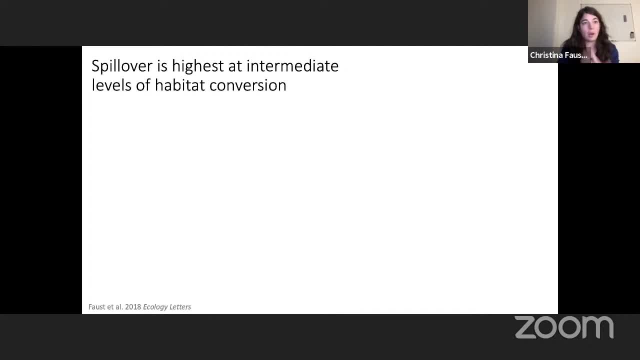 kind of imaginary world and think about when outbreaks are going to be common and so on. this plot again. the horizontal axis is the same as I've showed before, but along the vertical axis we're looking at probability of human infection. so this is thinking about: in a given year, what's the likelihood that you'll have? 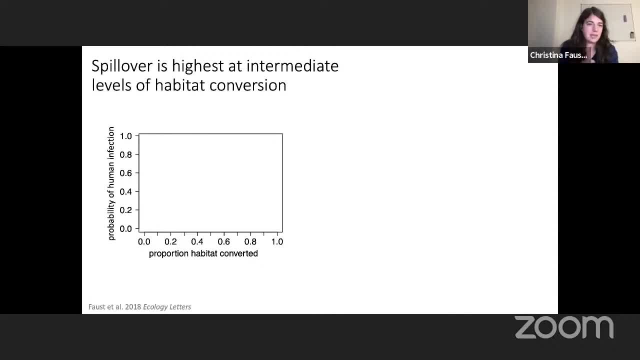 a single human infection and in this case, this. this is parameterized, so it's it's modeled to be Ebola, basically an Ugandan strain. so what we see is that, as we start converting habitat, we quickly see an increase in risk of human cases of Ebola, and then, as we move towards the edge, we actually 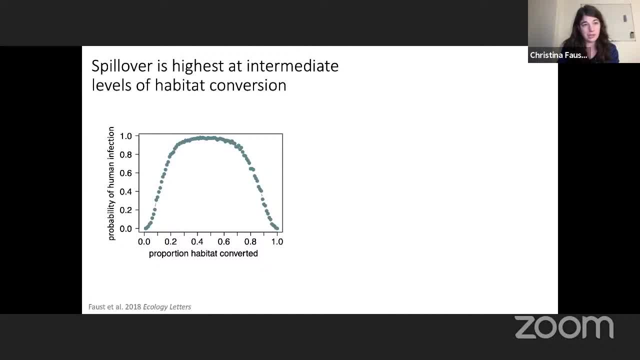 see a rapid decline, and this is because the number of hosts that are kind of reservoirs for this disease are really rapidly declining. and we can also think about, in addition to whether or not we'll get a spillover, is how big that outbreak would be. so this is: we can simulate this many 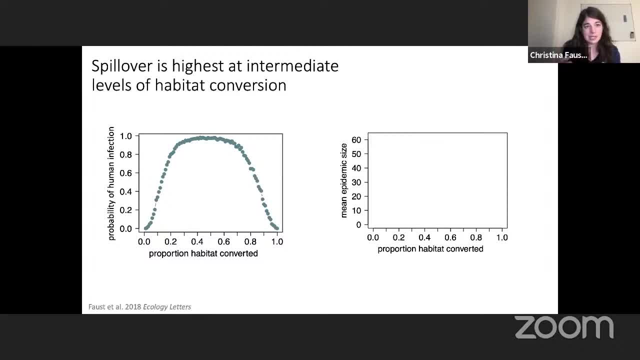 times and then measure what the outbreak size is, and what we interestingly see is that the outbreak, the highest outbreaks, are going to be the ones that are going to be the ones that are going to be the ones that are actually occurring at this lag, and and this is because the amount of humans that 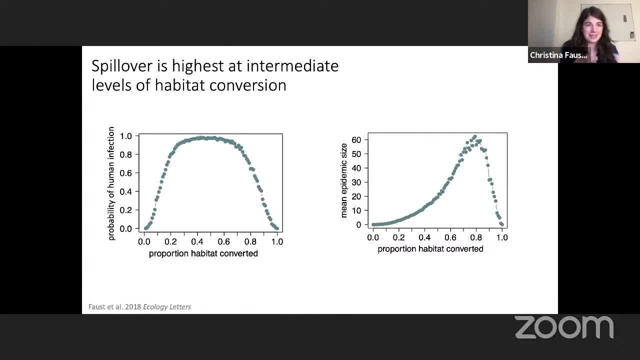 are in that habitat is much greater than in these lower habitats. so, although the the probability of an outbreak is lower, when it does occur there's a lot of human to human transmission that occurs, and why that's important is because the size of that initial outbreak is also important for the 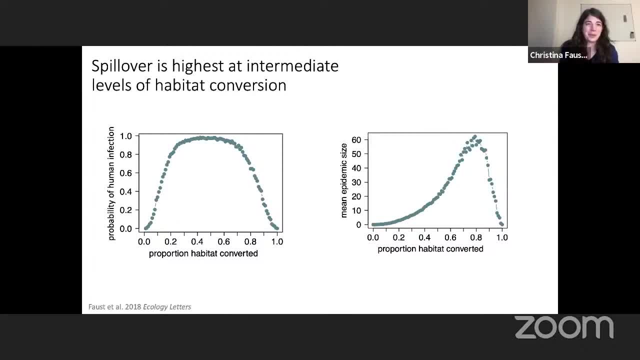 spatial spread of that disease, so so it could lead to larger outbreaks, like the West African outbreak in 2016. so both of these things are important to think about, and this is an example that's just using a slice of kind of across space, but we can vary. how much is deforested each year? 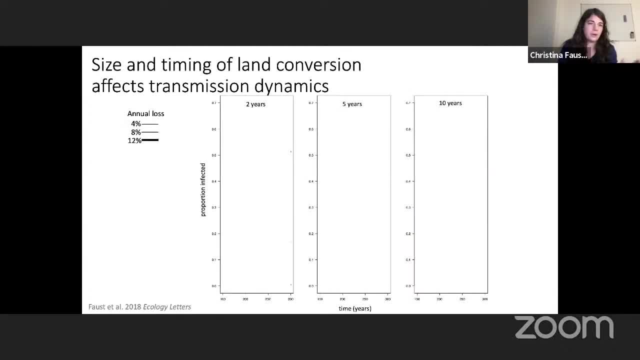 how much land is converted each year and and how that changes through time. so so these different plots are showing different amounts of conversion, and then the thickness of the line is how much land is converted in that one instance. and again, green here is our animal population or non-human animal population, and and brown is the 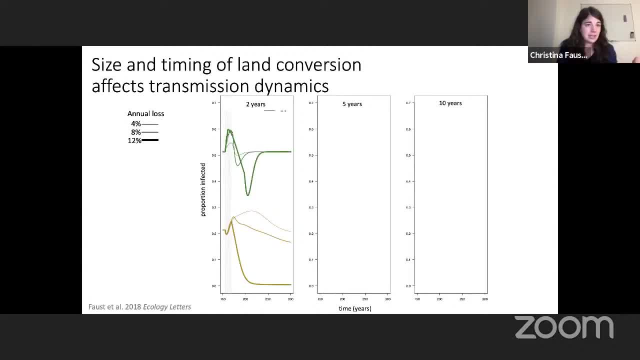 human population and what we see is, once we start seeing conversion, we see actually an increase in prevalence over time. this actually does dip down in some of the different conversion regimes over time. I'd be happy to talk about why that is, but this is just to emphasize that the size and the 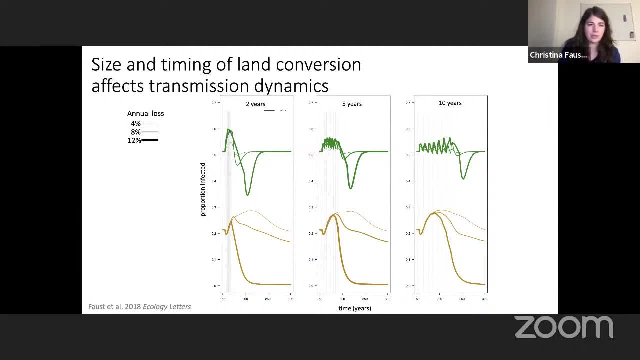 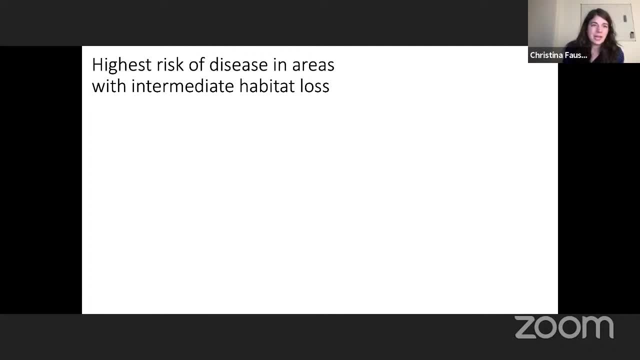 timing of conversion and the size and the timing of conversion and the size and the timing of conversion is also important for spillover dynamics. so these are all models, is this true? so there's several examples we have where disease systems or human risk is actually highest at intermediate level of 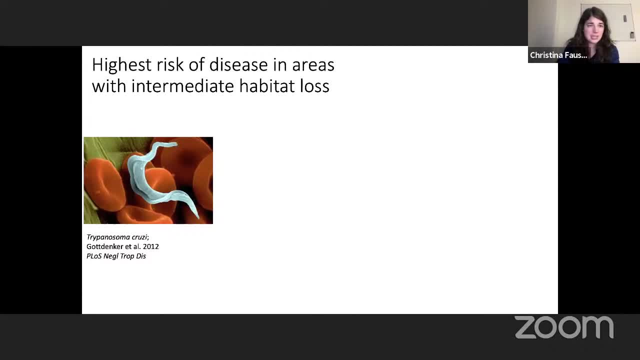 conversion. one example is shockus disease, which is caused by a trypanosome parasite, trypanosome crucii, and this occurs throughout Central and South America and there's some really nice examples of where you get highest human risk is actually at these habitats that are marginally converted, and 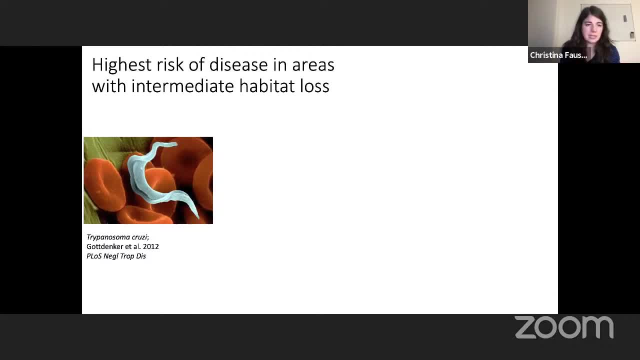 close to some very extensive forested areas. borreli ulcer is this mycobacterium. it's transmitted by water bugs and stream systems and they also find that intermediate levels of conversion. so you still have to have certain members in the habitat present. we do get highest. 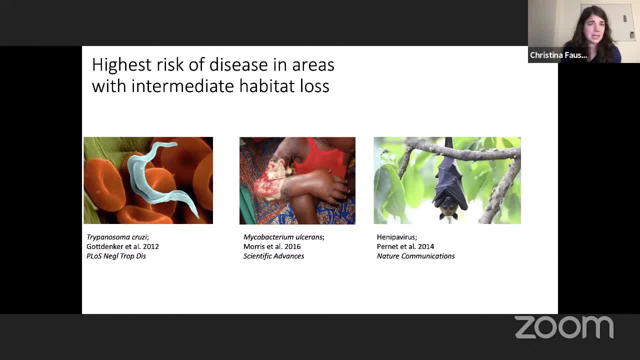 infection risk to humans. and then another example, which were probably these are flying foxes, so bats carrying Hennepa viruses. so this is in Central Africa that they found. humans that lived in villages that had recently deforested a bit around their village had the highest. 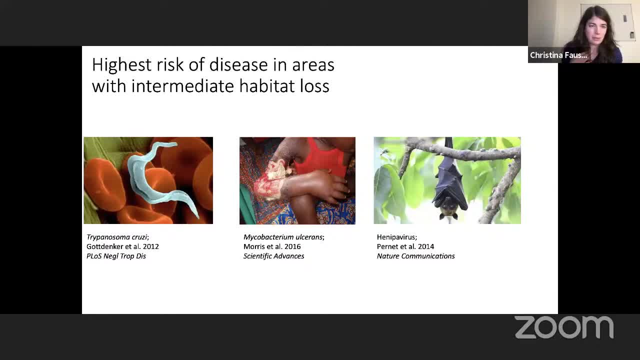 prevalence of serology for Hennepa viruses, which suggested they had higher exposure rates, and Kim will talk about some more exciting examples next. and when I give this talk I often have to caution people that converting all the habitat is not the solution. So Hendra virus has a really nice example. 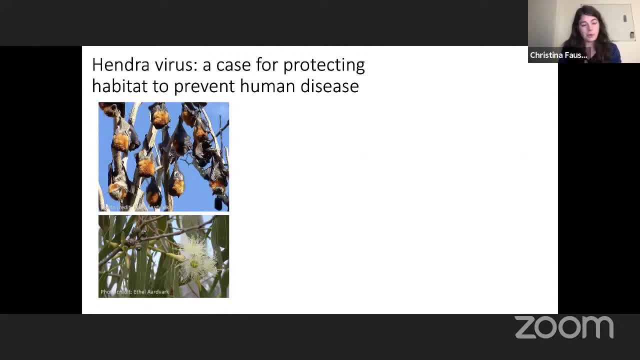 So Hendra virus is a bat virus that normally or a virus that normally circulates in bats in Eastern Australia And these bats feed mostly on nectar and pollen from eucalypt species That's down below, that's a eucalypt flowering event. However, the last century has led to massive loss of their own eucalypt habitat, And these bats have actually moved into urban areas. So they reside in camps or large roosts in urban areas and feed off of invasive species and also backyard fruit trees. 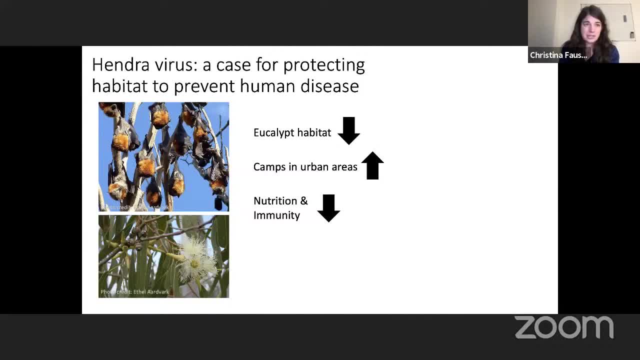 which decreases their nutrition and immunity and actually increases their likelihood of shedding virus, which we think in turn has led to the increase in human cases that we've seen over the last 20 years. So this is just a map of Eastern Australia, and the bats actually occur across Eastern Australia. 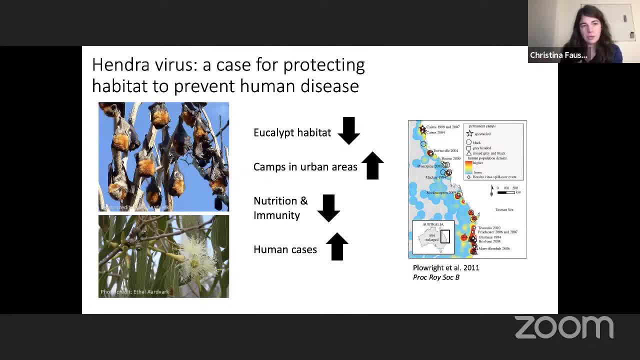 And the highest amount of bats is actually away from human habitats. but in white we can see the spillover events and these are concentrated in human centric areas. And it has to go through a horse horse. There's some complications about it. 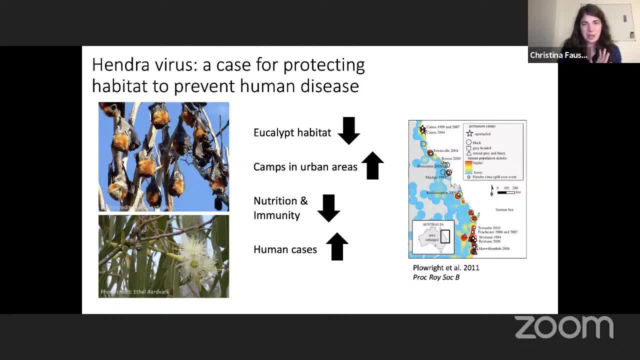 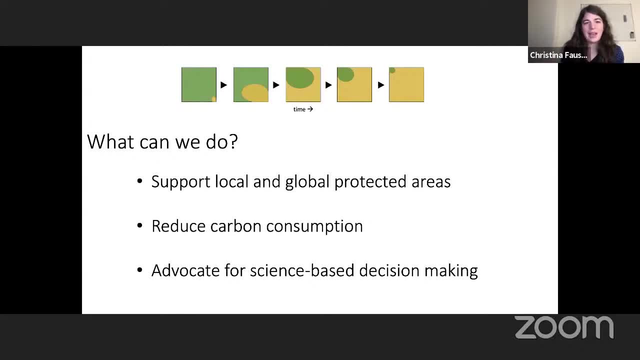 but I'd be happy to talk about it later, So I don't want to end on a bad note. There's many things we can do to kind of promote this one health approach and these protected areas we think are incredibly essential for maintaining biodiversity and high quality habitat. 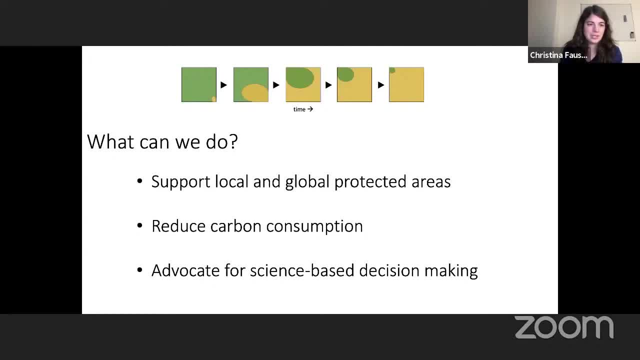 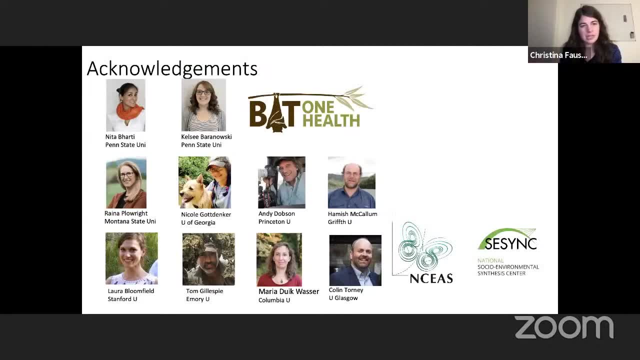 and reducing carbon consumption, So we can reduce land use change and also advocate for kind of science-based decision-making which some people have brought up, And with that there's many people to thank. And if you're interested in bat one health or this kind of Hendra virus, 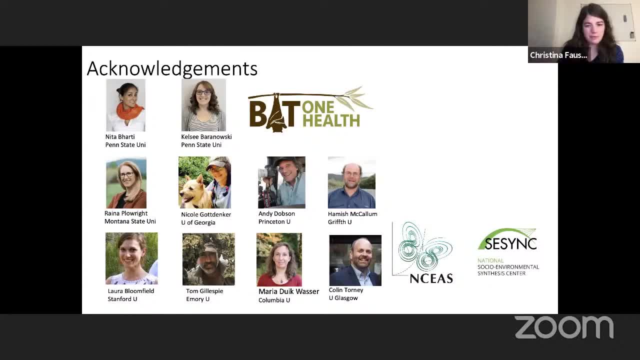 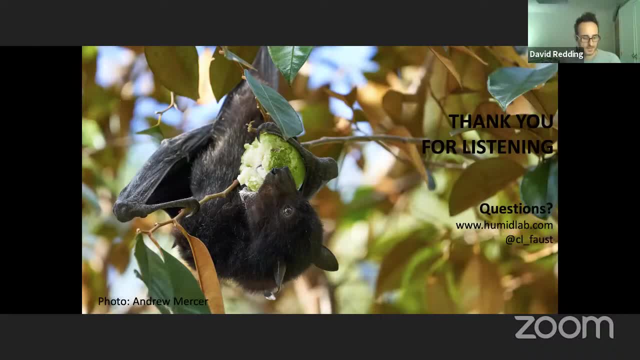 you can check out their website And there's many people that have been involved over the years with this, So thank you for listening. Thanks, Christina. That was a brilliant talk of one of my favorite papers of recent time, I have to say. 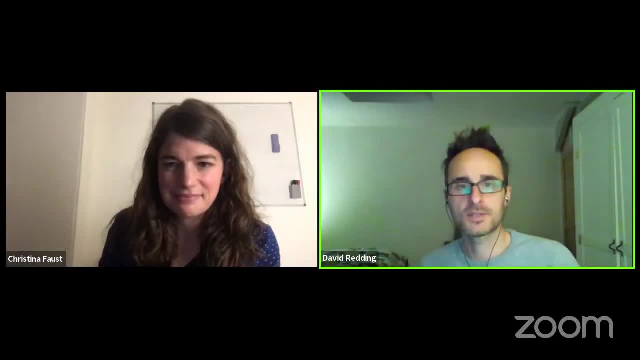 So okay. So just having a look at some of the questions that are coming in, Some of the things that I was interested in was- I don't know whether it's that easy to answer as a question, but I was thinking about whether there's kind of 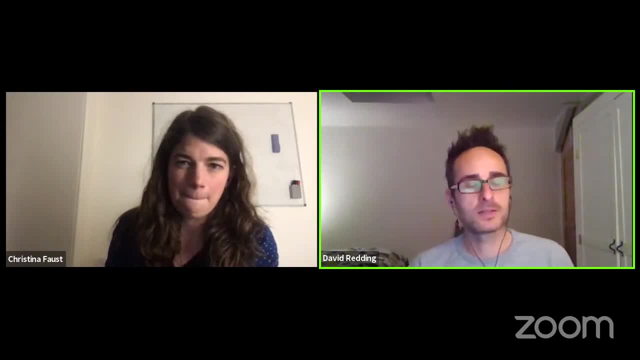 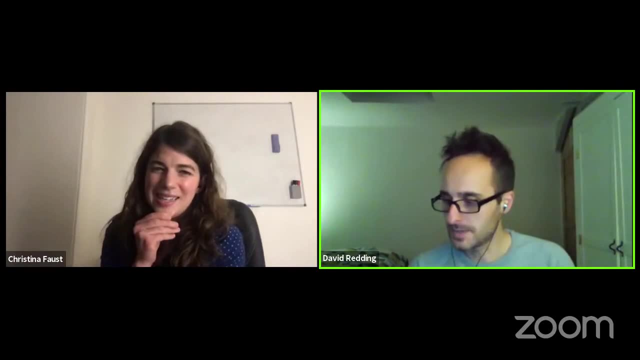 different pathogens that might be being passed on at different levels of conversion, whether there's kind of characteristics. So I'm kind of thinking that in areas that have been converted for quite a long time we may be looking at kind of endemic or chronic sort of diseases. 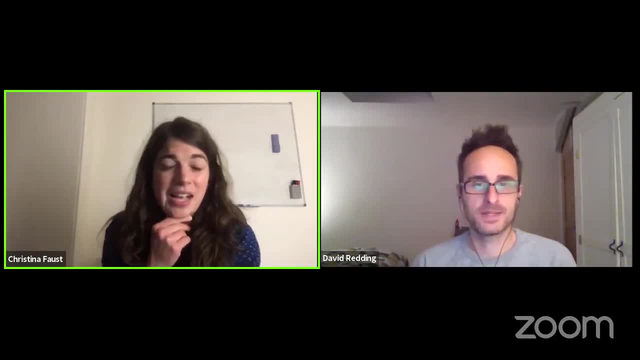 I don't know whether you've sort of thought about that, Yeah, So I think it's gonna heavily depend on kind of, yeah, the lifespan of the pathogen, If it's a chronic infection- Yeah, infection, so this is a pathogen that's always going to be in reservoir host species- and whether 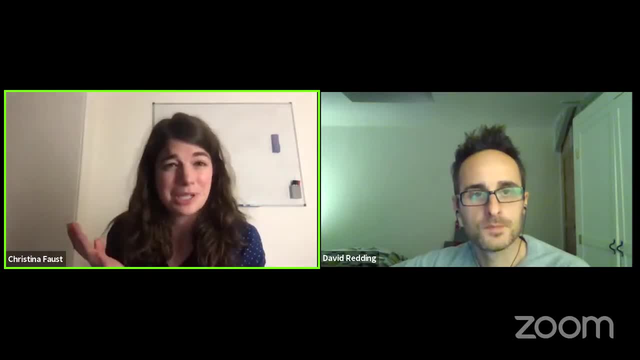 it can have an environmental stage so. so a lot of these nematodes or parasitic worms that we have can actually have a stable environmental stage so we can have time lags. so when you convert a landscape rapidly you might have kind of a bolster of a reservoir host. that's actually putting out. 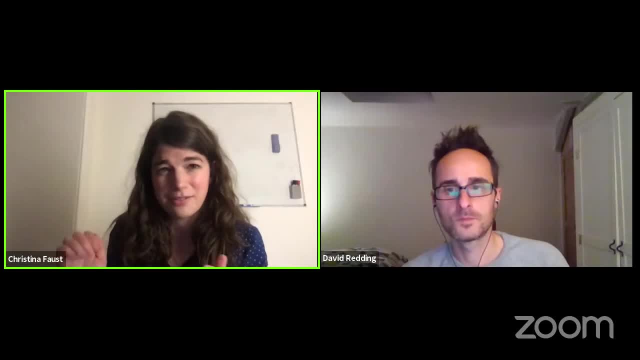 lots of parasites and then you could have a carry-on effect. i think i'm going to go with rory and that a lot of these are going to be context dependent, but i do think there's a lot to learn about parasite life histories and and and what's needed. um, how long their generation? 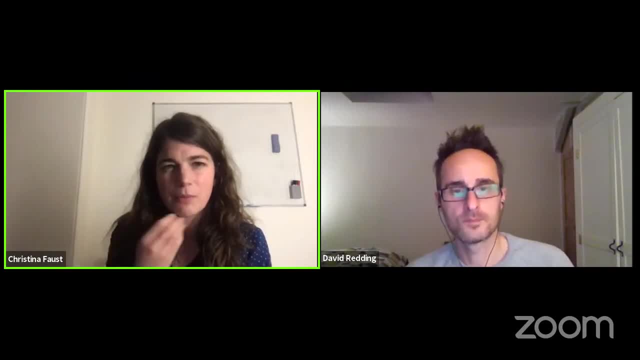 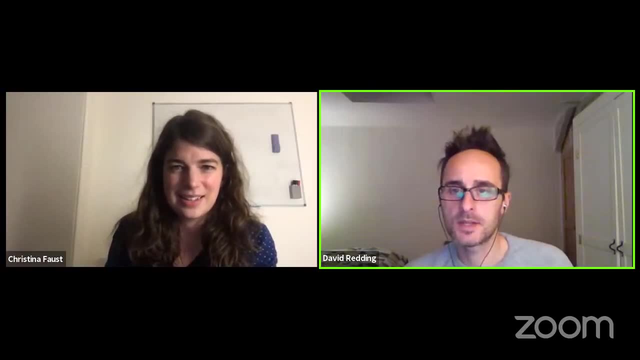 times are and how stable they are in the environment, to be able to inform a little bit more of this temporal and spatial variation. so yeah, um. so a question that's come in, um, but i guess you sort of sort of uh is is what you've been talking about is um, how do we counter keeping 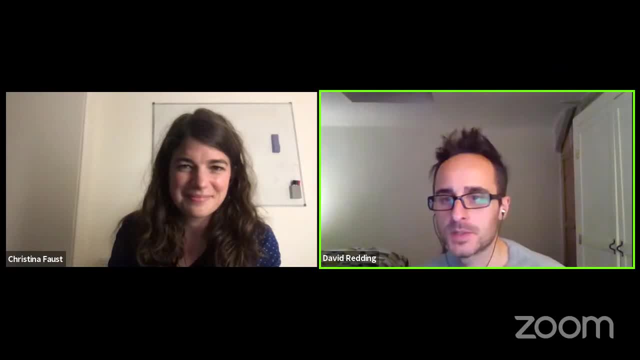 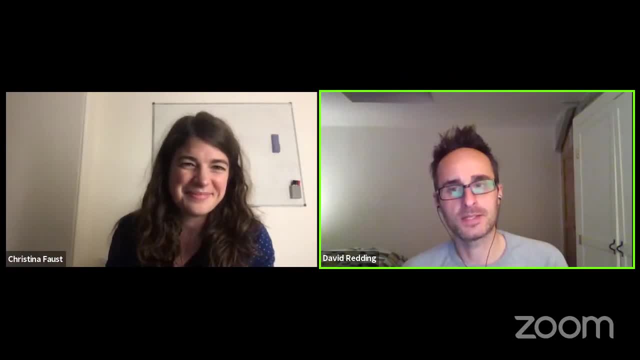 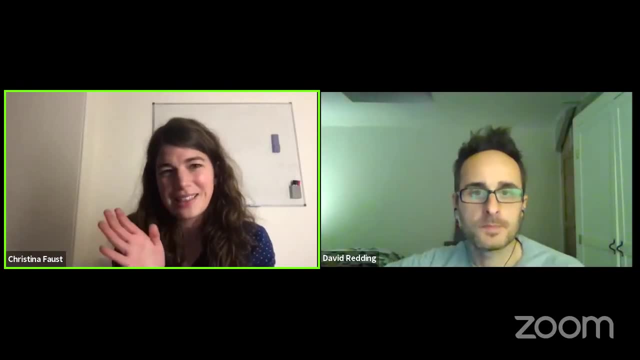 kind of thinking, i guess, how, how is fragmentation, how do we manage fragmentation and that sort of thing? yeah, i think well, there's kind of two sides of the coin, right in that some hosts thrive in in natural environments but, as rory mentioned, some hosts thrive in urban environments and i there. 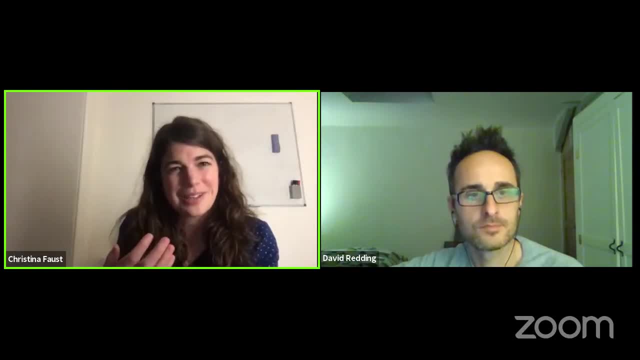 is a move to kind of um manage hosts in a way that that we can improve their health. there's transmissible vaccines that we have for vampire bat rabies that we can employ, so there's treatment options for hosts and learning to kind of how to manage pathogens within those host populations. but i think for a lot of. 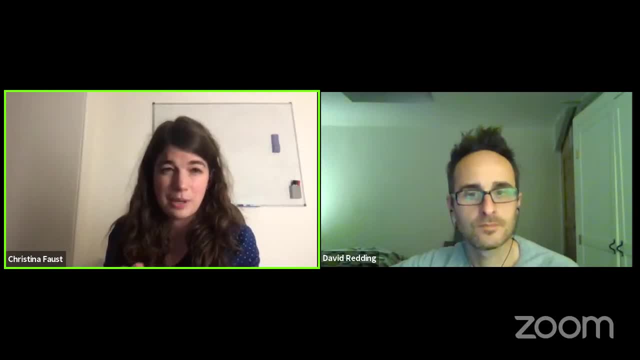 diseases. we don't yet have the full toolkit to be able to help manage disease within the host. we do know that healthy host is better for our health as well, um, so that improving immune systems in hosts can also have knockdown effects for us. but yeah, it's. 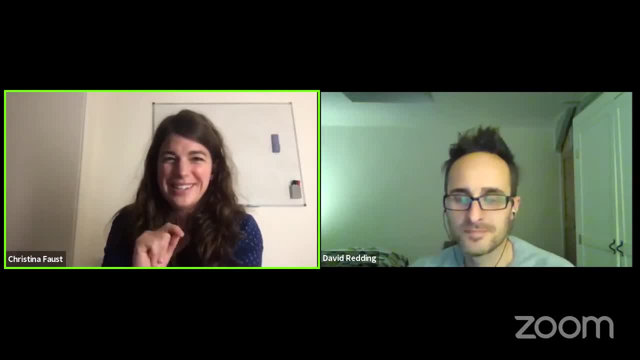 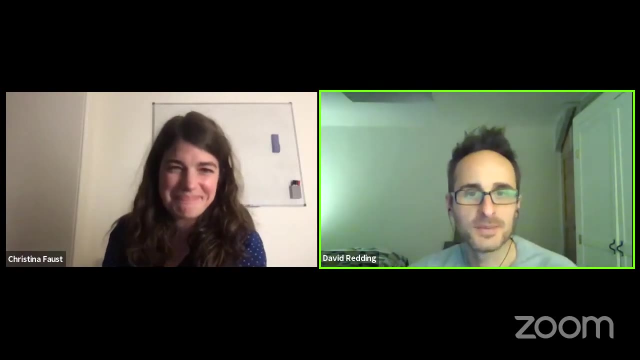 yeah, i don't think that answered the question completely, but i think if you ask anyone that's tried to control any rodents, um, in an urban setting it's nearly impossible, um. so, yeah, certainly it's, um definitely you're left with some very difficult to control animals, i think. 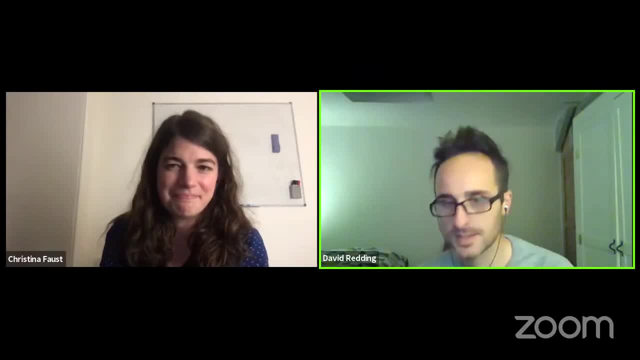 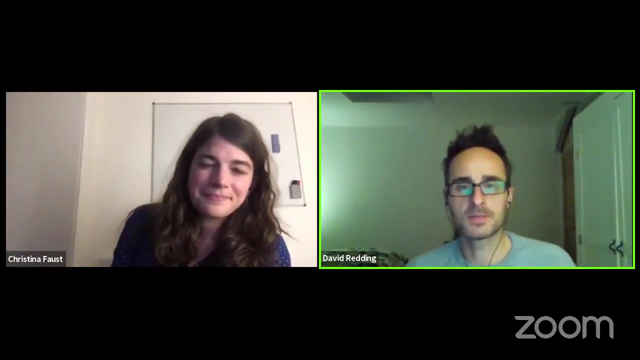 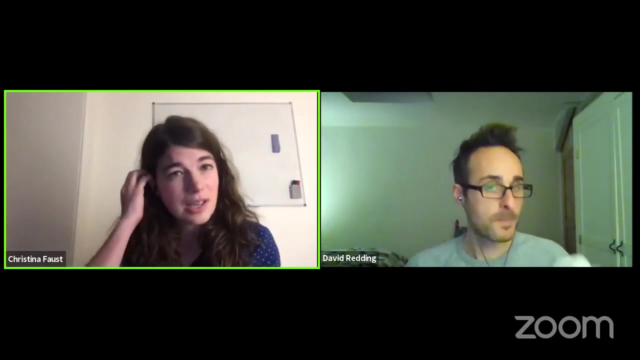 as you develop the landscape into sort of more human dominated landscapes. okay, just have a quick look. um, i said i guess this kind of question also really has just been answered. but should we then target active management against certain species that increase risk? yeah, so i think, especially so in eastern australia with with bats, the, the target is actually now to 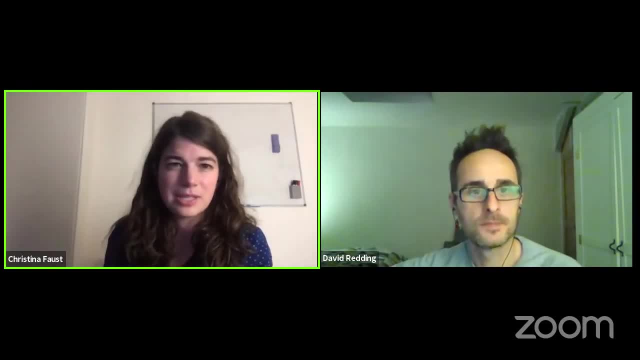 restore their natural habitat and draw them out of these urban centers so they're adaptable and they're able to move around and they're able to move around and they're able to move around and they can move into urban centers, but it's not ideal for both site, both humans and the animals. 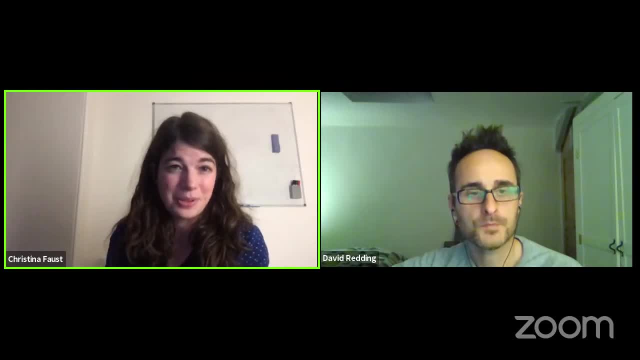 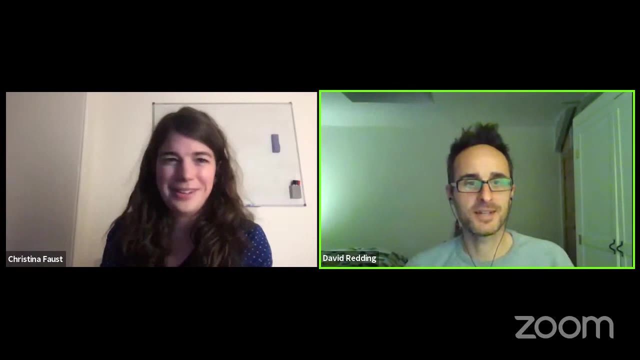 so active restoration is actually probably the best tool they have to control, manage that that particular host. so i think it is an option as we learn more and more, um, but it will definitely depend on the disease system. yeah, i don't quite know how, what we do with black rats, really, and 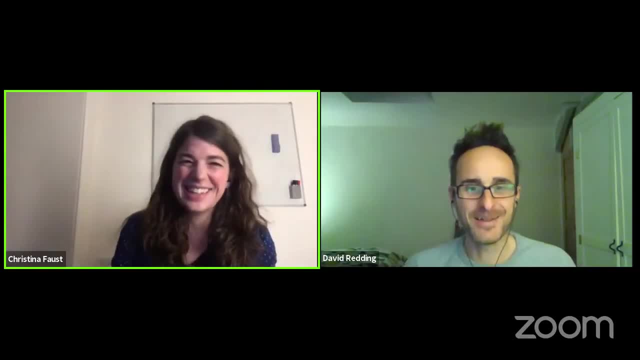 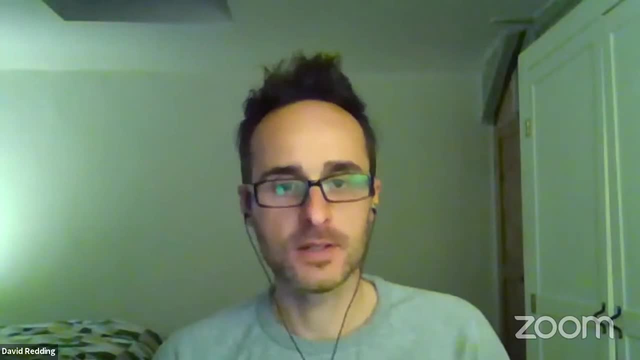 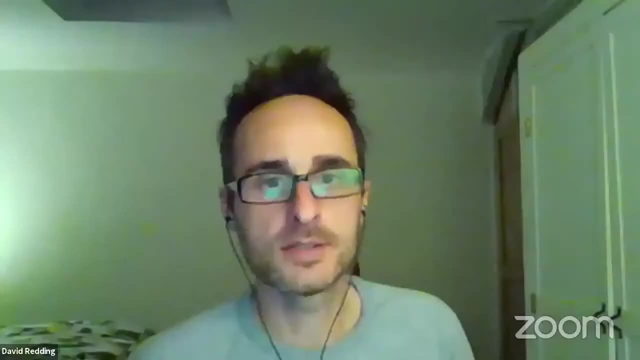 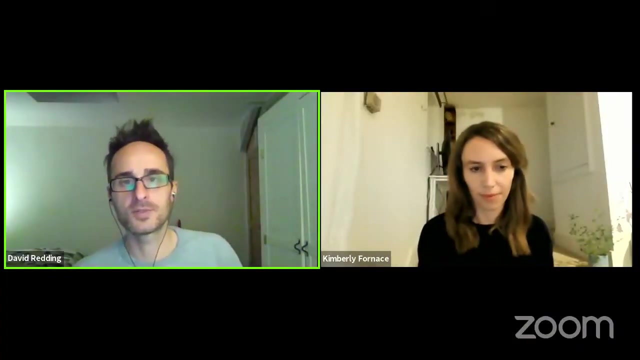 how we draw them back to wherever they came from. but, um, okay, well, thanks very much, christina. that was great talk, um, so so our next speaker is dr kimberly fornace um, who is an assistant professor of at uh, the london school of hygiene and tropical medicine, which, i've said correctly, at this time her work is: 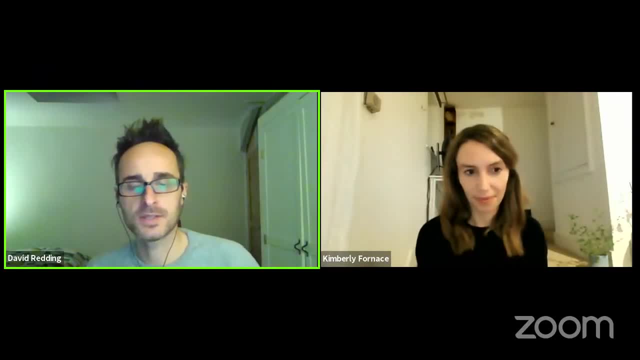 mainly looks at the effects of landscapes on infectious diseases, and some of her work, i think is- is kind of what it's um some of the things that i was trying to allude to, of how we can kind of think more holistically and and think in a kind of working in a multi-disciplinary way. so it's um very exciting to. 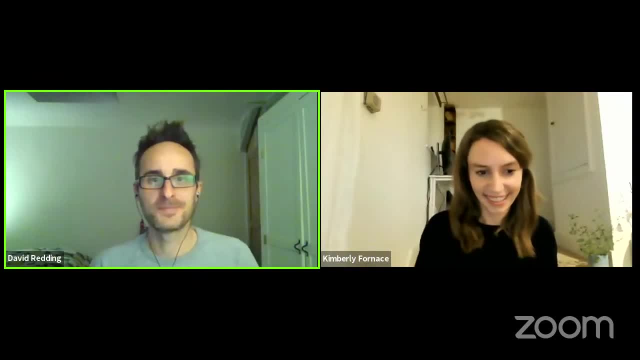 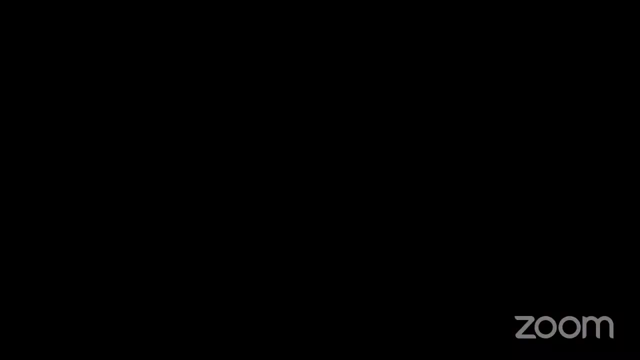 hear what she's been doing over to you. great, thank you so much and so right. so just um while i'm waiting for my screen to share. so i'm going to take a little bit of a different take um from everyone else and i'm going to take a little bit of a different take on the. 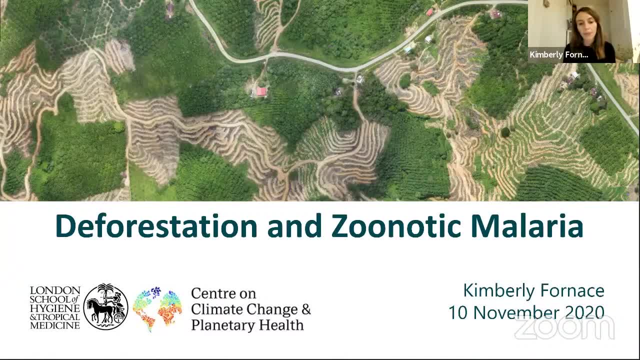 um from everyone else and i'm going to take a little bit of a different take um from everyone else and i'm going to talk about a very specific research project. um, so, this was the monkey bar research project, which was a collaboration between asia, the philippines, the uk and australia, which was really looking at this. 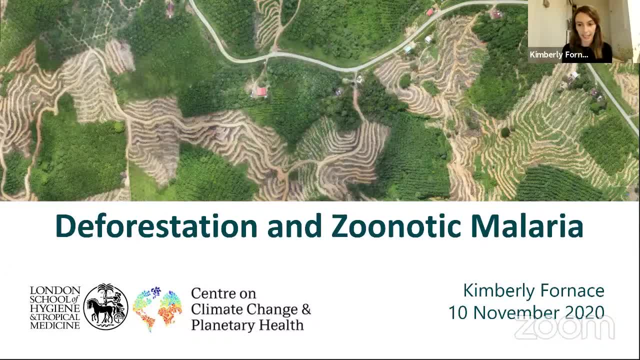 relationship between deforestation and zoonotic malaria in asia. right? so just as a bit of background, this is looking at plasmodium nolsi. um. so plasmodium nolsi is a malaria parasite which is typically carried um. so plasmodium nolsi is a malaria parasite which is typically carried. 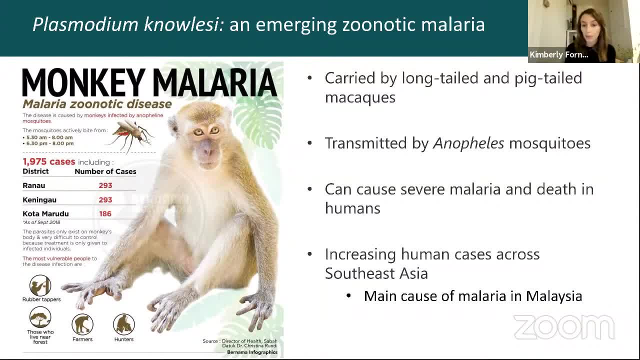 by long-tailed and pigtailed macaques. by long-tailed and pigtailed macaques, like all human malarias, this is transmitted by anopheles mosquitoes, so human cases of plasmodium nolsi occur when a mosquito bites an infected macaque and then goes on. 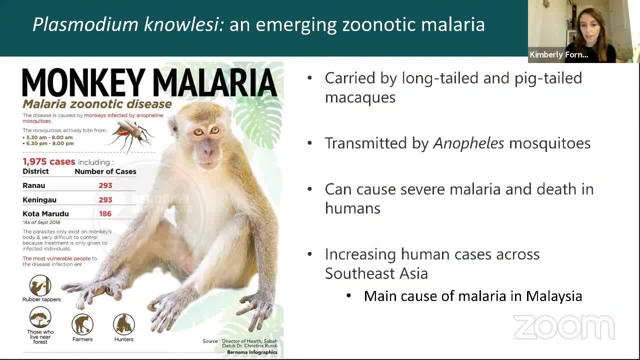 bite a person, and this is an important public health issue. so this can cause severe malaria and death in people. and what's a particular concern is there's increasing numbers of human cases which are reported across southeast asia, so plasmodium nolsi is now the main cause of malaria. 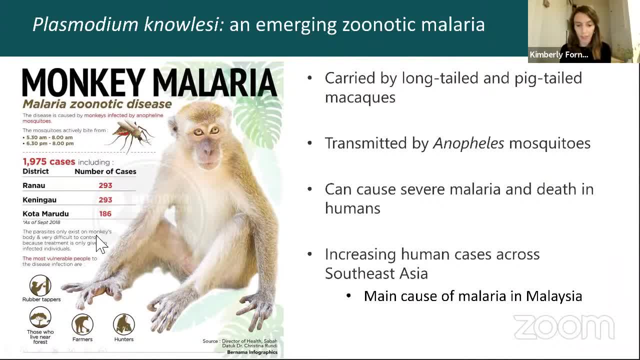 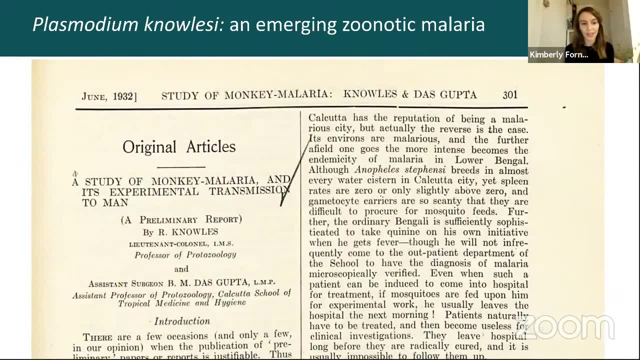 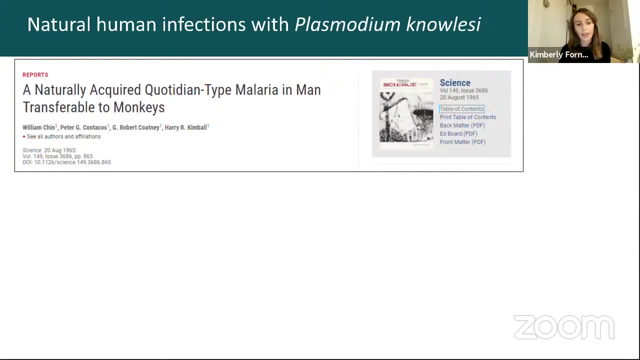 in malaysia, um, and there's several thousand cases reported every year, and so, while this is an emerging disease, this is not a new disease. nolsi was first discovered in 1932 in macaques, and the very first naturally acquired human case of nolsi was identified in 1965 in a person, and but there was very little evidence. 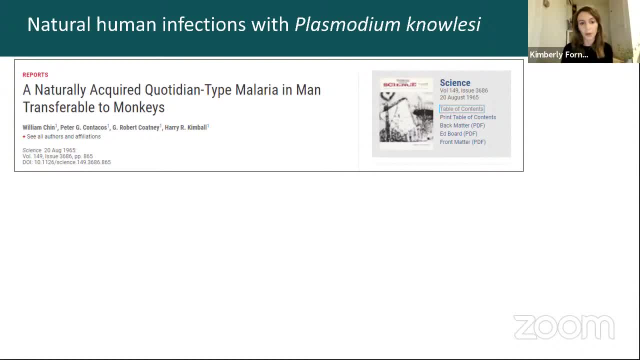 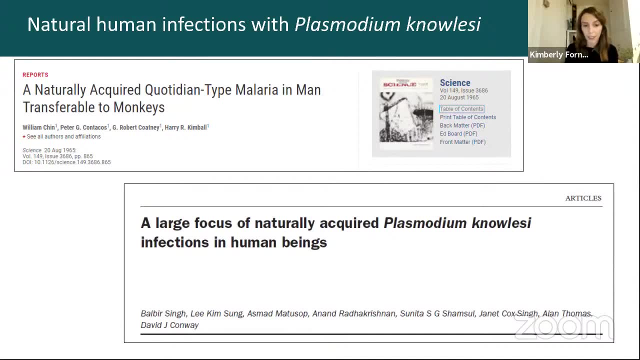 that this was actually a substantial public health issue, and so no other human cases were reported until 2004.. and in 2004, colleagues working in malaysia and borneo used improved diagnostics to show that a large number of human malaria cases were in fact plasmodium nolsi. 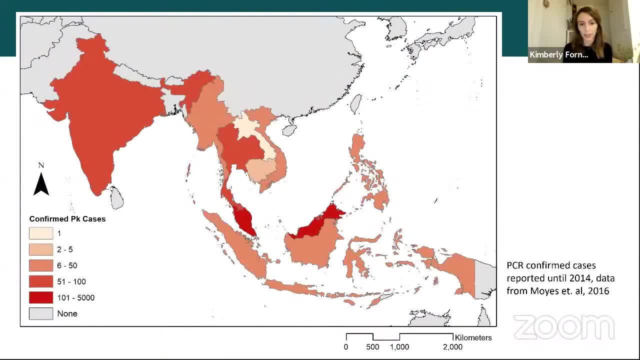 and since 2004, plasmodium nolsi has been reported all across southeast asia. so there's quite a wide distribution and these numbers have increased substantially since this map was made. but i think what's quite notable is, despite this wide geographic spread, there's 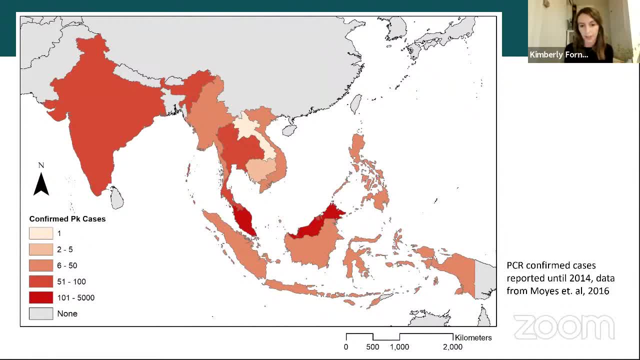 substantial differences in the numbers of cases reported in different locations. so malaysia has the highest number of plasmodium nolsi cases reported in the world and the particular focus of this is in this island of borneo. so if we overlay this map- deforestation- what is immediately obvious is that these areas that have some of the highest rates of 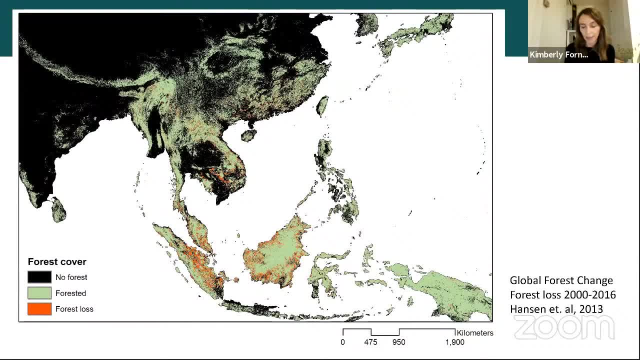 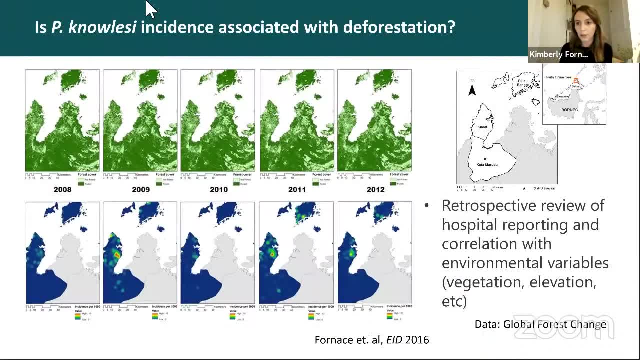 deforestation also are reporting some of the highest rates of plasmodium nolsi. so when we started this project, one of the first things we wanted to do was to look at the relationship between forest cover and plasmodium nolsi incidence, and one of the questions we wanted to to answer is: 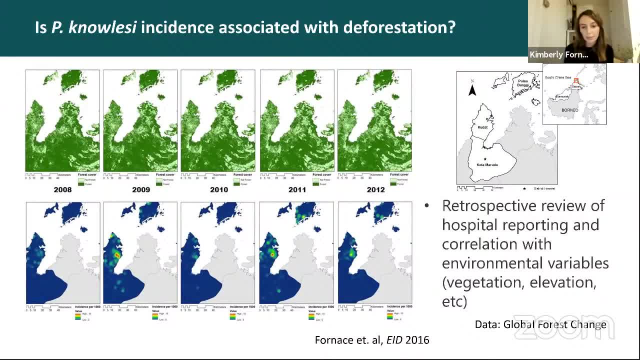 nolsi incidence associated with deforestation, or is this really, you know, effective? now that we know nolsi is here, the more we look at it, the more we actually find it, and so, to do this, we did a retrospective review of hospital-based reports and fit some models to 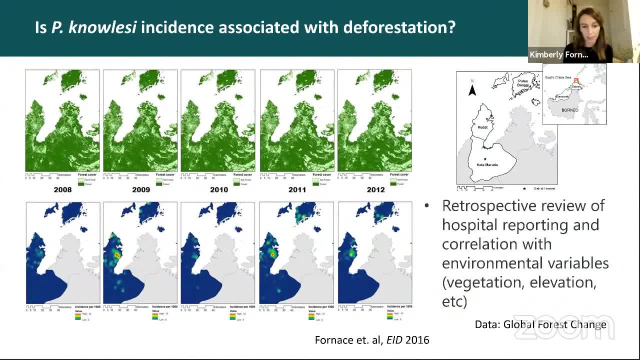 to estimate village-level null-zye incidence, adjusting for some of these issues around reporting and diagnostic sensitivity. We then integrated this with a number of different environmental variables, looking at deforestation, forest cover and other metrics, And what we find is the answer is yes. 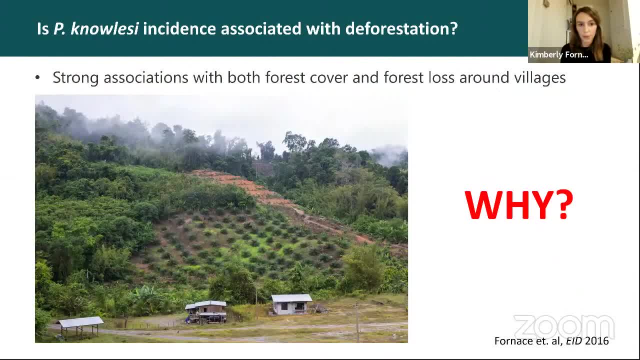 There is a very strong association between plasmodium null-zye and deforestation. So these villages, which are reporting some of the highest numbers of plasmodium null-zye cases, are areas where there's ongoing deforestation. 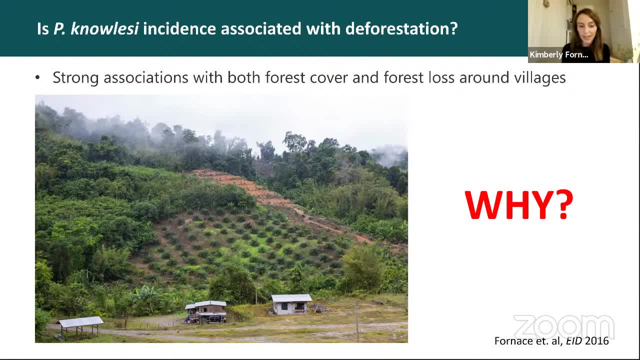 But notably, as Christina's already explained, these are areas that are not just deforested, but these are areas that have both forest cover and forest loss, so these very patchy, fragmented landscapes. The next question we really tried to answer is why. 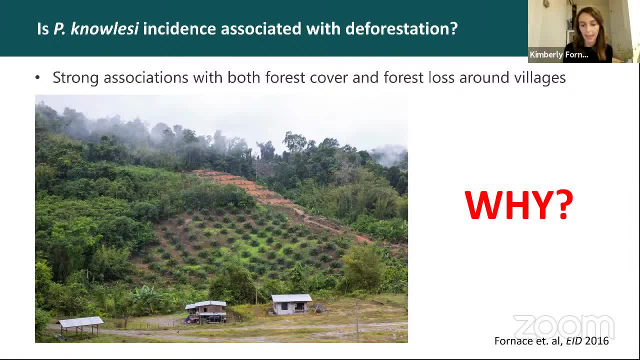 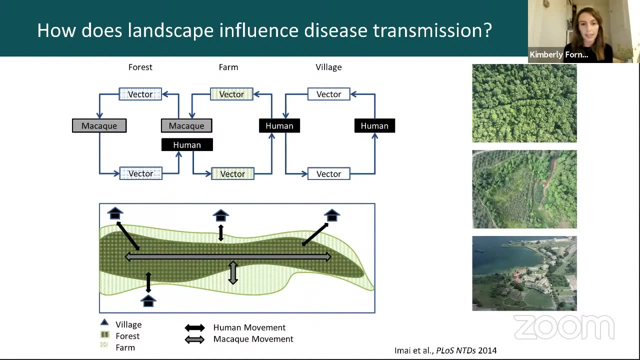 So what are the mechanisms that underlie why these particular landscapes are associated with risk? And so, if we think about this really quite simplistically, thinking about these different populations that are implicated in plasmodium null-zye transmission, we know that we have people that are living in villages. 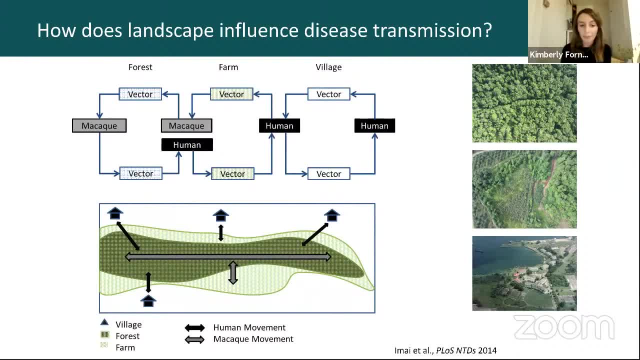 and moving into farms and forest landscapes. We know we have macaques that are living in forests, moving into farms and often into villages, And we have different numbers and densities of mosquito vector species which are living across all of these different habitats. 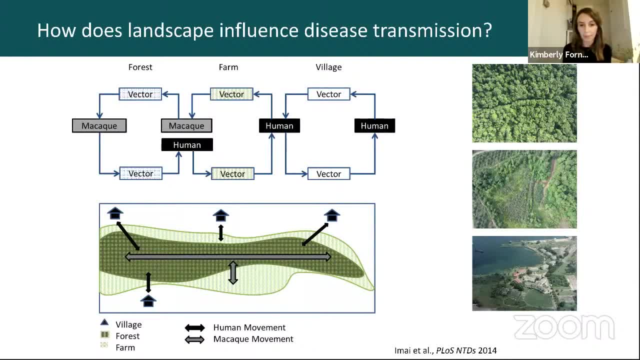 So we hypothesized that deforestation was really driving these, was driving plasmodium null-zye incidents by increasing the proximity of these different populations, So really bringing these populations that were previously separated together. And so one of the first steps to actually 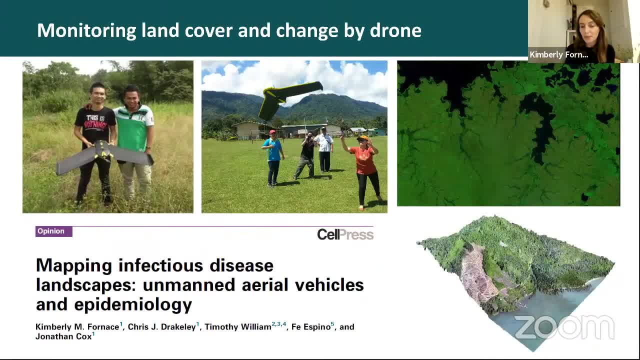 is looking at where deforestation is occurring. So I think we've already seen some very nice examples of using satellite data and we used a number of different sources of satellite data to monitor deforestation and landscape But as well, in addition to looking at satellite data, 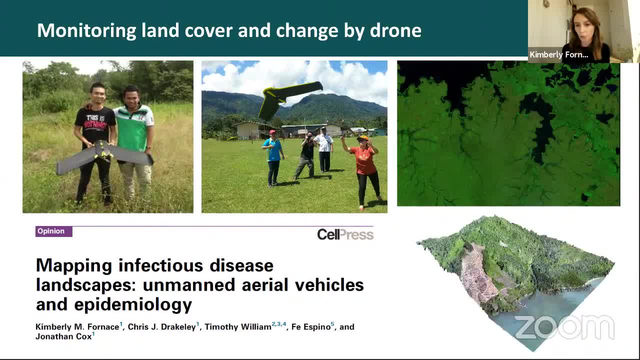 which can detect landscape changes over much wider spatial scales. we also used a drone to look at very fine scale spatial patterns of deforestation, And so this is just an example of our drone flying in Malaysian Borneo. And why this is really useful is this allows us to collect 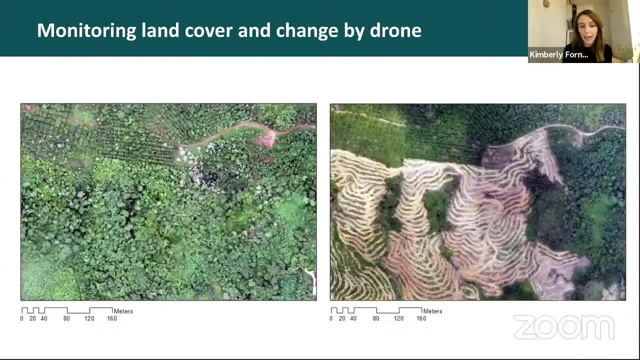 this very, very detailed data on land cover and actually map deforestation as it's happening, And so this is an example of the same site in Malaysia, but only several weeks apart, And this is an. this is an incident where we were. 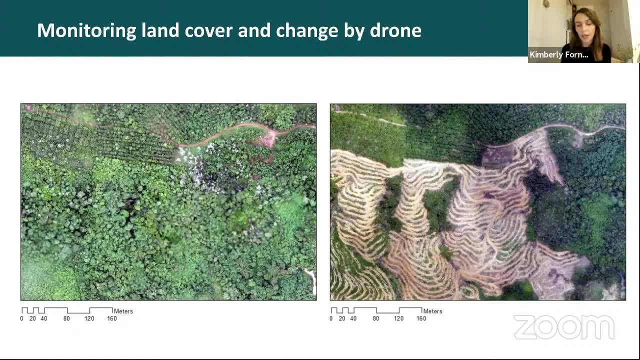 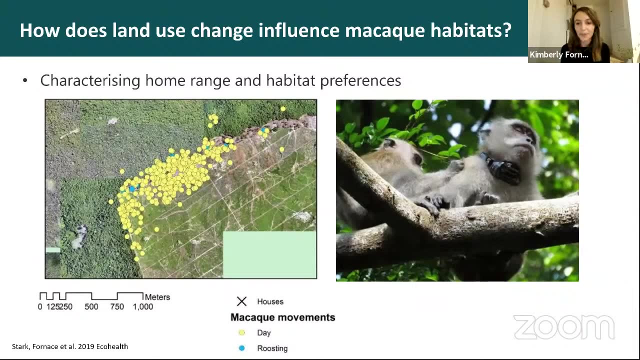 we were able to actually map deforestation as it was ongoing, So to capture this clearing while it was happening and look at how this impacts all these different populations. The next step: really thinking about these populations and how do they fit within these landscapes. So of course, we needed to look at macaques. 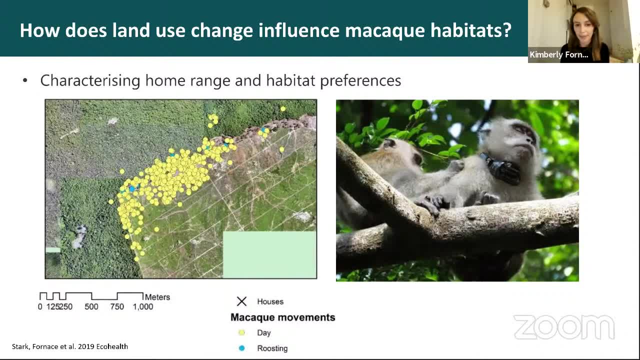 and to understand how macaques are using these different types of landscapes, And so, to do this, we GPS collared a number of macaque troops and this is collecting data on the locations that macaques are moving into, So we're able to look at how they're using. 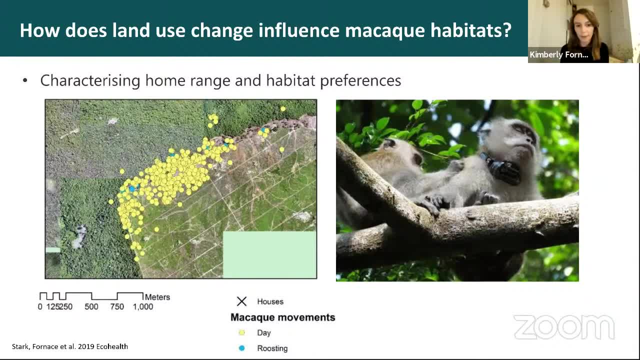 these different landscapes, how far they're moving and how these movement patterns change in response to deforestation. Well, of course, in our ideal world, we would like to GPS collar every single macaque in Borneo. we obviously can't, So we also looked at a number of other ways. 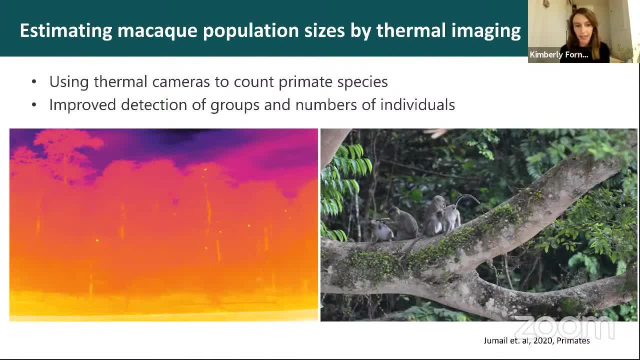 we can estimate wildlife populations, list and based basely and from a distance. So this is another example of using thermal cameras. So this is thermal imagery that detects heat signatures And we use this to identify rapid estimates of macaque populations, And so both of these images below. 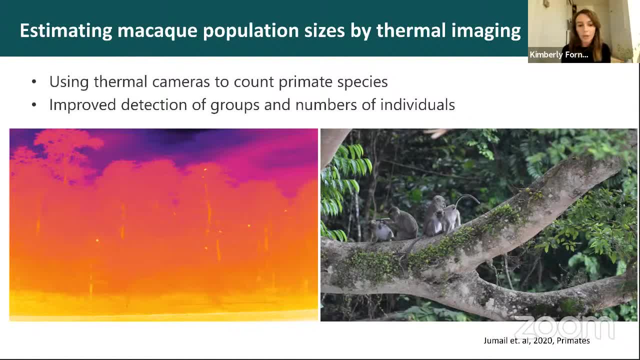 are at the side of a river with macaques roosting in trees, And what you can see is from these thermal images. you're able to pick out these little bright dots, which are actually macaques roosting within these trees. 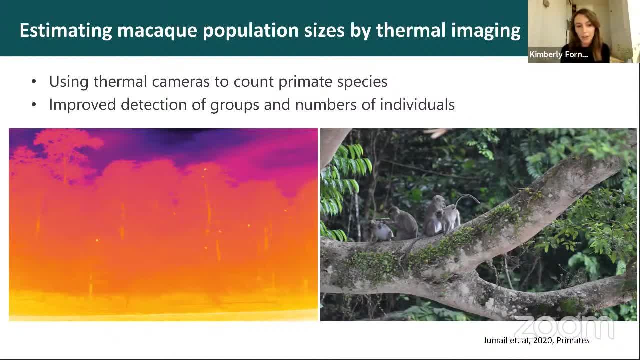 So from this we're able to identify how many macaques are in an area, And this is particularly useful when there's very poor visibility, so situations like at nighttime or with very high canopy cover, And then, of course, we really needed to look. 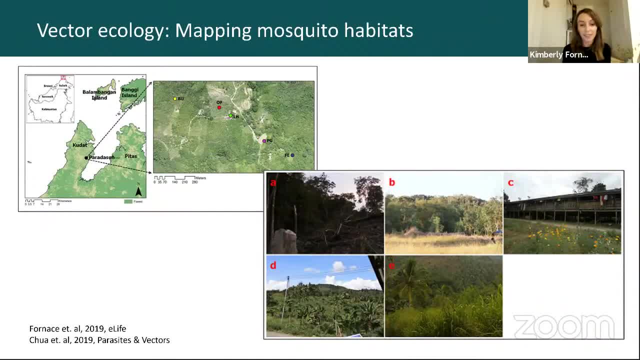 at mosquito ecology. so where are the mosquitoes as well? And to do this we did a number of entomological studies in different habitat types. so looking at different types of forest, different types of agriculture and villages and close proximity to households. 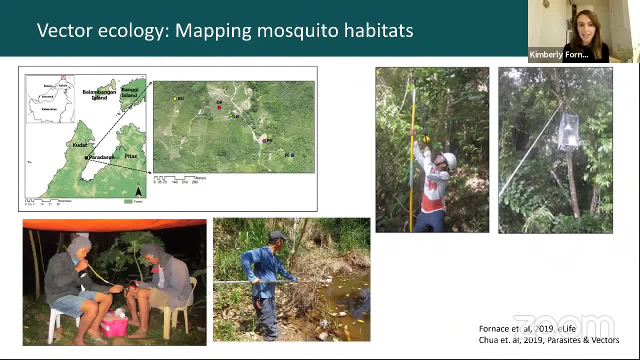 And we did a number of different studies to look at mosquito ecology. in this area We collected, And So one we looked at human landing catches, so actually collecting mosquitoes as they were coming to land on a person's leg. So this is the example in the bottom corner. 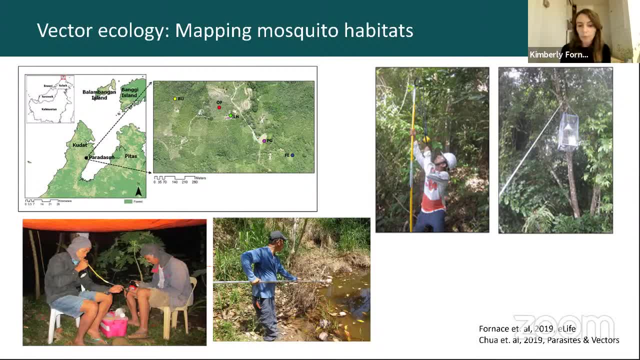 And working out how many bites a person would receive As well. we looked at different water bodies so whether or not they had this mosquito larvae, And we conducted a number of different mosquito trapping methods that we used at both ground level and within the canopy to look at what mosquito distributions are. 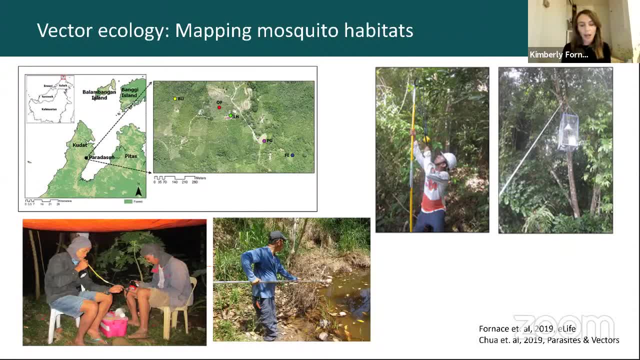 within these different environments. So we looked at different water bodies whether or not they had this mosquito larvae As well. we looked at different water bodies whether or not they had this mosquito larvae, And so from this, what we were able to determine. 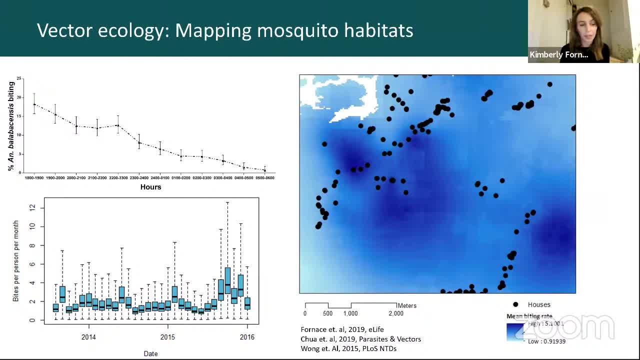 is that the primary mosquito vector of Plasmodium nolzi within this area is Anopheles balibicensis. This mosquito bites outdoors And the highest biting times are between 6 PM and 10 PM, And fitting this mosquito data to a number, 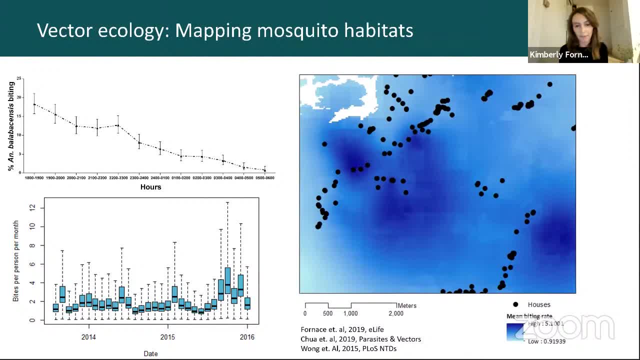 of different environmental covariates and predictors, things like rainfall and weather, we're able to actually develop models to predict how many bites a person is likely to receive at a particular location at a particular time, The kind of final component of this. 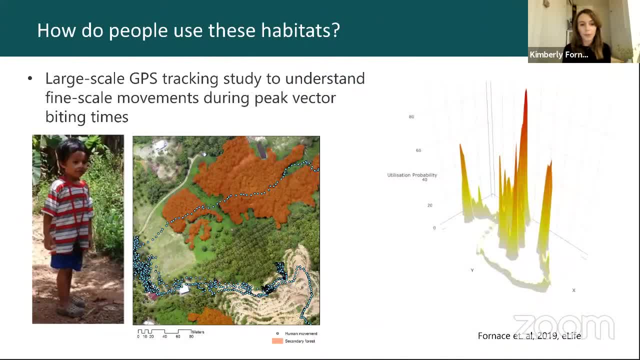 is looking at how people fit into these landscapes, And so we're particularly interested in where people are at these hours between 6 PM and 10 PM, when mosquitoes are biting, And we know this is occurring outside. So to look at this, we conducted a GPS tracking study. 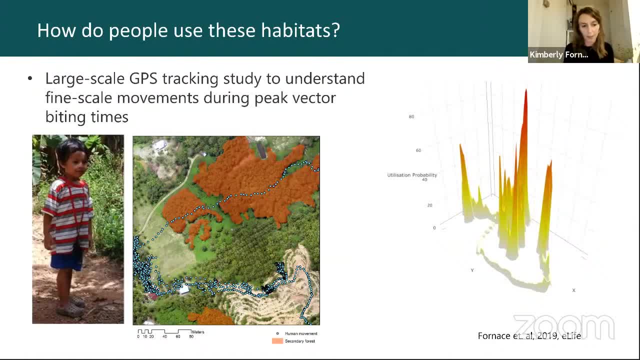 So it's a bit difficult to see from this picture, but this child is actually wearing a small GPS tracker like you would take for a run, And we were able to collect a number of different types of this very detailed movement data that allows us to build models of individual space use. 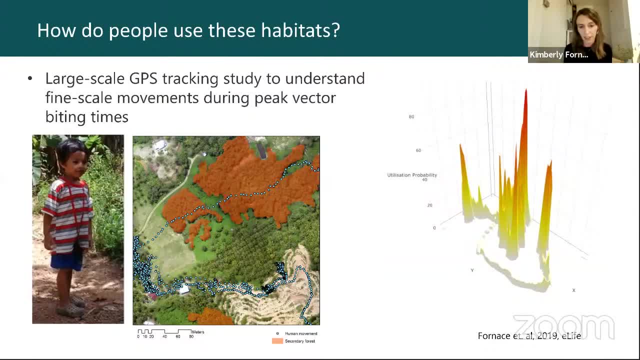 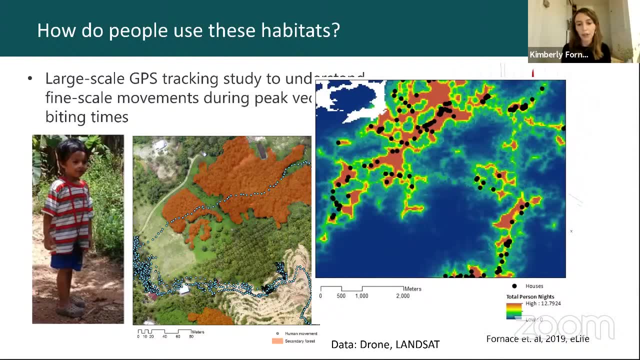 to work out the probability an individual is in a particular location at a particular time And we're able to then use all of this data to expand at a community level, So to look across entire villages where people are likely to be going during these times. 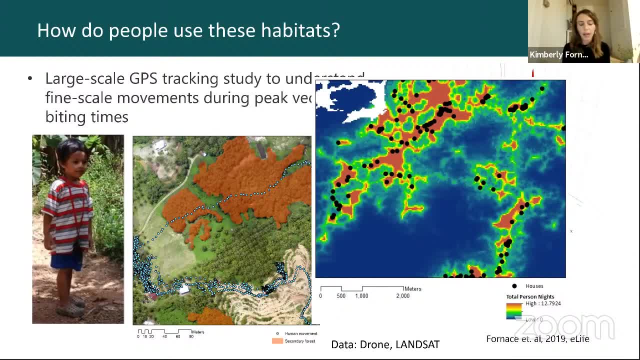 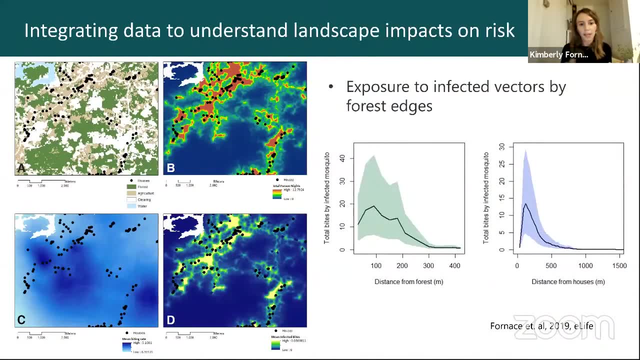 and how often they use these habitat types. And finally, thinking about how we integrate all these different sources of data together. we have data on land cover. We have data on human space use and movement, Data on mosquito density. macaque densities. 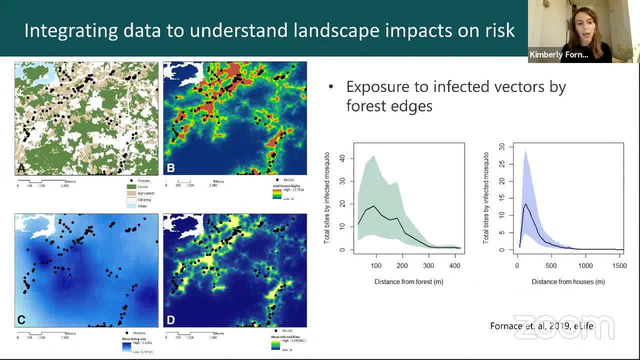 and infection prevalence within these populations, And what we can show is that we do see this. increased exposure to infected mosquito vectors is occurring around forest edges, So people are likely exposed around forests, but also still in close proximity to households, where they're spending most of their time. 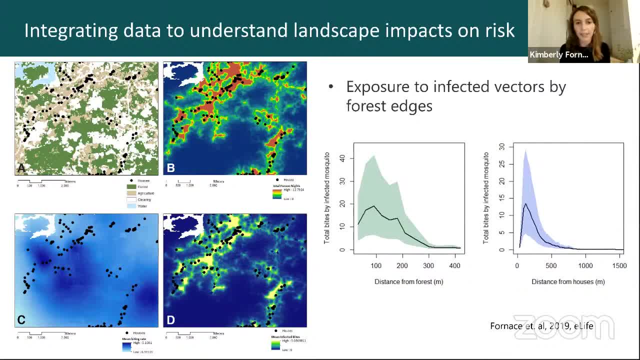 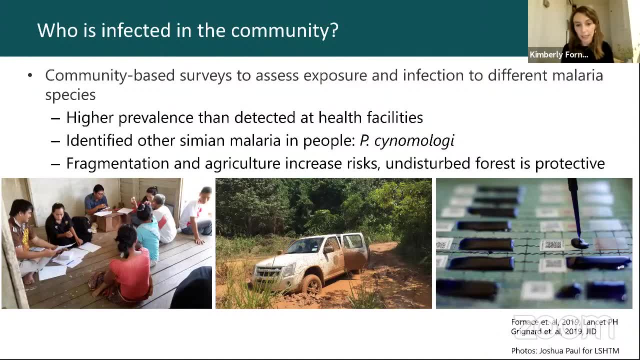 Finally, we wanted to look at much, much wider spatial scale to see if these patterns are true at population levels. So this is a number of community-based surveys we conducted. We actually tested over 15,000 people to determine exposure and infection. 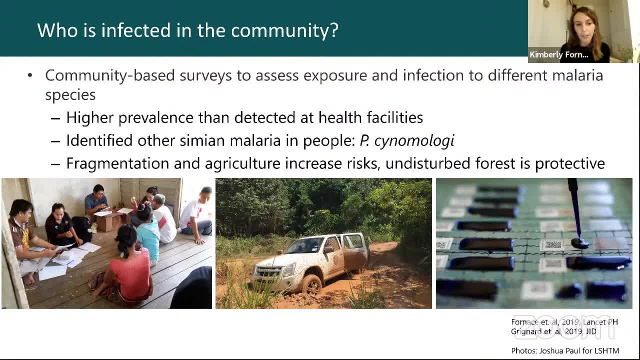 to Plasmodium nullzii and other malarias And what we found is there's much higher prevalence than was detected at health facilities. And we found there's not just nullzii in this population, but there's also other simming malaria. 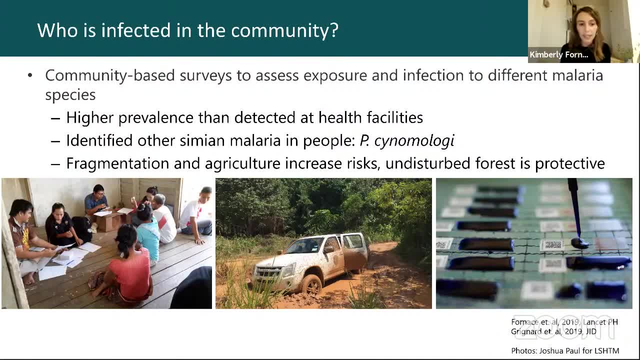 so Plasmodium sinamulgii, And we do see these patterns where there's very strong associations with fragmentation, agriculture increasing risk and forest actually being protected, And so with that I'd like to end there. So thank you very much, and to all the people. 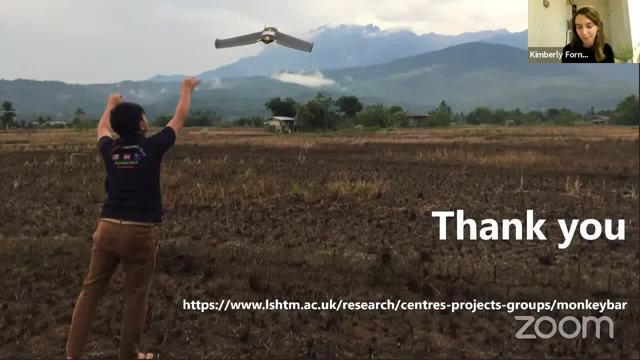 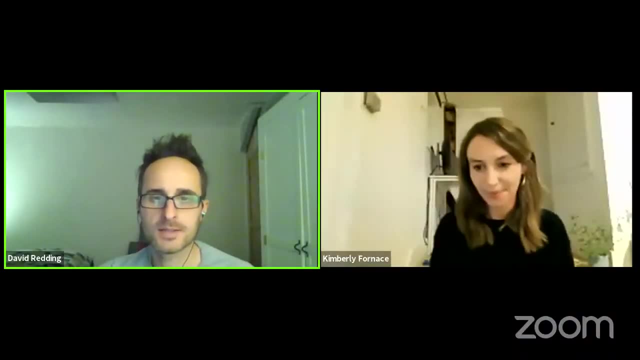 who participated in this. Thanks very much, Kimberly. That was a great talk. I think getting these detailed pictures of what's going on really adds loads more depth to some of the kind of general you know the studies that we've been looking at about you know. 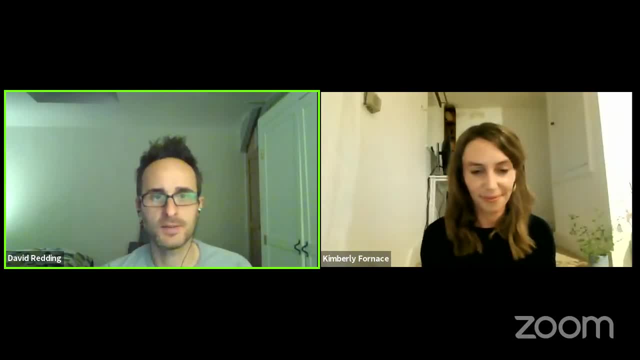 saying: well, you know, range edge is important, but it's really interesting to see how you approach it from all these different angles. So let me just have a quick look at some of the questions. So I guess there's a question here saying: should we target? 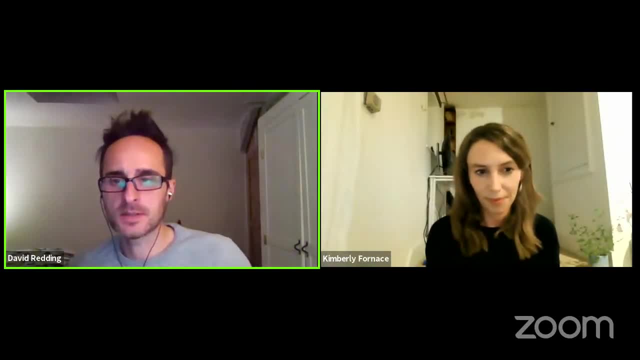 Again, this is one that I asked before- but target active managements against certain species that increase risks, And I guess for mosquitoes that's a bit of a no-brainer really. Yes, we try, not always successfully. It is really challenging, particularly. 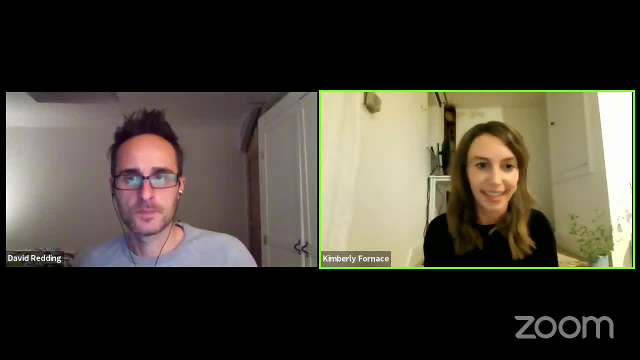 when you're looking at outdoor biting and mosquitoes that live in forests. So many of the things that we use around households, like bed nets and things that protect people, are not particularly effective in this situation. Oh OK, I've got one here. that's, oh, I've. 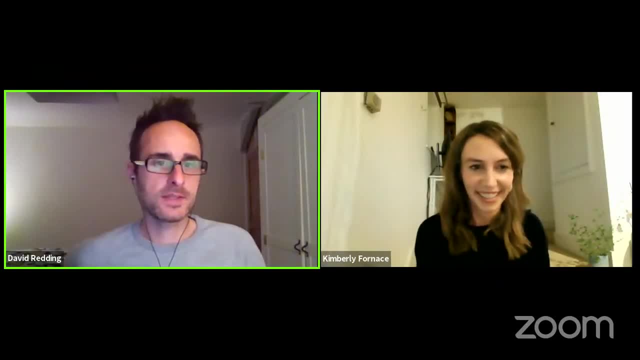 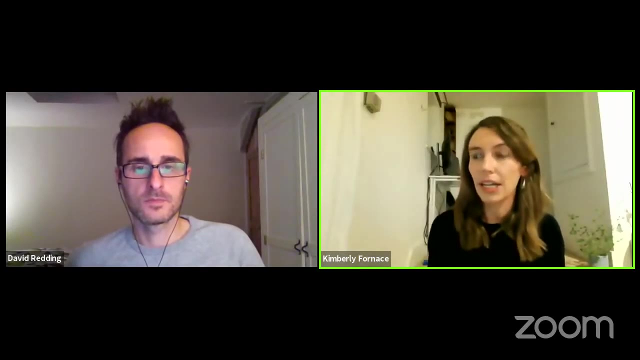 got a couple of questions appearing for you now. What evidence is there that Null's eye can be transmitted from human to human, as well as macaque to human? Oh, that's a good question actually. So it can be transmitted, And the reason we know that is that in the 1930s, 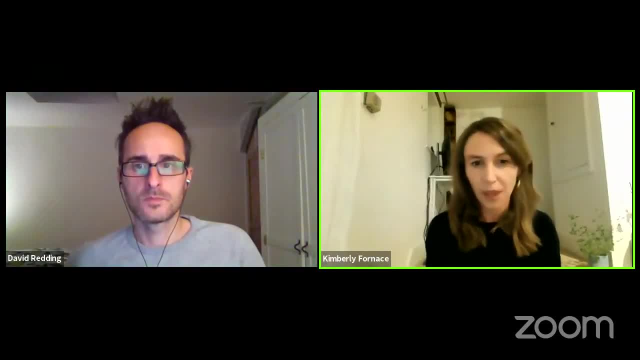 they actually looked at Plasmodium nullii as a cure for syphilis. So there are some very ethically dubious studies that infected American prisoners or volunteers with Null's eye to show that you could have Null's eye that could be passed to a mosquito. 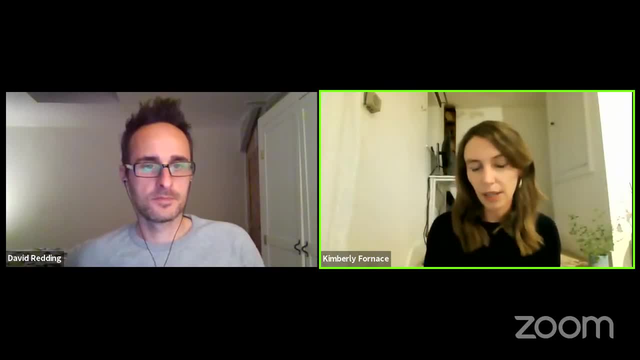 and then be passed to another person. So all of the genetic evidence and the modeling evidence we have so far suggests that this very rarely occurs in the wild. But it is actually the focus of some ongoing work we have with the World Health Organization at the moment. 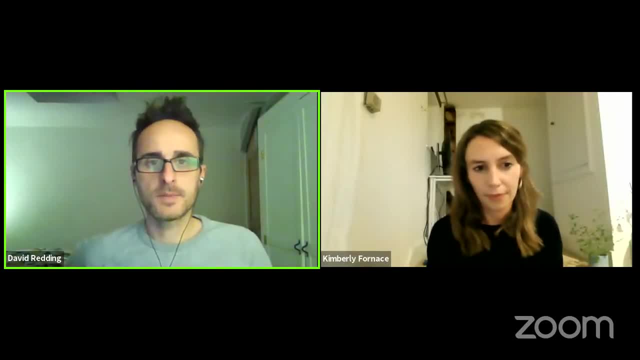 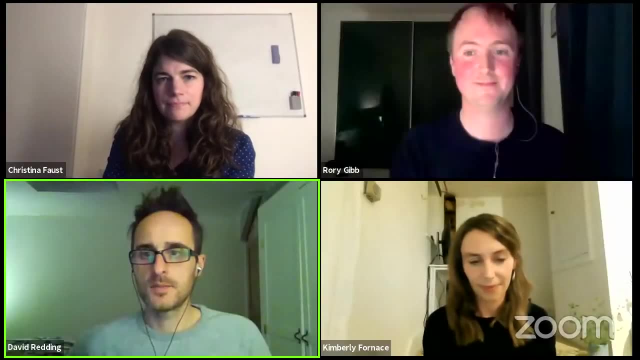 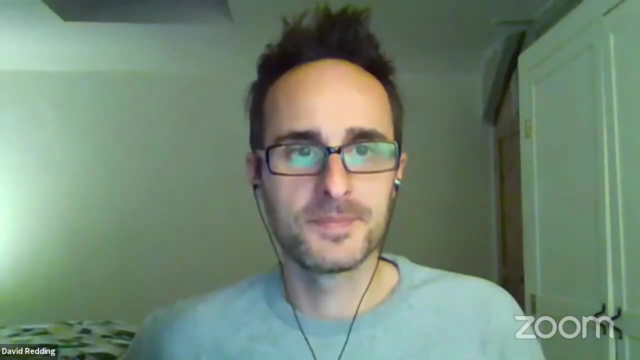 OK, well, because we're running a little bit late, I'm going to stop there with questions. I think we're going to open it up now to a Q&A where I'll go through some of these questions and see if anybody wants to answer them. 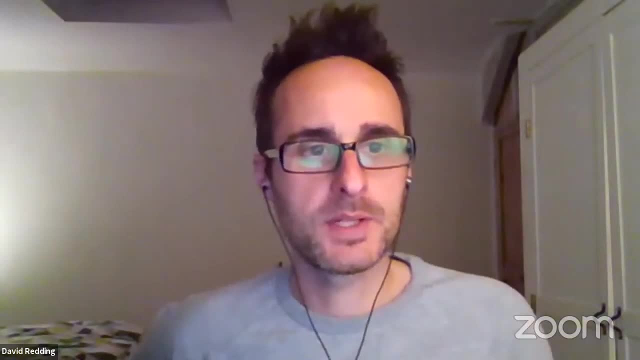 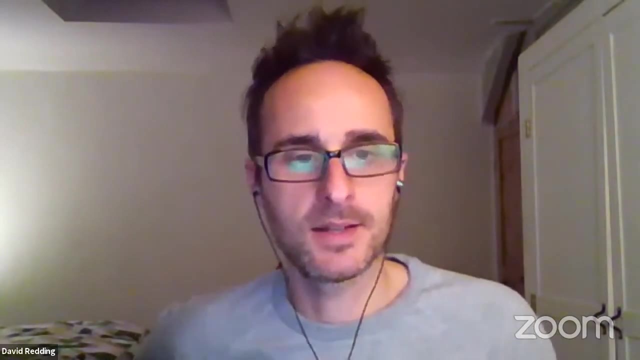 So, starting at the top here, the most popular question here is: how significant is the impact of climate change on the propagation of zoonotic diseases? Is it likely that climate change will cause more pandemics in the future, such as the one that's happening now? 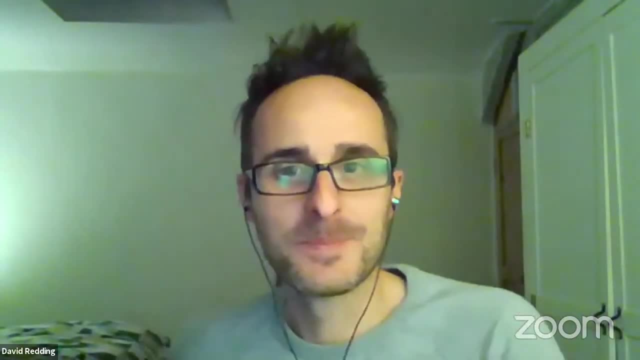 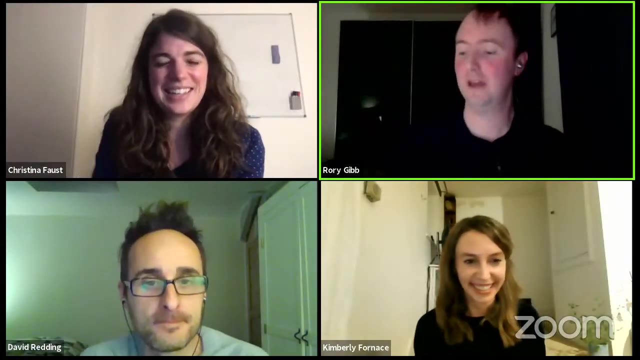 Considering we're talking about land use. I don't know whether anyone wants to take that one on. If not anyone, I can go Yeah, Yeah. so I mean it's a huge question in a sense, right. So in a way, when we think about land use, change. 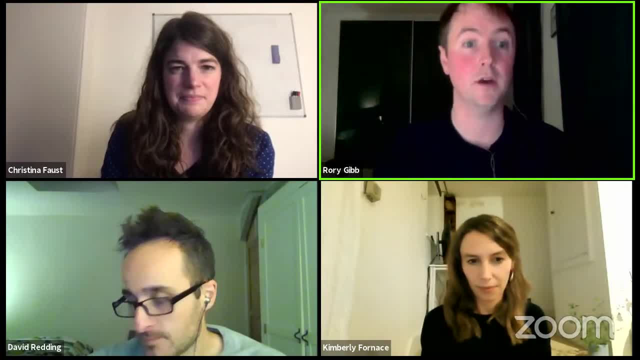 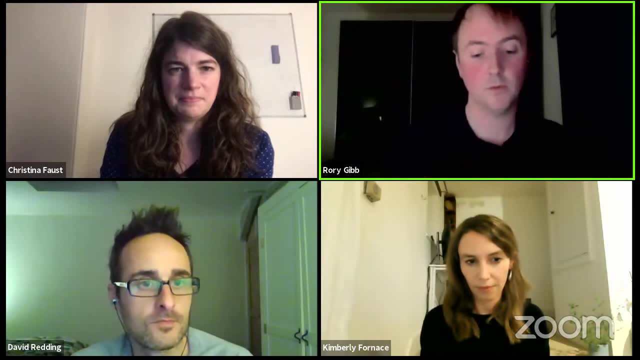 we're often thinking about ecological processes that are going on at relatively localized scales. We're thinking about, as Kim was showing, these kinds of quite small-scale landscape transformations that can really influence risk along borders of meters or kilometers. But when we're thinking about climate change, 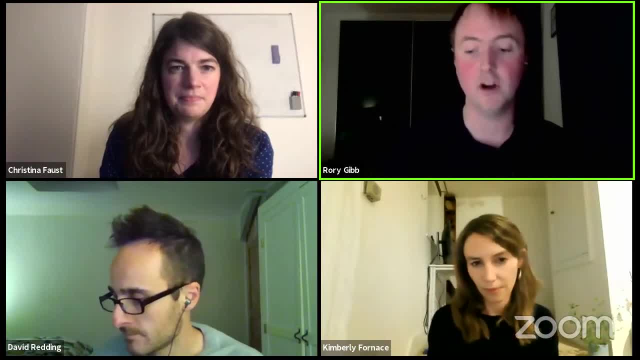 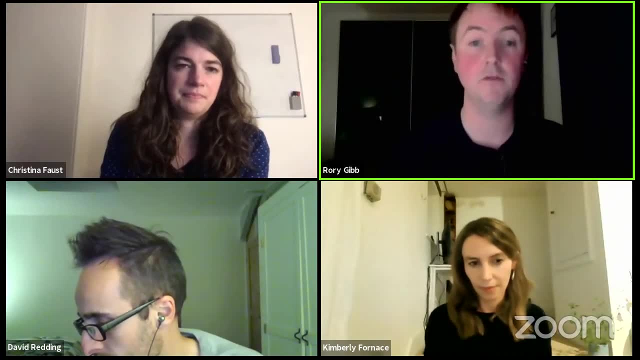 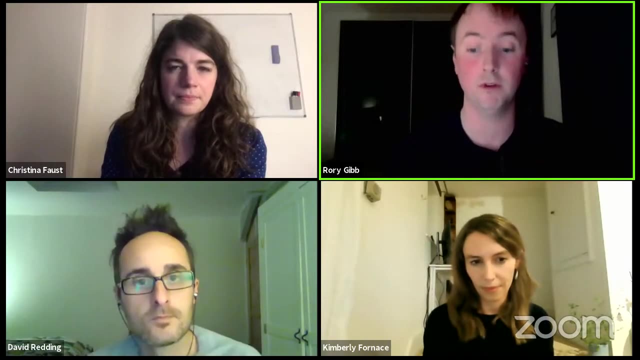 we're thinking about really profound shifts in how the environmental conditions allow species to persist, And so there's already evidence that a lot of species are moving around the globe to track optimum climatic conditions, to basically move away from areas that are getting too warm for them. 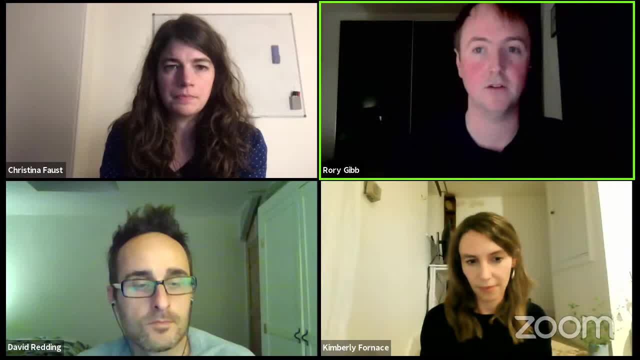 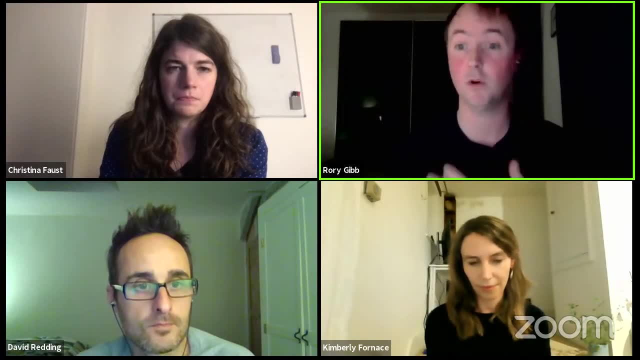 and into areas that better suit them. So there's a few factors going on here. Firstly, we're going to have novel communities emerging in the future, right New species that haven't come into contact with each other necessarily before coming into contact more. 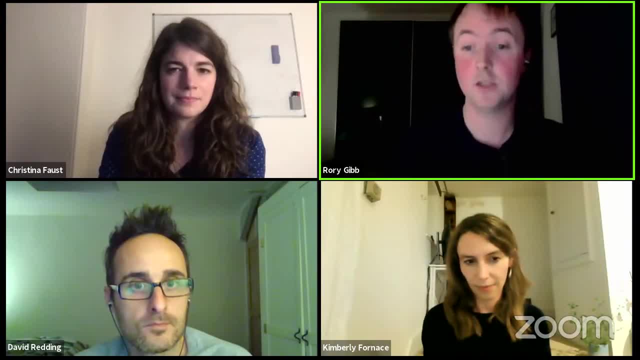 So this could potentially Lead to kind of increasing spillover events, not only between, I suppose, wildlife and people, but also between wildlife. So there are kind of conservation issues here as well. But just to give one specific example rather than ramble. 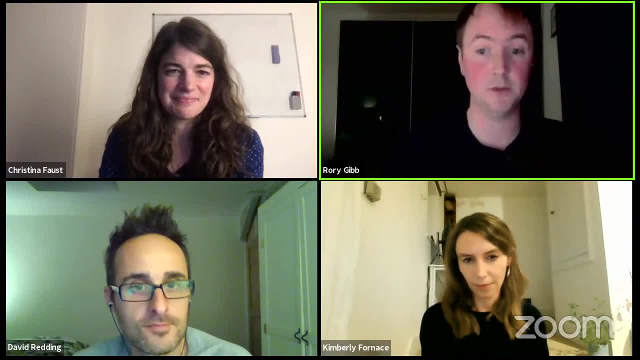 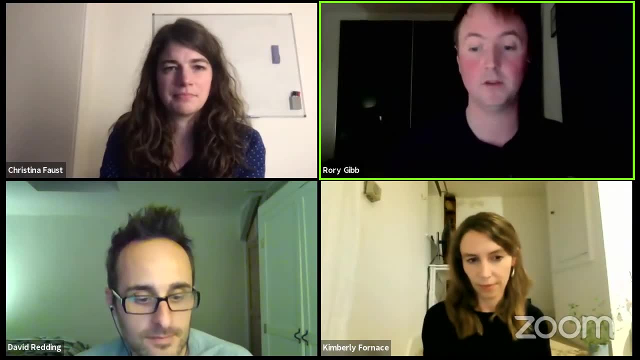 I do quite a lot of work on dengue, And so the Aedes mosquito that transmits dengue is obviously an urban specialist. but also there's kind of evidence that as the planet is warming, that it's spreading more, more. 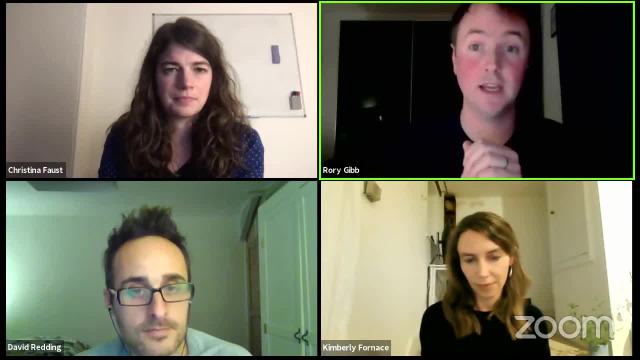 more widely across the planet And this is potentially leading to kind of bigger outbreaks of dengue in places that haven't experienced it before. There's absolutely already reshaping disease risks now and will continue to be a huge influence in the future. Anyone else? 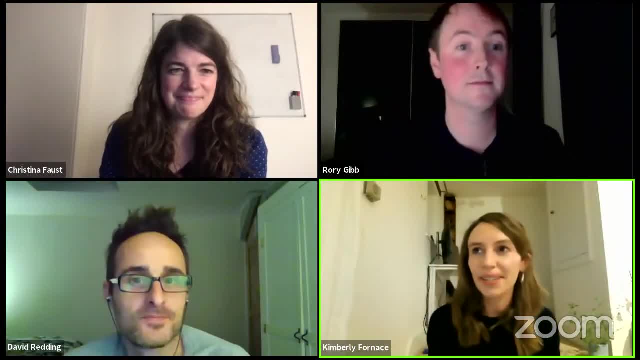 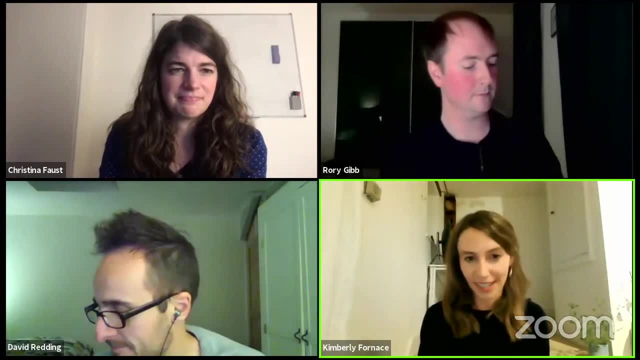 Yeah, I mean I agree with everything you've just said. The other thing I would say is that land use and climate change are not disconnected. So we've seen really large forest fires. We've seen extreme weather events that have flooded areas. 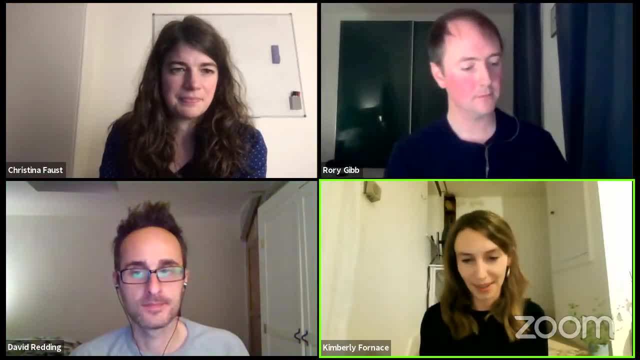 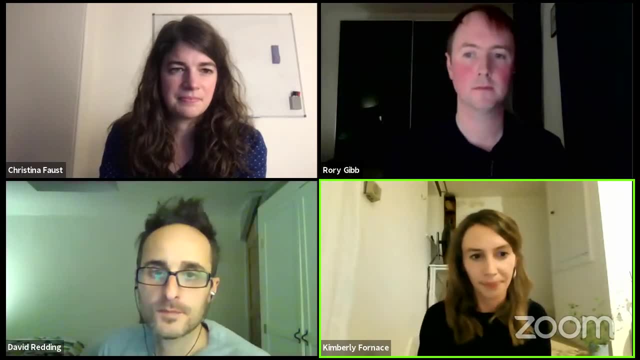 So when we're talking about land use change, we're often thinking it's only human-caused or directly human-caused And there is an interaction between these two and that are incredibly important for disease. Do you want to say anything, Christina? 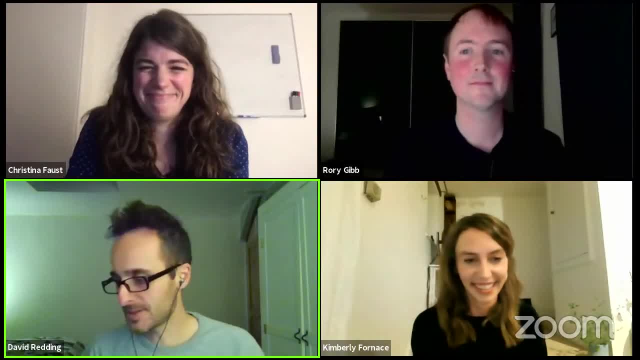 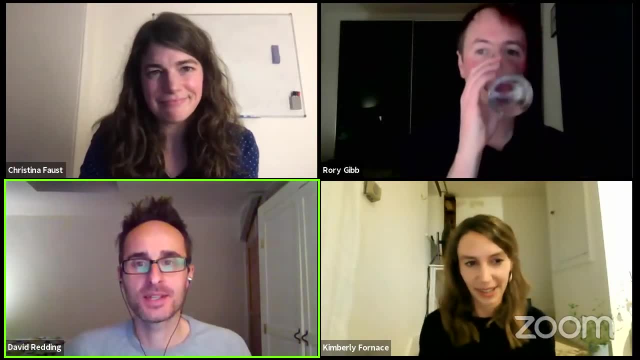 or should I move on to the next one? OK, just to say that was my point as well. so you stole it. OK, great, Let's move on to the next one. So the next one. I'm just doing them in popularity here. 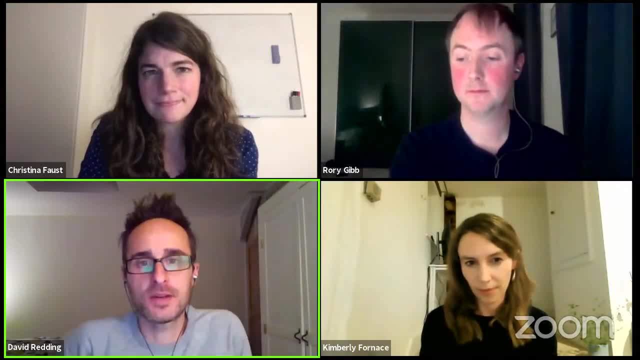 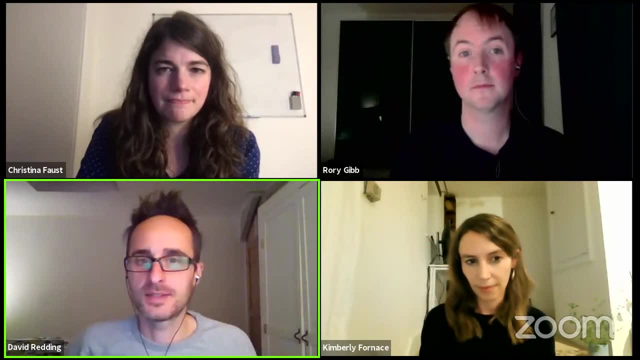 Do ecotourism practices in which people have direct contact with wild animals make it easier for pathogens to make the leap from wild to domestic hosts? Can tourists be made more aware of this risk? We see this is a big problem So I can jump in on that. 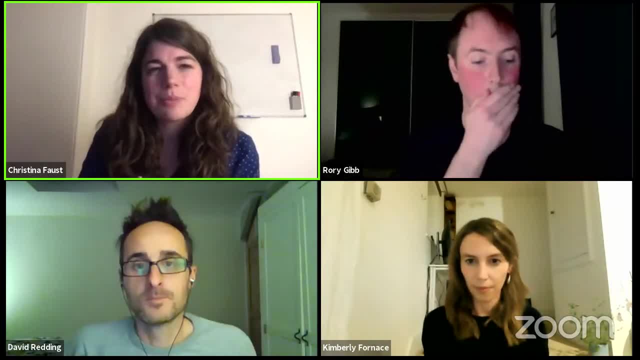 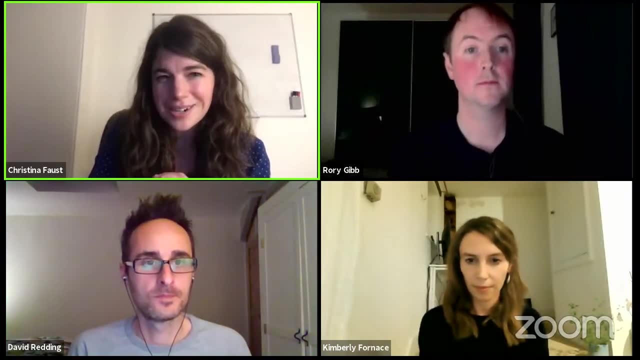 So I think it is a risk for certain areas, but I do think there are conservation organizations that do a really good job of addressing this. So I think conservation doctors in Uganda, which kind of deals with communities around mountain gorillas which are very sensitive to human. 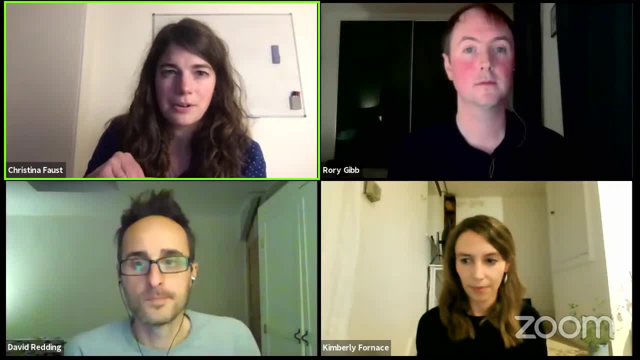 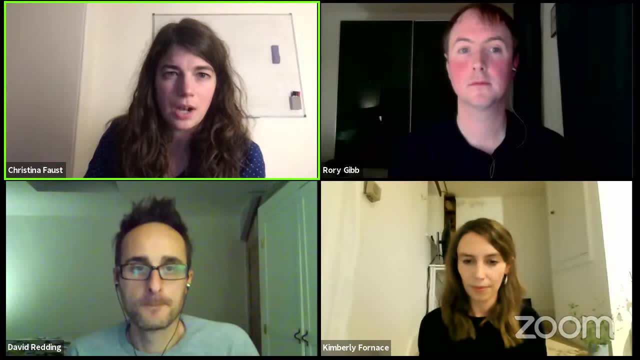 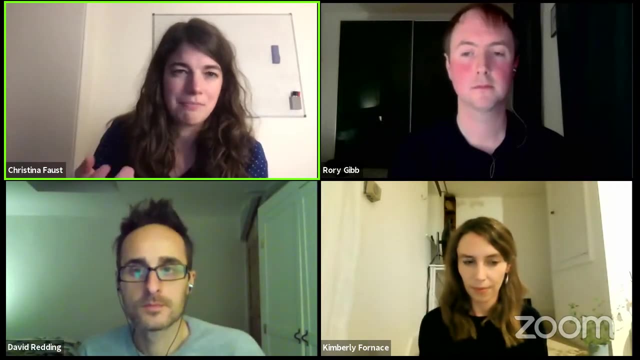 pathogens do a really good job about educating visitors and kind of promoting this One Health idea. So there are organizations that do a really good job where there's lots of evidence that this is really important for the wildlife and human interface. So, yeah, I'm going to get that one. 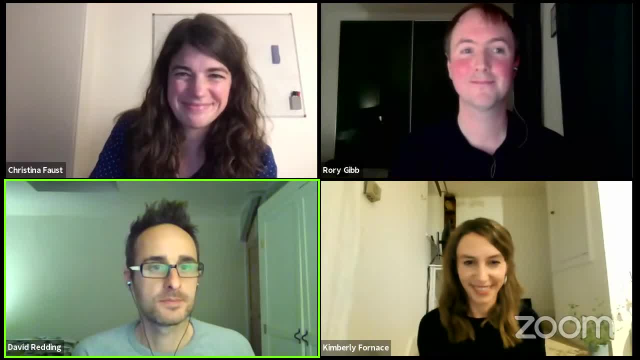 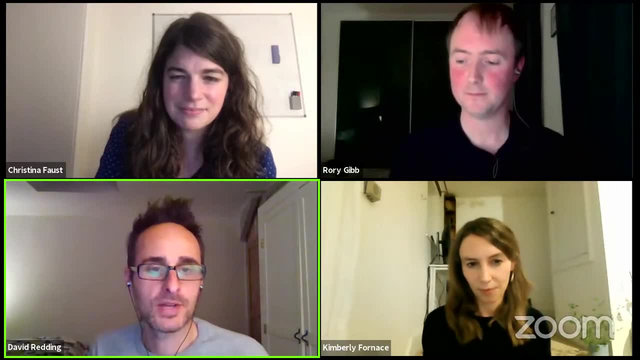 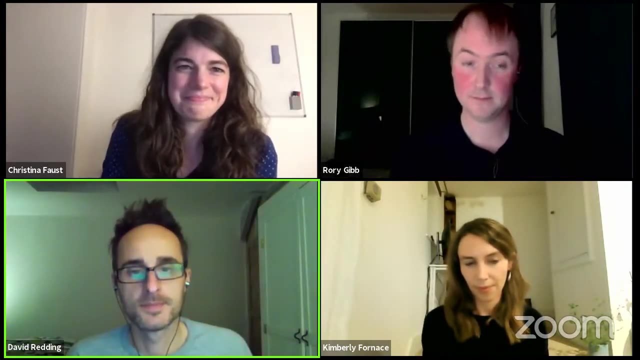 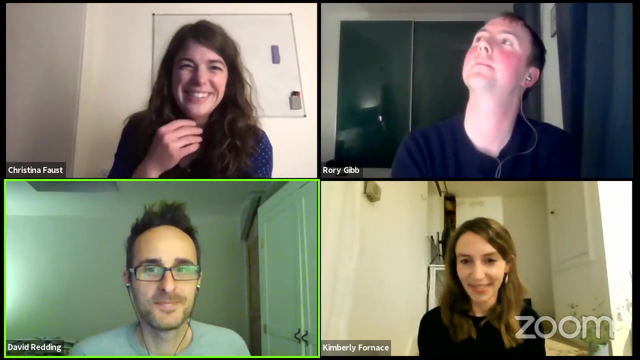 I can't really speak to that, so I'll move on unless OK. so the next question here: does rewilding areas and bringing back natural habitats without human interference decrease the likelihood of diseases spreading zoonotically? Anyone, I can have a go. 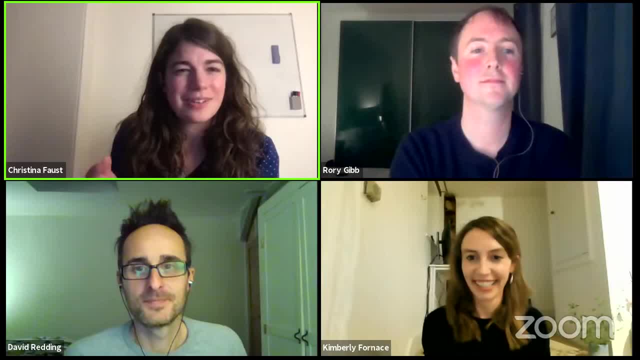 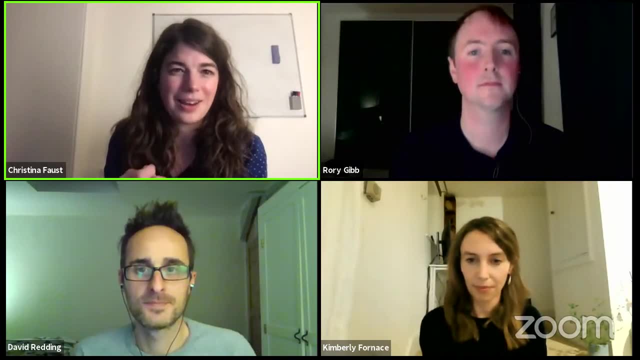 Yeah, So there's not much research done on this yet. So we know a lot about how communities disassemble, so how they break apart, But we're not great at understanding how they reassemble. So In Scotland there's been huge rewilding efforts. 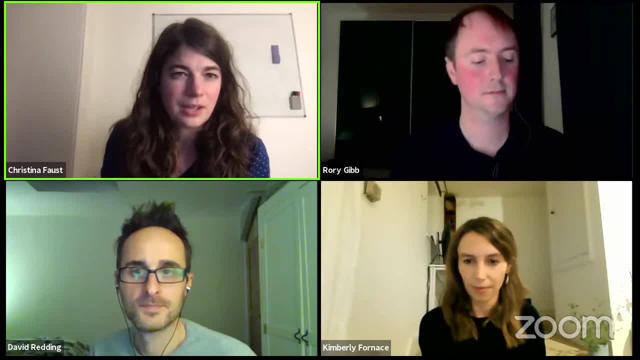 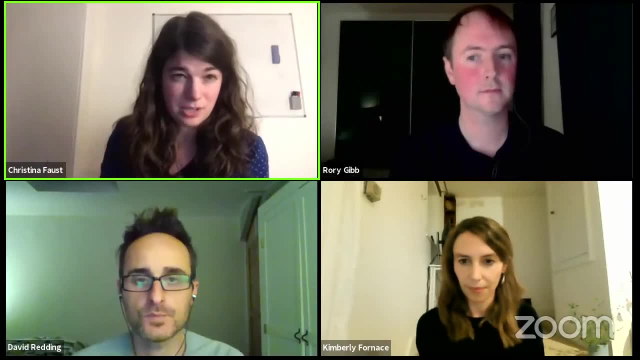 And I think there is kind of an interest alongside of this to look at how that changes Lyme disease and important domestic pathogens like domestic sheep, pathogens like liver fluke. But I think the jury's out. I'm not sure of anyone who's looked at this sort of process. 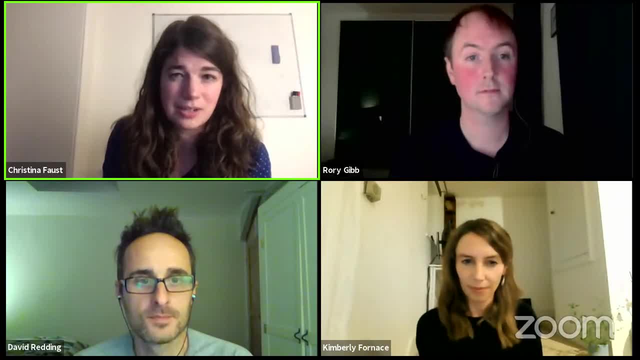 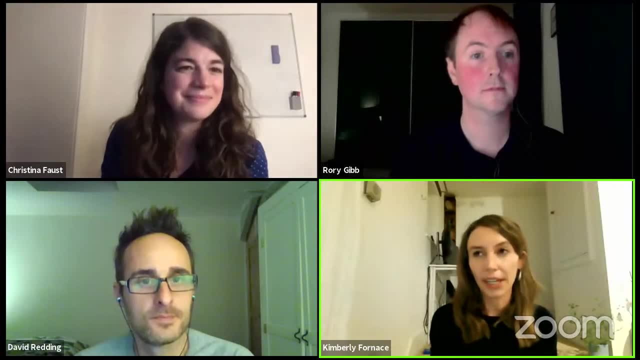 But I think it's going to become increasingly important, as this is an option. Yeah, I can add that there are some ongoing projects in Borneo Looking at reforestation and particularly reforestation to meet some of these climate change commitments. 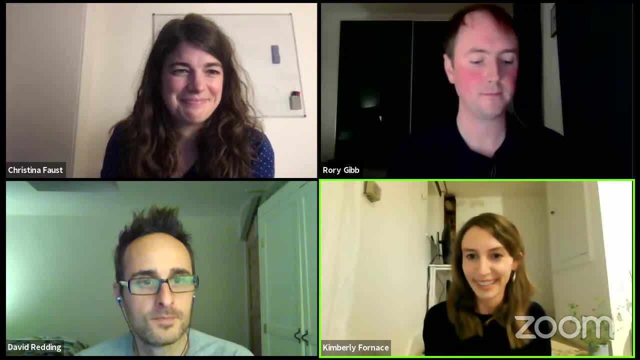 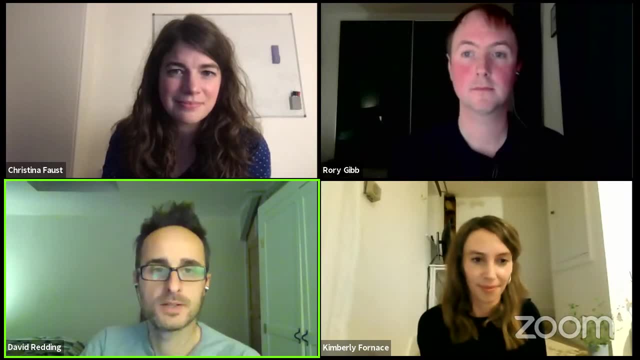 But again I think it's the same conclusion. where kind of the verdict is out? I guess my initial thought is: how much is reforesting, rewilding going to work with increasing populations, increasing demand for food and non-sustainable action? 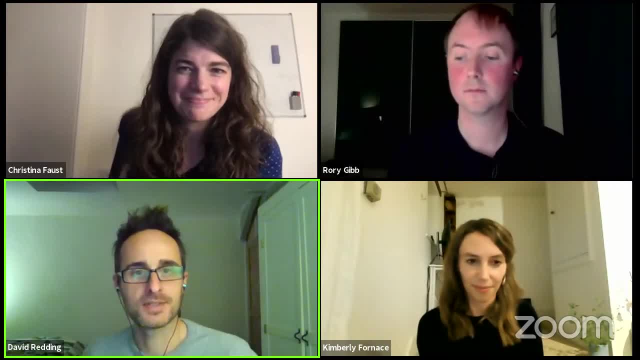 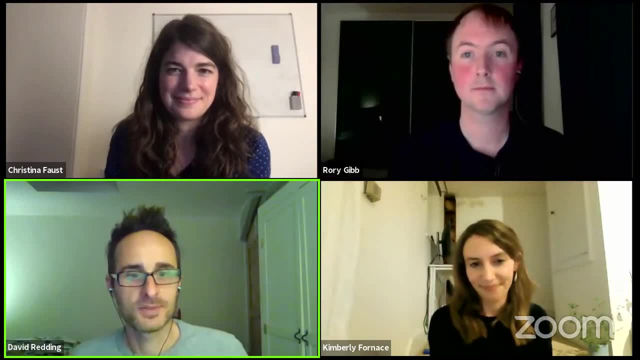 So I guess it's one of those things that whether it's academically interesting versus whether how much is It's going to go ahead is something that I think about. Rory, do you want to say anything, or should I move on? 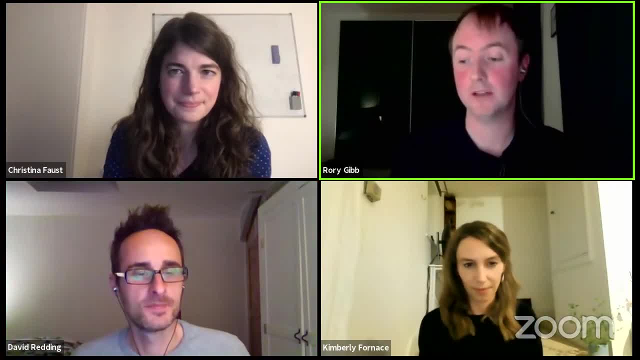 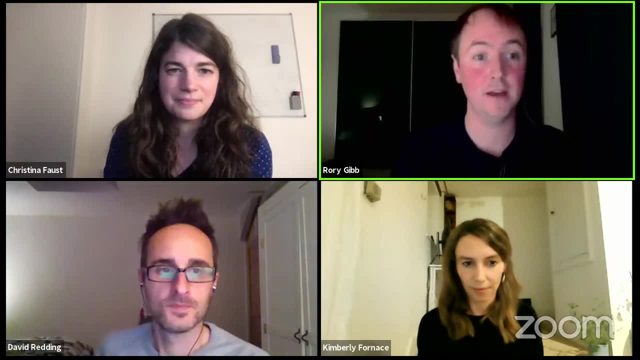 The only thing I would say as well is that I think, if we're thinking about global scale issues, I think that we know that some of the most effective ways to prevent people from getting sick is to improve their socioeconomic status in various different ways, So it isn't solely an ecological problem. 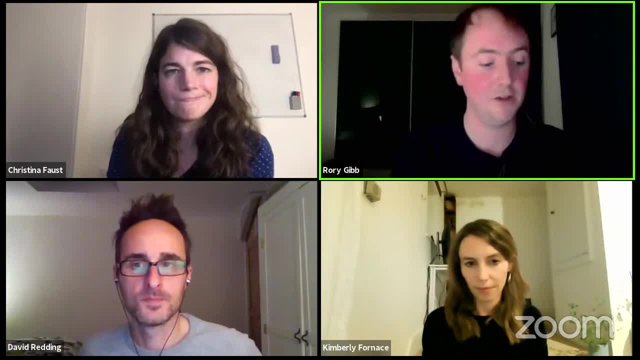 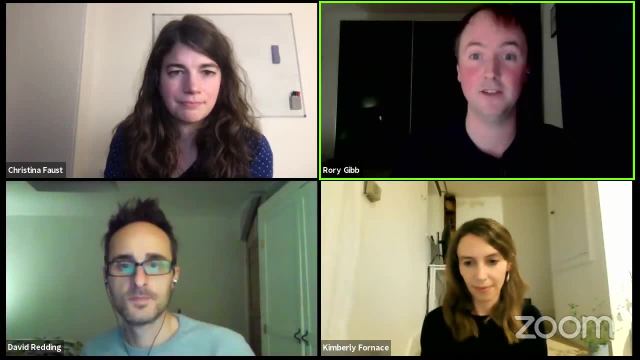 Like. a very large part of this is also to do with understanding how the ecology interacts with where people are at, And I think when we're thinking about building resilience to kind of climate change and changes in ecosystems, we need to be thinking about how to improve people's 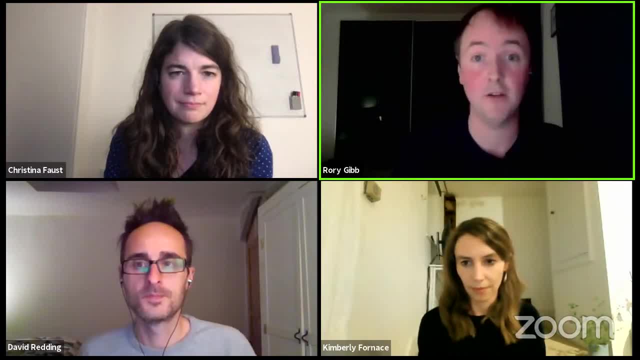 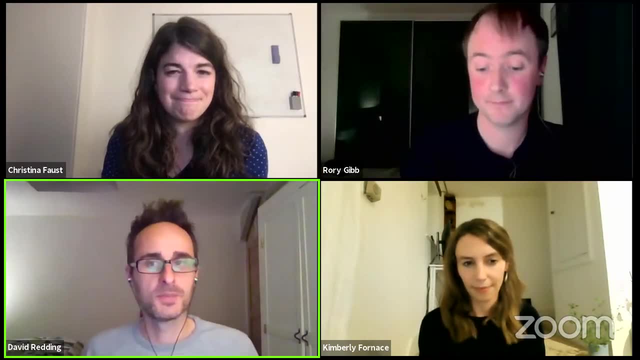 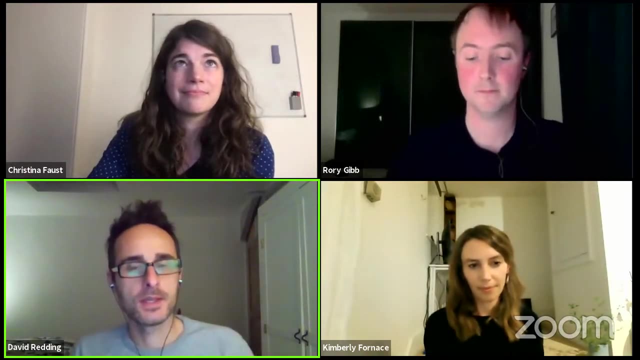 socioeconomic status in ways that helps give them better access to health care and reduce the chances of these kinds of spillover events occurring. Yeah, couldn't agree more. OK, so the next question here is: so: can we design agriculture? Can we design agriculture? 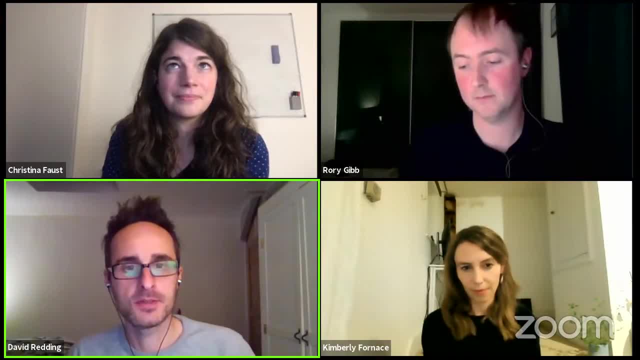 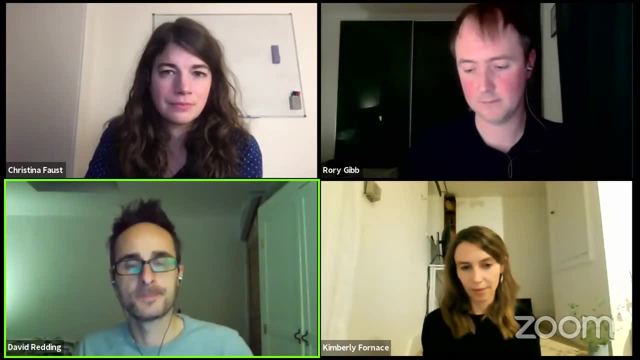 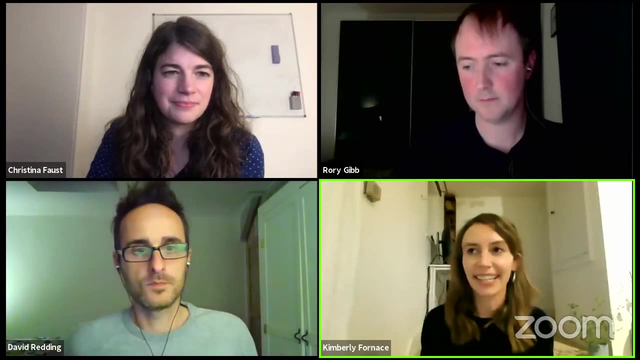 Can we design agricultural landscapes that are less risky from disease transfer viewpoint, eg a greater mosaic of trees and crops and agroforestry? It's something that there's quite a lot of ongoing work on, and I think malaria is actually one of the best examples of this. 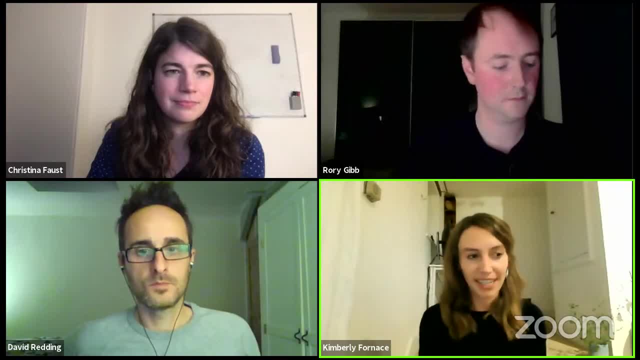 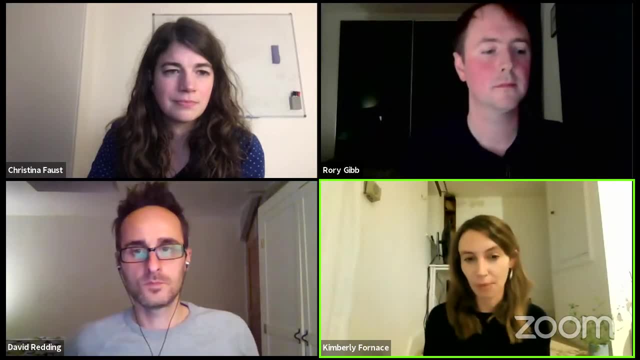 So it's quite famous kind of malaria history of people, particularly in Italy in the 40s and 50s, filling in the ditches and managing these agricultural landscapes in a way that really decreased mosquito, And so there is evidence that this can work. 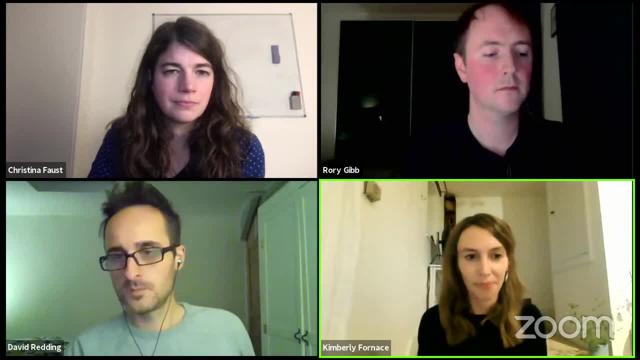 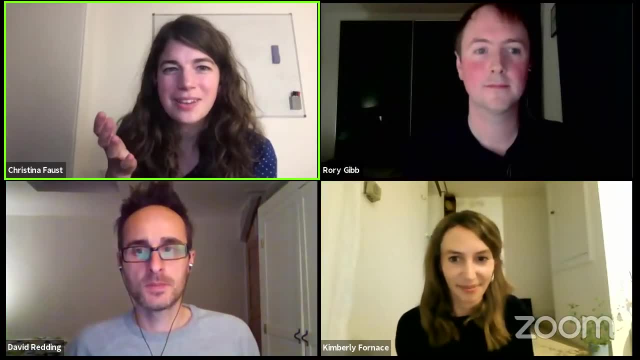 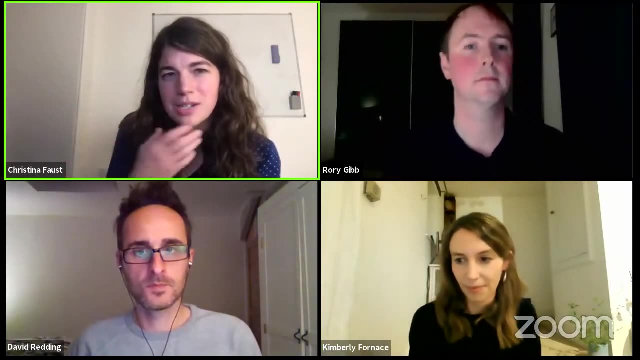 and I think it's something that really needs to be focused on Others. I don't know if you have anything from the loss of fever perspective, but in some landscapes and agricultural landscapes, when you're managing for those pests, if you have a more ecologically friendly management. 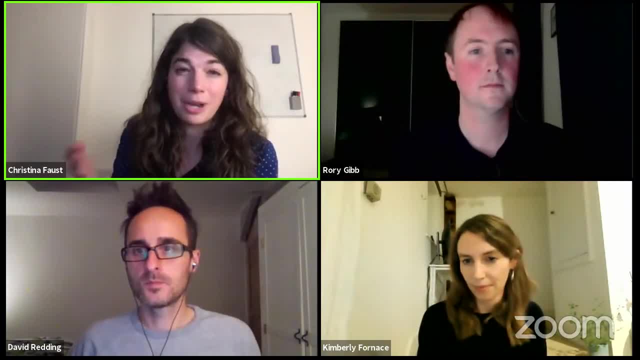 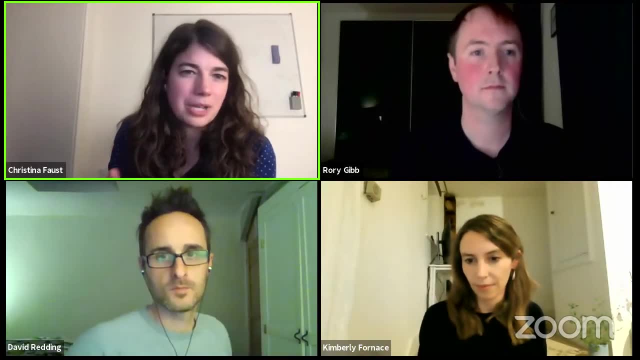 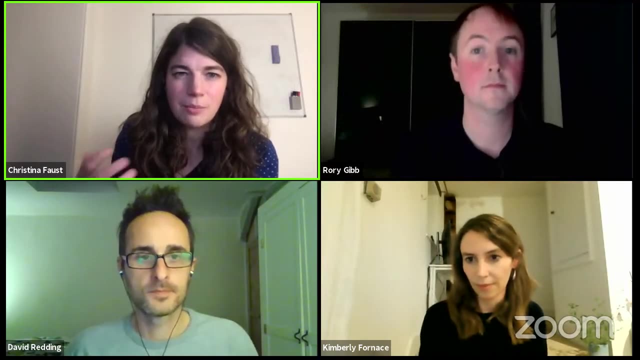 of agricultural systems, you can actually support higher biodiversity of rodents. that decreases the, and the data is still out on that, but it seems to be the case, where you have more sustainable agricultural systems, that you can actually reduce prevalence of that important zoonotic reservoir. 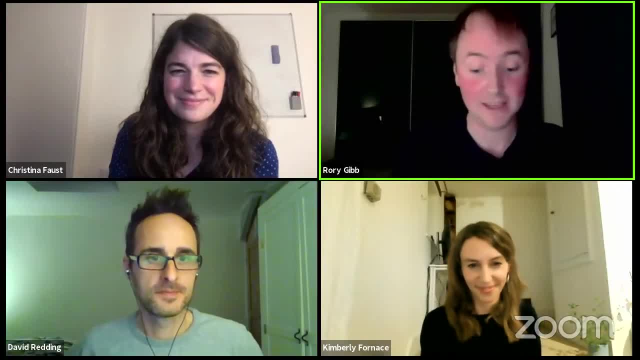 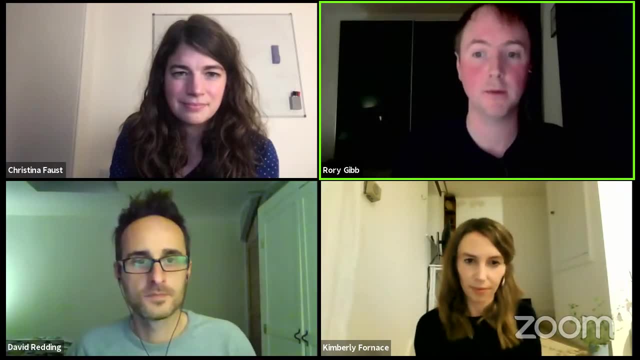 Have you all each want to say something? Just to say yeah, I mean, I think that this is a really important question for Lhasa and I think it's something that's kind of on the list, but, yeah, of increasingly something that we've been talking about and thinking about, but, yeah, the kind of i 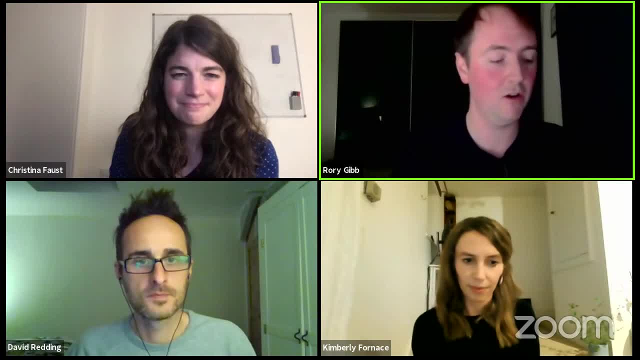 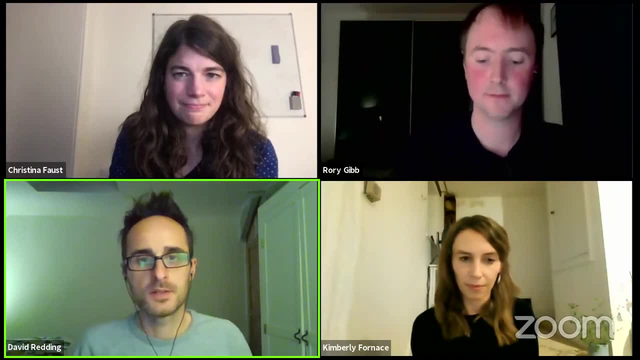 guess the jury's out on what it means for lhasa, because there's so in a lot of ways we don't really understand how big a deal lhasa is and how widespread it is. yeah, i guess from some of the work that i do, it's it's that thinking about our sort of unintended consequences of how, how we you. 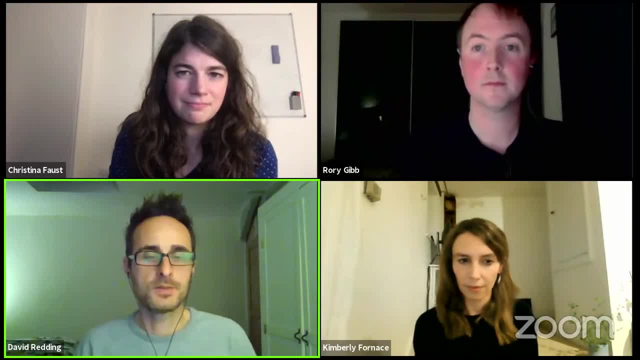 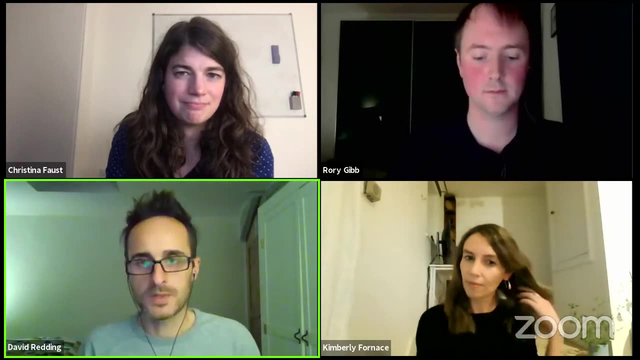 know, manage landscapes, and thinking that, well, okay, let's do something to get rid of um, you know, let's stop uh hunting happening. so then we bring in lots of livestock and all we're doing is transferring from one problem to another. so i i think that, um, when we're talking about managing 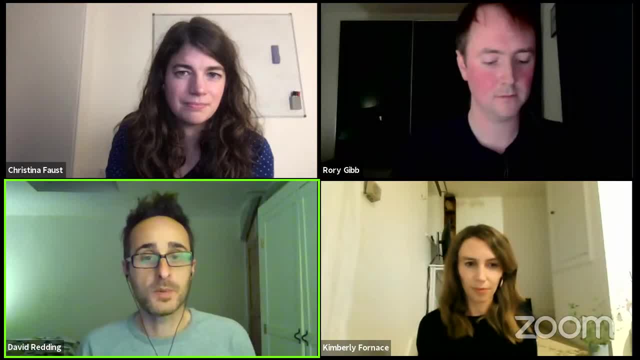 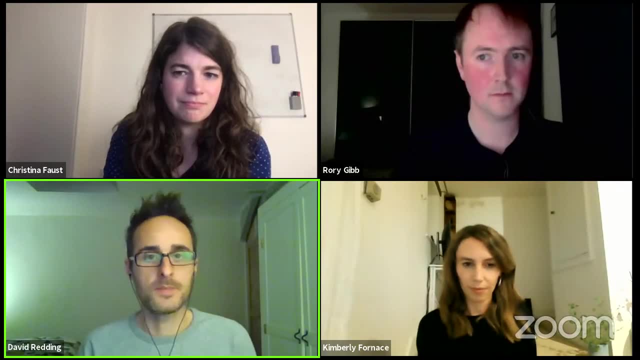 and designing landscapes, that that some of this kind of general work might point towards, you know, kind of whether land sharing or land sparing type, um sort of divisions may be most effective, or whether you know we're currently ending up in what christina was talking about: these kind of worst case scenarios most of the time 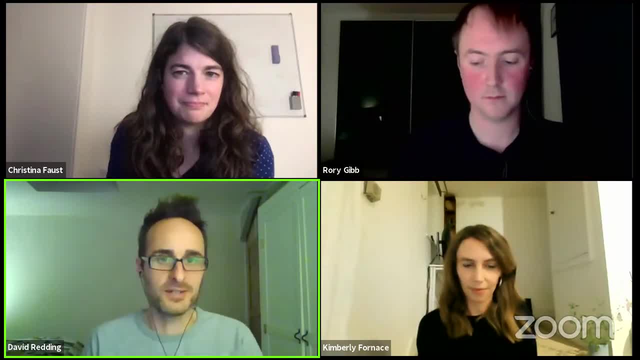 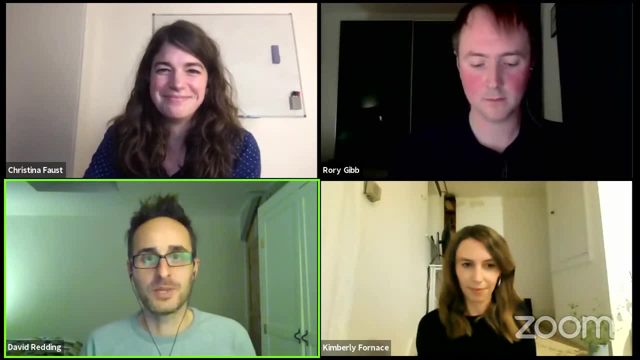 where we're just lots of things are overlapping. we've got lots of edges, you know, bringing it in kimberly's work, so so whether we're just sort of sleepwalking towards this kind of perfect storm situation, or whether we we can actually start kind of trying to think more holistically and 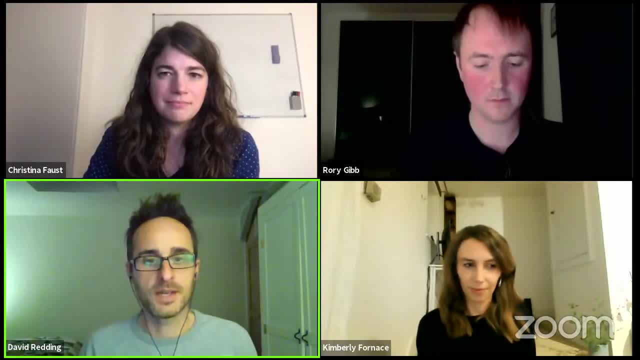 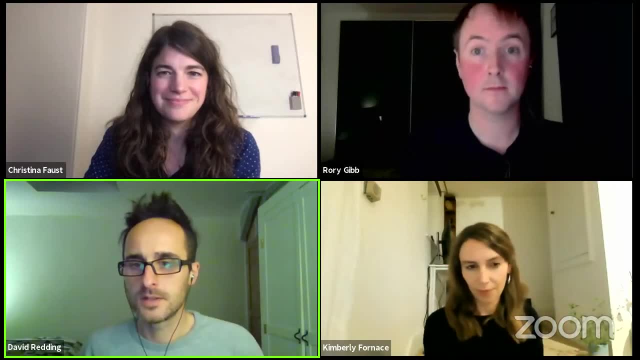 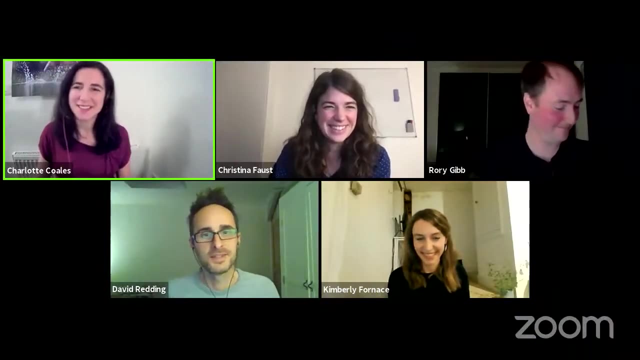 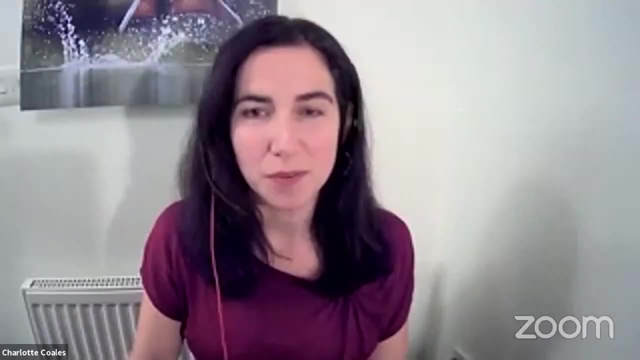 and and bring these, these sort of elements together. so i think we are reached the end. i think that's right, is it? um? um, I'll come, i'll come back in. yeah, thanks, so much dave for for keeping an eye on time. i'm sorry. sorry, we can't keep going because there have been so many questions coming through. um as a. 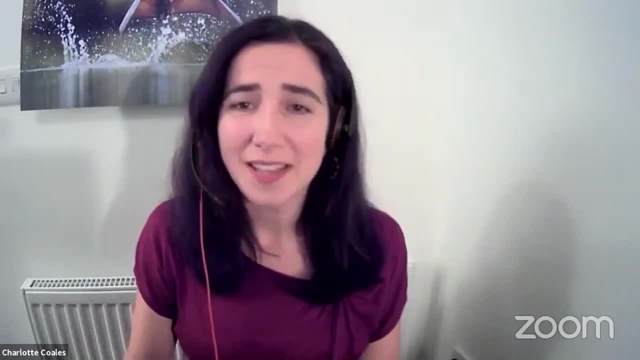 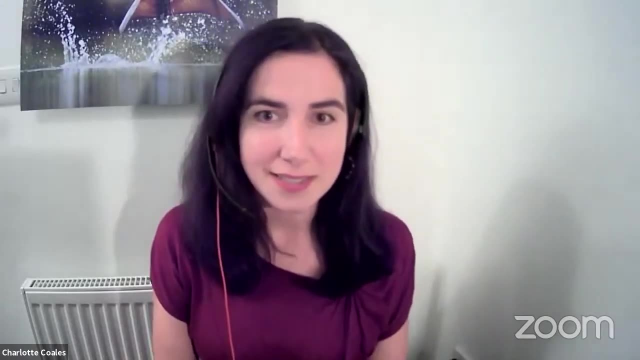 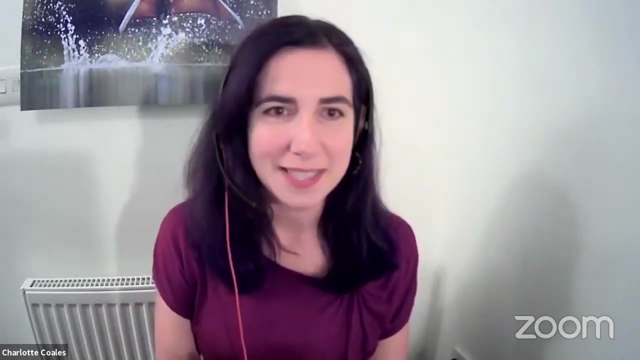 a result of this evening's event, and thank you all so much for your contributions. um, tonight it's been great to to hear from you and hear about some of the case studies and examples you shared as well. um, and a big thanks. thanks as well to ellie darby, who's been working behind the scenes. and is the producer of the film, and i'm going to hand it over to ellie darby, who's been working behind the scenes and is the producer of the film, and i'm going to hand it over to ellie darby, who's been working. 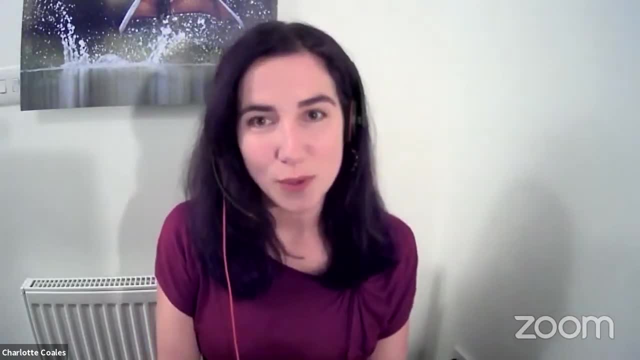 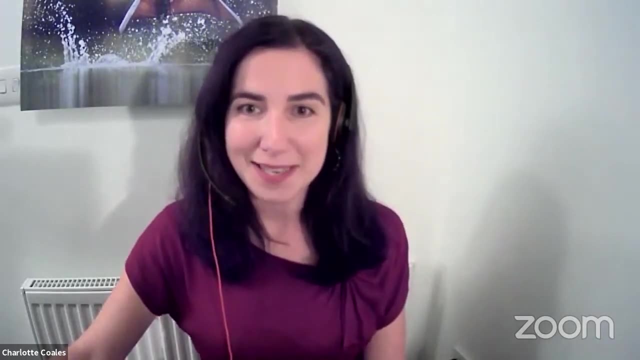 tonight's event. thank you, of course, to all of you who have been watching this evening and sending in your questions as well. i'm sorry we didn't have time to answer more of them. as i mentioned at the beginning of the event, we are really keen to get your feedback, um, and try and improve these.